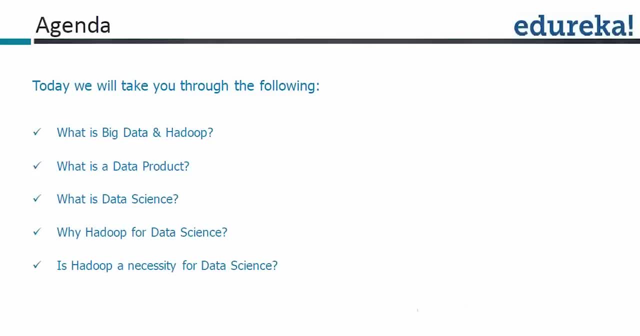 science, and you know we'll also. you know I'll tell you a small problem towards the end. you know a simple problem. you know how we can see that in Hadoop. right, that is something I'm going to. if time is, time permits, I'll try to show you. 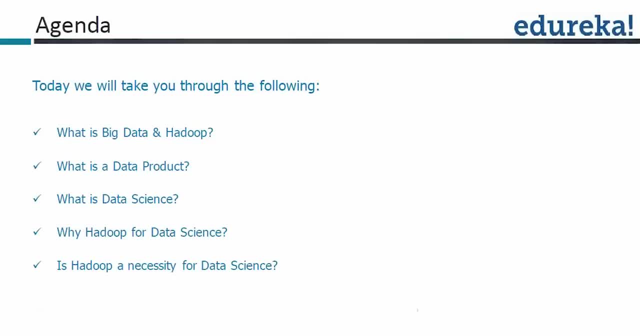 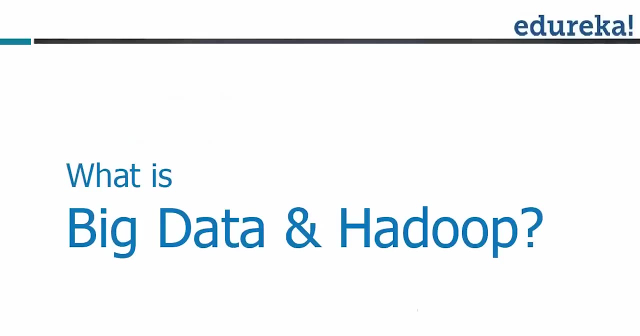 that as well, right? so here is our agenda for today. and, moving on, what is big data and Hadoop? right, let's try to demystify these terms, right? so I think, if you, some of you may may have noticed, right, people with you know, people who have, I think, many of you, 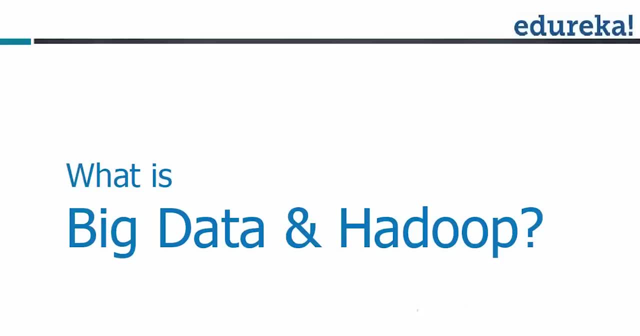 must have at least look through the internet, Google and various social media sites and YouTube and all that. there are scores of videos available pertaining to big data and Hadoop and there are lots and lots of things you know, related topics in internet and all that. so it's all. 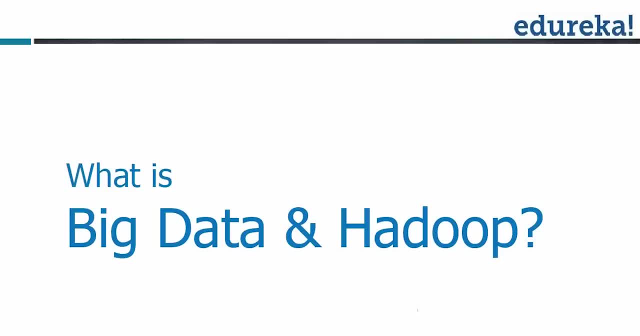 available in different, you know manifestations, I would say, but you know, is there enough clarity still there? you know that that's, that's a question, you know, which requires to be answered right: what is big data and what is a Hadoop? so can you, you know, can some of you just take a quick guess, and you know, 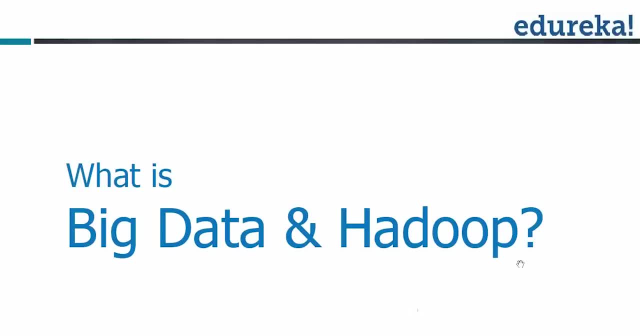 type it out in your question window. what do you think is big data? right? I just want to keep it little more interactive here. what is big data, friends? anything that is big, anything that is large, anything that is scalable. what's your- you know- view about big data? and what is Hadoop, you know? just give me one answer. 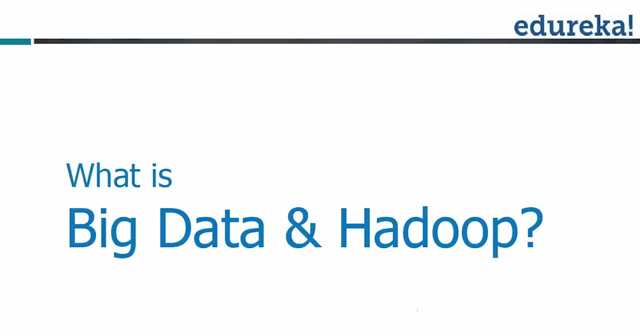 right, just one word answer: data within data or from your experience. we just want to give you one minute. you know something interesting and you know what is big data. is the big data things? just specifically about big data. so, Hadoop, why do you think is big data and what is? 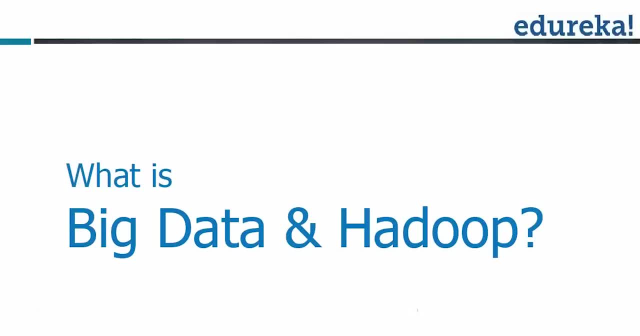 Hadoop, what is it? and we'll get into that later. so from there's a big data we have. Is the paid data? okay, Shrek on says that. anybody else just take a guess? okay, awesome, a lot of people, Svea. I'm just reading the ones we know, which are: 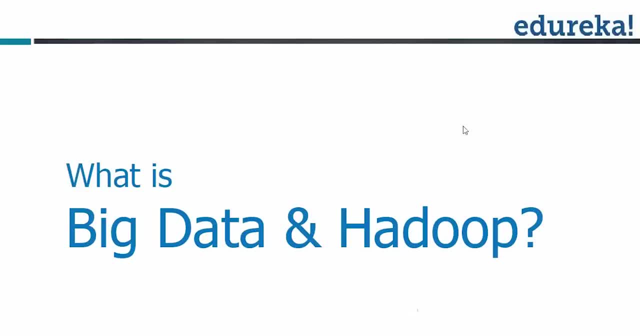 coming closer framework to analyze huge data volume. huge volume, velocity, variety managing high volume, not samples, entire thing. huge data, huge amount of data manipulation, large amount of data which can't be processed with regular database- awesome, I think. I mean I'm very happy to you know, get a lot of. 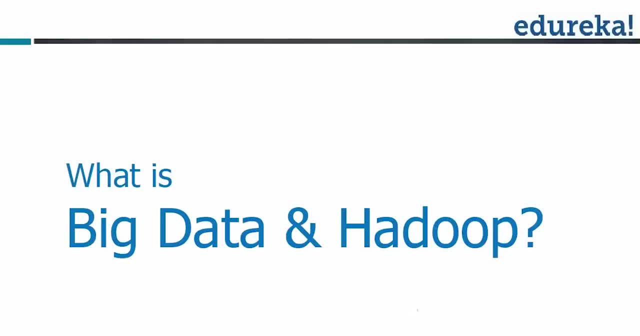 great answers from all of you. I think you guys are not starters for sure, right you? I think a lot of you have unstructured data, beautiful right data in terms of zettabytes and, yeah, brilliant guys, Hadoop is a framework to handle our shadow. yeah, thanks, thanks, all so, friends, if someone asks you tomorrow what is big, 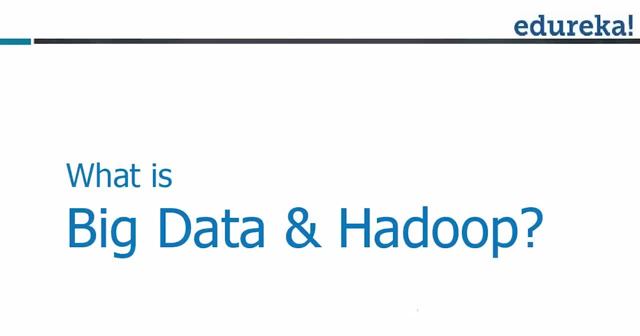 data. what is Hadoop? you should know the answer. so anything that can be you know the data is that is big, right? so, if you can, you know something which is of high volume, coming from different varieties and which is coming at a alarmingly high velocity, right, so that is going to be a big data. not only that, many of you. 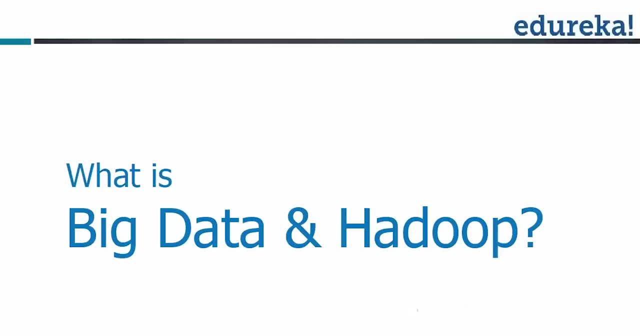 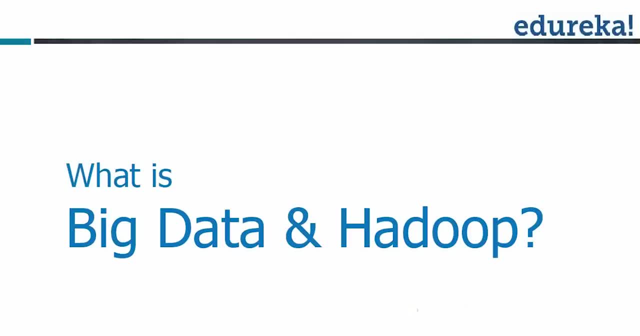 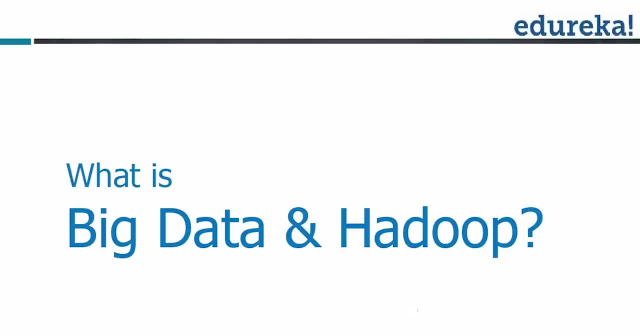 it's like doing something in, or could I think that point. you know, Facebook was probably not there. awkward was, you know, one of the sought-after things someone was doing that. you know, Yozai, people will look at that person like an outcast. you know, maybe he's- he's not a. you know he's not very aligned with the job, or. 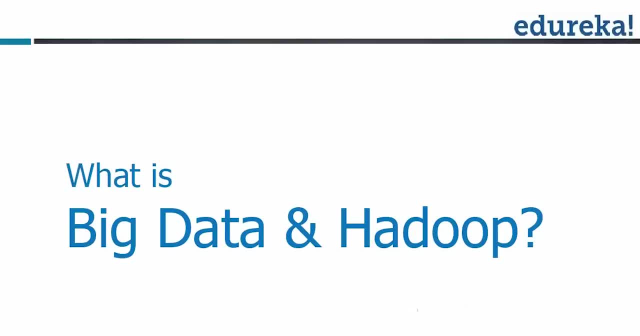 is just, you know, he's just like a wayüll増 X kind of image, right, that's just all digital art, right? so today, social media, however, 80-, do not tend to pick up over the top a ton things showing in your top half, you will notice, you know, if the information of it was copiedョ. 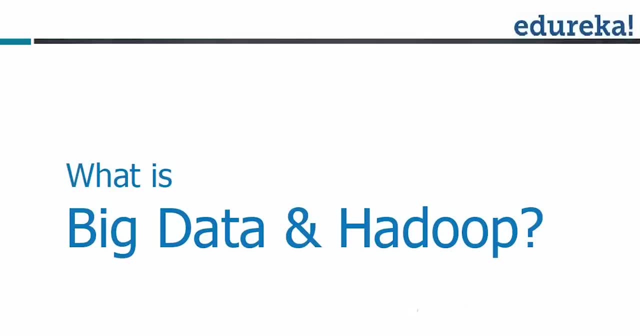 media cannot be ignored, right, so we do sentiment analysis, right. so a lot of major decisions are based on sentiment analysis. what we do in Twitter, right, and we look at you know a lot of product insights come out of this. lot of things keep coming right. so major product decisions are made based on the 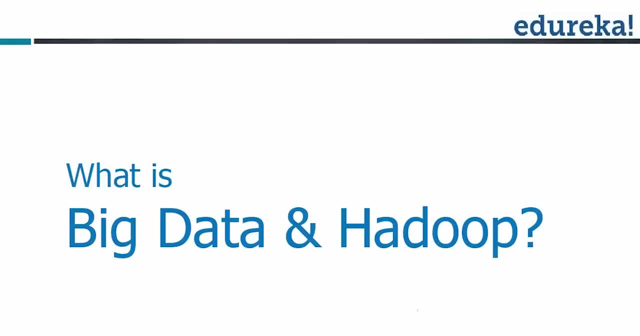 decisions, you know, based on the insights, what we derive out of this social media and various kind of you know channels. so we cannot just ignore this. so times have changed, that's what I'm trying to say. so huge data, unstructured data, everything is big data. Hadoop is a framework to handle this big data. yeah. 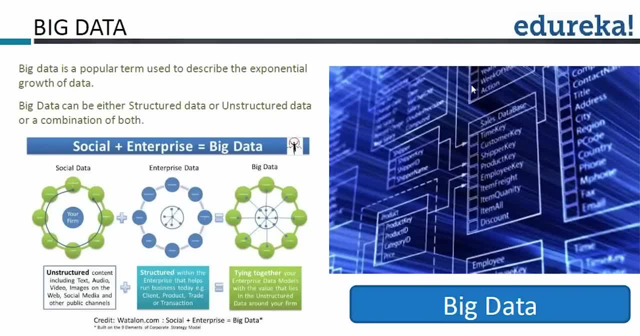 so, coming to this, you know, look at this exponential growth of data, fine, social enterprise data, right, it's just a culmination of everything big data put to be there. so big data can be either structured data or completely unstructured, right. so unstructured is something you know, something like your text data, your 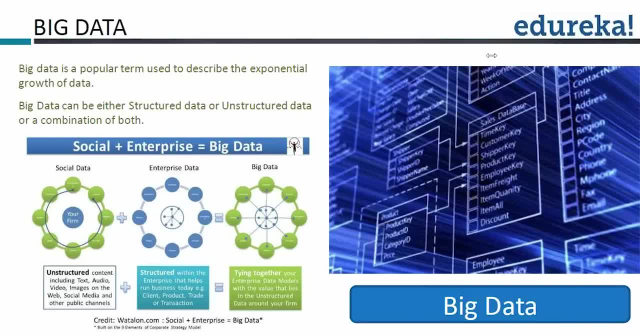 audio video. you know something that cannot be structured right. all these are unstructured data and these kind of unstructured data is becoming more and more. you know we are getting more and more of such types. compared to better at 1983, 됩니다 data right? all these unstructured data we have tracking. 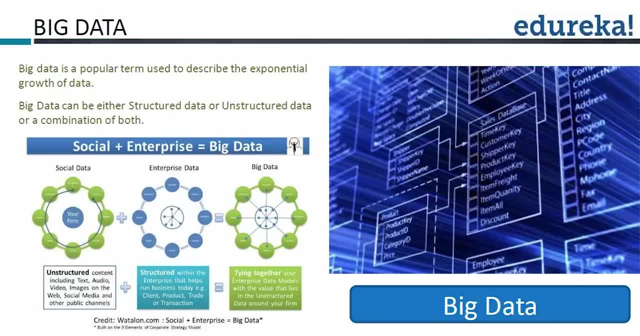 data and droite, micro and right. so this is really right and right, that can be data. so that's the story about big data today. right, so we cannot. and and the traditional systems, whatever we have been having, overall those systems are just not able to scale up right? that's one of the reasons why we are looking at 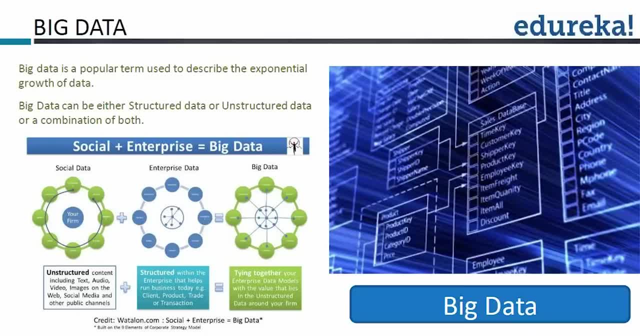 you know big data a lot of people are. you know they just want to jump into this bandwagon because they don't have a choice now, right, so most of the enterprises, or you know, earlier they were dipping the toe. now the curiosity is: you know even more? you know it has gone up and we really want to get on. 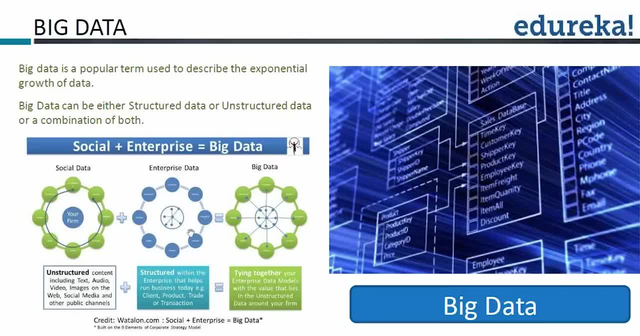 with big data right. can someone tell me, like okay, one is the social media they cannot ignore, and all that? can someone tell me what could be the factors for companies, corporates, enterprises, to show the sudden, you know- shift? you know it's like a tectonic shift. I would say that. 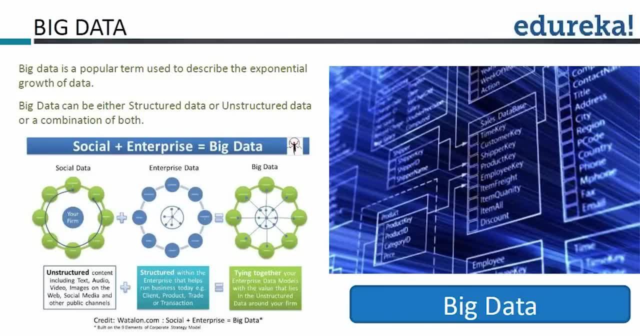 why is there a tectonic shift of the mindset of these corporates, companies to jump into the big data? you know we cannot say that big data was, you know, just came like yesterday. right, it has been there for the last few years, right? probably four or five years, right? so why is the sudden rush? can someone tell me? 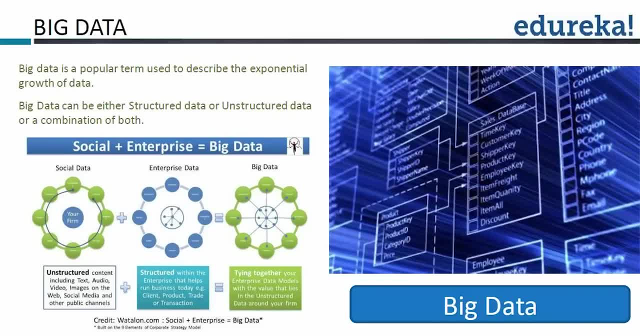 no, like just can someone guess? awesome, great answers: better business: handle all types of data, predict what that will be interested in buying- excellent, yeah. unstructured maintain- okay. cost-effective genome- okay, I like this answer right. cost-effective mining the data- right. so, friends, data analytics- nearly 90% unstructured data- yeah, all these are where all of you are telling. 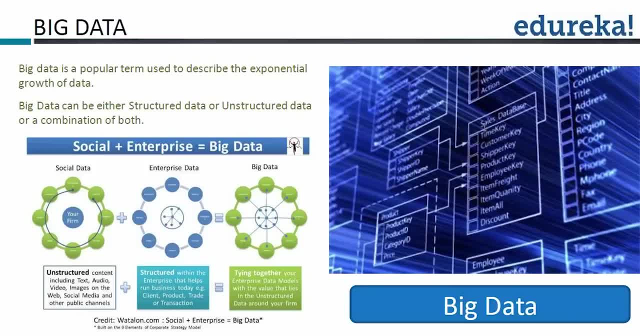 very, very valid points. one couple of things you know which really makes it more interesting for the customers is, oneness, for us to process this kind of data right. the other amount of data can you all, you know, if you for us to buy even a? you know a RAM, a 640 KB. you know 640 MB RAM. you know, those days I am. 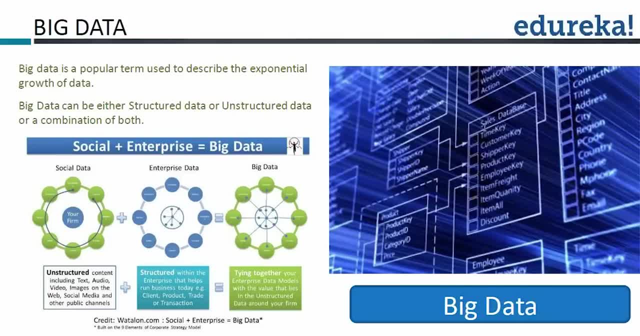 talking about. you know it was seriously expensive. you know it was seriously expensive. you know it was seriously expensive. you know I'm talking about 90s, mid 90s and all that. so those were the days, you know. and today, the mobile phone, what we are, you know, just for 20 grand, right, you get a. 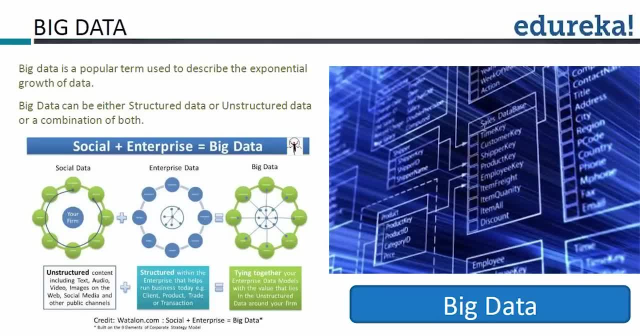 fantastic mobile phone with octa-core. you know it's phenomenal speed right, the and it has really, you know it. I would say that most of the tablets, what we hold today, they are faster than many of the laptops available. right, they are really faster and you know, most of the work gets. 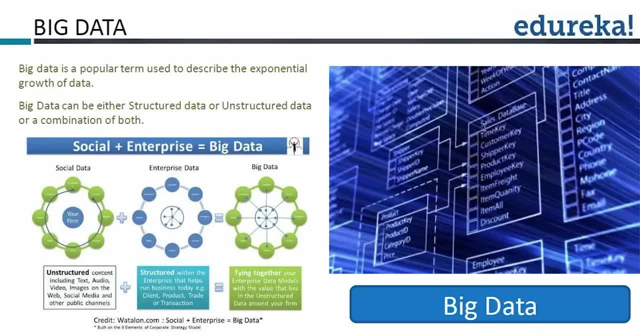 done through tablets itself, right? so it's: things have changed, times are changed. you know we are just moving ahead and you know we are in a very fast-paced environment. things have changed and it's going to be constantly changing, right. so that is, let's not forget that right. so what is powerful? 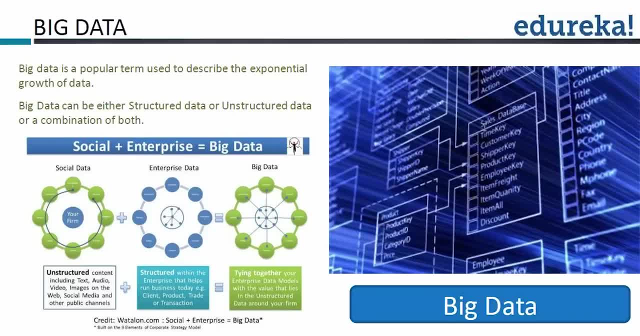 today may not be powerful tomorrow, right, so big data itself will be a moving target. right, it's going to be a moving target. and the other thing is the cost to process the data. right. these kind of things are going to be changing, right, so the hardware cost has really plummeted, right. one is the cost of processing, right. 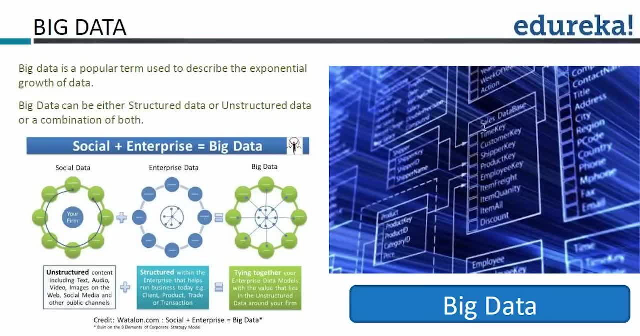 the hardware. those things are really come down right. so the company is: you know they don't have the apprehension to try out this because you know they cannot. also, the most important point is you know they just cannot ignore this big data any longer, right? so most of you have pointed out that you know it is. 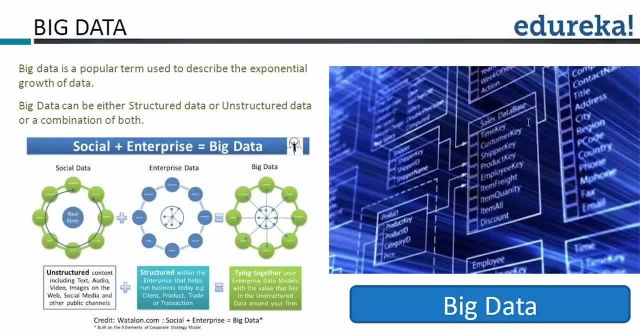 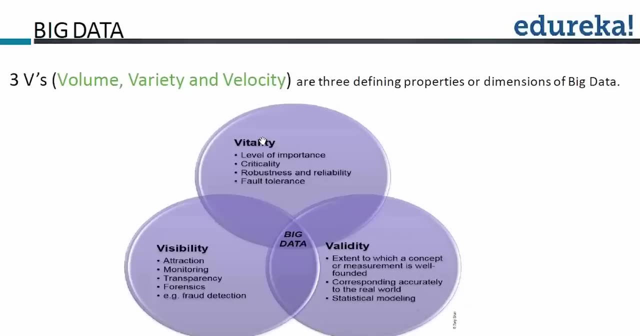 good for predicting the you know pattern, buyers pattern and whatever business they are on right. So it's critical for organization to keep in pace with a fast changing world. giant has pointed out great point, Yeah, So yeah, these are all valid points. friends, Look at this three V's and if you look at you know IBM, I think they have, they've got. they've added one more week called veracity, which is the your quality of the data itself, right? 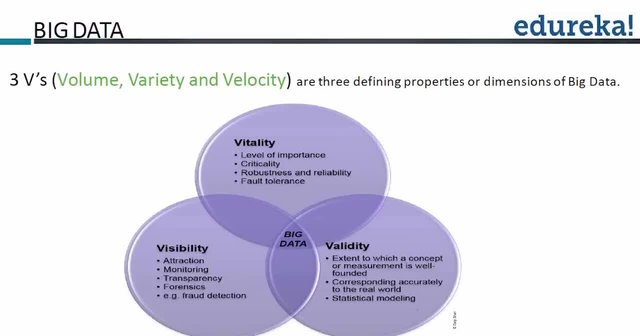 So, uh, volume, variety and velocity is there. Look at this vitality level of importance, how critical it is, how robust it is, fault tolerant, monitoring, transparency, forensics, fraud detection, for visibility. A big data is like you know it, just it's like a central theme for all this bubbles: validity, corresponding accurately to the real world, statistical modeling everywhere, right. 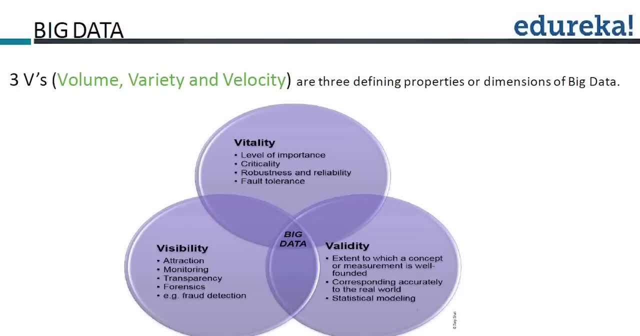 The data is growing. data is big, right, So big data, even though I can say that you know it is going to be a moving target but it's going to stay for quite some time. now, right, Because all this data science, even our- uh, you know, our- experiment with IOT, right, Everything you know- has got to do a lot with the data, right? 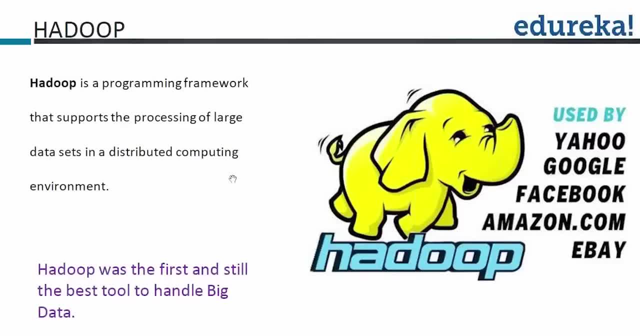 Just a minute. So Hadoop is a programming framework. You see this, this adorable yellow elephant- Large process, large data sets in a distributed computing environment. So look at this. I, I really like this, this part. Hadoop was the first, still the best tool to handle big data. Friends, let's not forget one thing Today, I think if you, if you have seen, uh, Hadoop, then we people are talking about Spark. 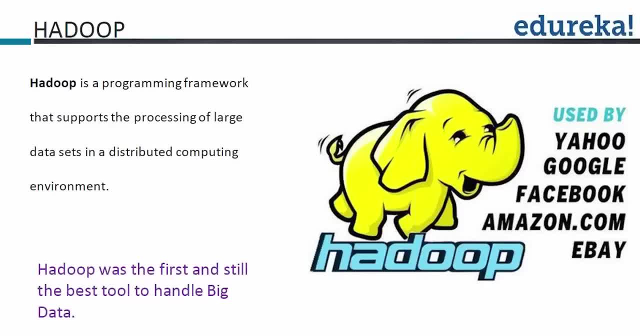 People are talking about Storm. People are talking about Flink. There are several flavors. There are a lot of projects, you know, that are in. you know some are still in the research stage. Some have come out and some are. you know they will become a efficient project, uh, a little later. There are lots and lots of flavors of you know, Apache. uh, you know open source. Those things are coming out. But you know, if someone learns Hadoop, Hadoop still has a lot of flavors. 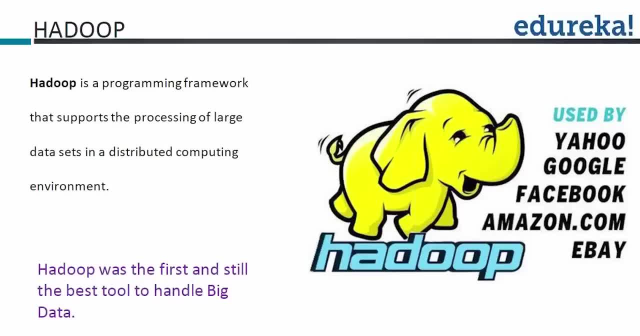 So Hadoop still remains the favorite, you know, to handle large amount of data, Because there are a lot of fancier options, like you know, in-memory computing. People say different things, But Hadoop is the fundamental thing, right. It still remains one of the widely used frameworks to handle big data. 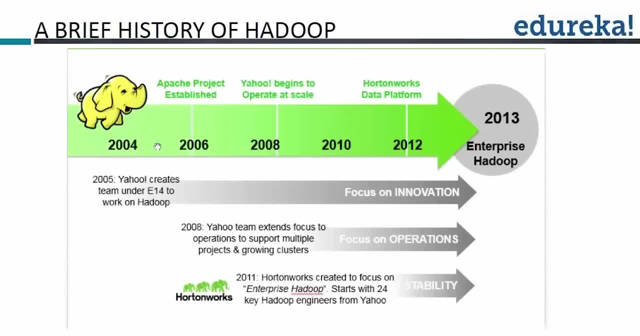 Brief history of Hadoop. Look at this. Uh, it was established. Yahoo creates team under E5. It was established in 2014 to work on Hadoop. It became a project Operate at scale- Hortonworks data platform. I think some of you must have experienced this. Hortonworks has. you know they have this sandbox and everything you know. Uh, you know that's that's also gaining popularity today. So Cloudera, Yeah, Yes, Shrikanth, Thanks. So Cloudera is there. In fact, a lot of people you know offer Hadoop platform right. 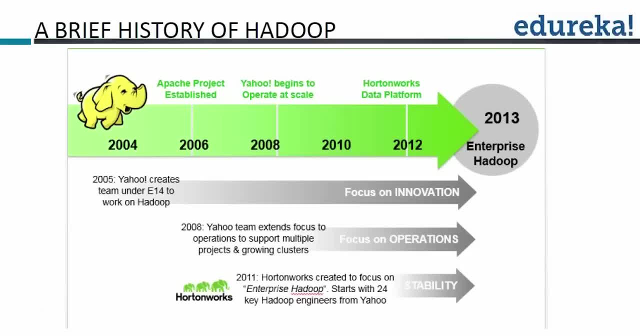 Hadoop remains an open-source, because you know Hadoop remains popular, It is open-source. Secondly, it is very, very successful. I mean it's cost-effective, It is scalable, It's horizontally scalable, It is flexible. okay, Provides scale on economy. You can just go on, you know, you can go on adding this. 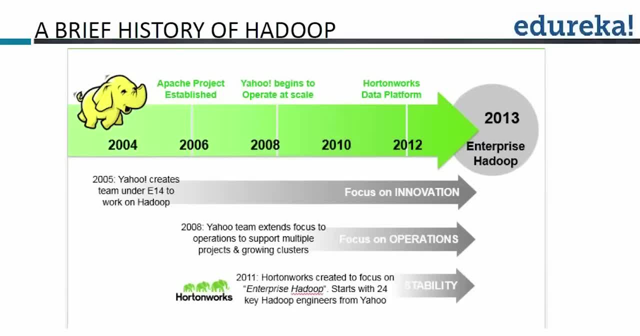 Balakrishna is asking: Is Hadoop a technology or a framework? it it's. It's a technology framework. I would say it's more a framework application to handle big data right, Because Hadoop has It's a frame. It's a framework which has got two vital ingredients. 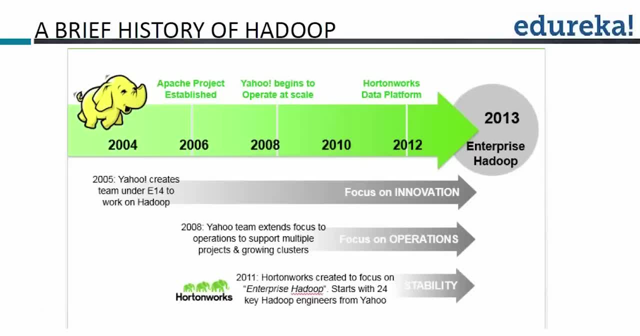 Called Hadoop file system, and the map reduce for processing the data, right, So I'll come to that. I'll come to that. I'll come to that. It's So. it also provides stability and all that stuff, right? Hadoop, so Hadoop. 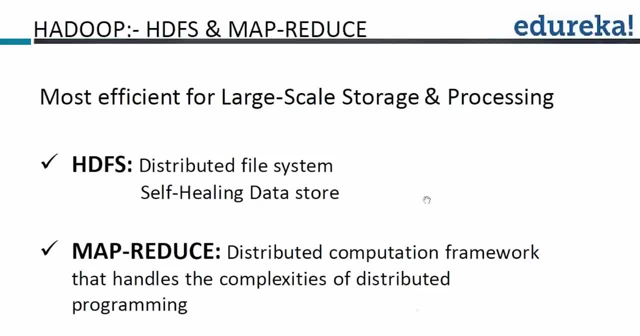 Look at this: What is horizontal scalability? Sure, Yeah, Shrikant has asked this question. I'll answer this. then I'll answer the mudras question: any language processing tools? I'll come to that. Yeah, so let me answer. What is horizontal scalability? So, friends, 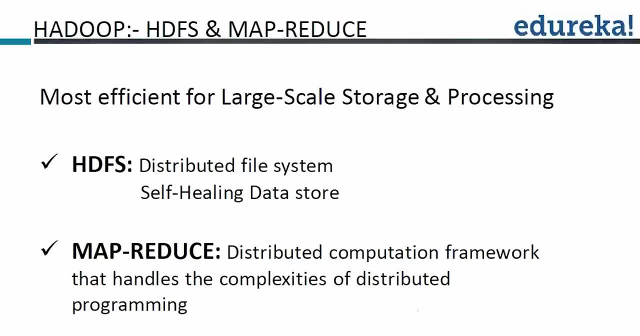 What I try to say is like, let's say, you have a machine, right, you have a mission, We just got about two gigabytes of RAM, right, I have operating room of RAM for, shall we say, 100 gigabytes of data, and You process a. 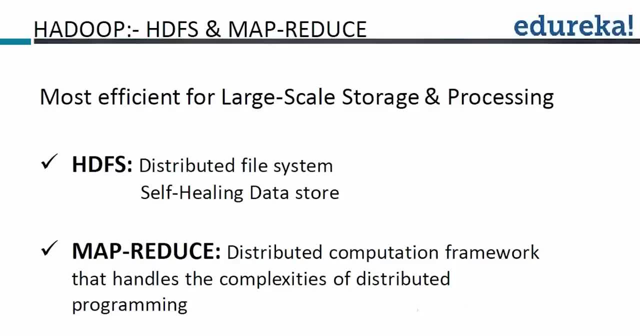 Hundred gigabytes of data, right? So let's say it becomes very slow because of the disc io switch, disc io. you know It keeps switching the io for the RAM to load the data, things like that, Right over a period of time. it becomes very slow, crippled, what you realize. 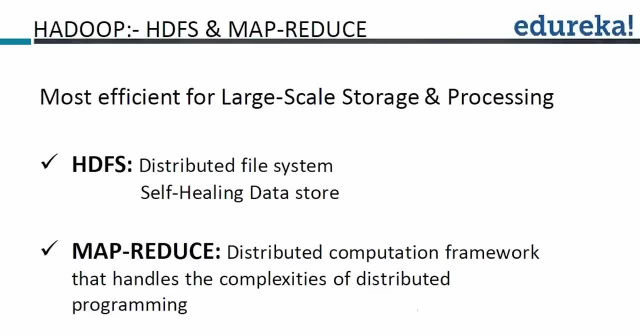 Hey, it cannot process these kind of data, this volume of data. You try to juggle around. you upgrade the ramp, you try to make the ramp to, let's say, gigabytes. it becomes faster. right tomorrow you bring on another file which is probably half a terabyte. what's going to happen? the same problem will come in. 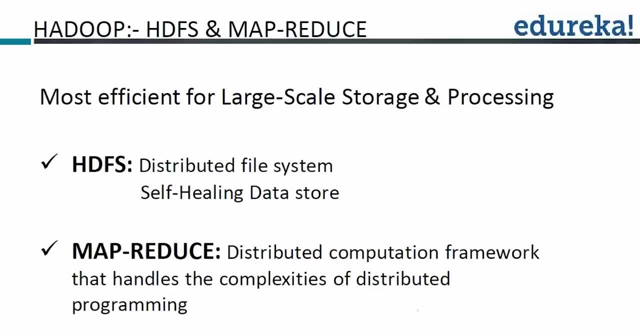 right, because it's not able to. you know, the RAM is not good enough to sustain or to handle a file which is a much larger size. right, it gets crippled. so what we do? we keep go on upgrading how far you can upgrade. you tell me that right it's. 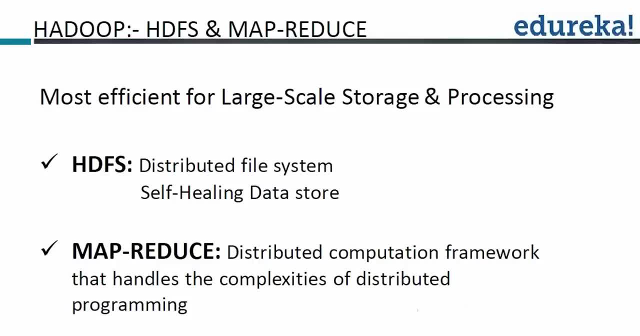 you will be restricted. I mean, you cannot go on upgrading this. so the other option is: you handle, you know, you probably have a system you know, which is probably of, let's say, four gigabytes of RAM. right, if this system is not able to handle a large file, you add another five systems. right, these are commodity hardwares. 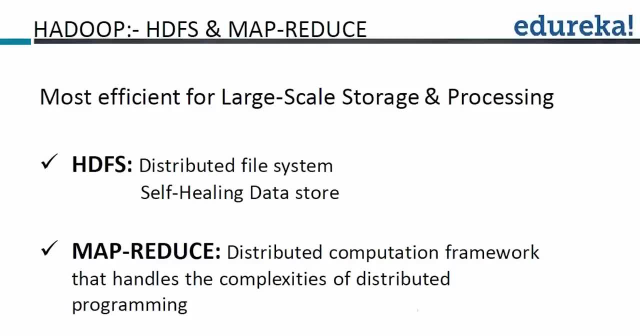 right, so you're they're not going to be super expensive. you just go on adding it right, so it the way it is going to be handled is. you have a system which is not going to be super expensive. you just go on adding it right, so it the way it is going to be. 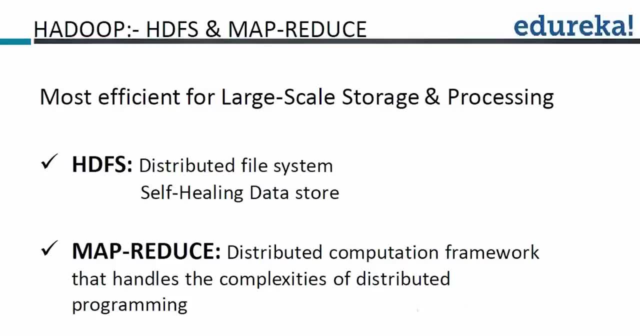 handled is. you know, it is growing horizontally, right, not vertically. you're not going to, you know, go on bubbling up. once particular machine right. you rather add more terminals which are far more cheaper and which is going to perform distributed computing versus computing on a single machine. 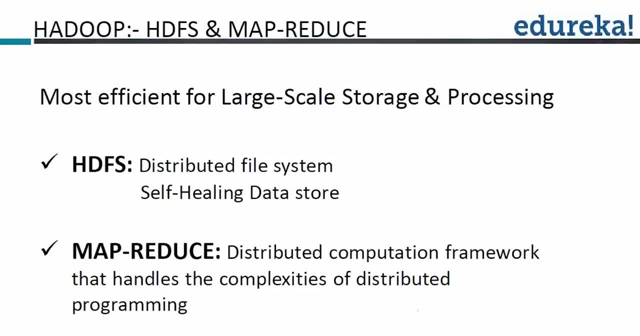 single powerful machine. this way the amount is, the workload is distributed, so it becomes far more efficient. am I answering your question, Shrikant? are you clear now? okay, so is it related, any of language processing friends? Hadoop itself was written in Java, just for your information. so, but Hadoop doesn't mean 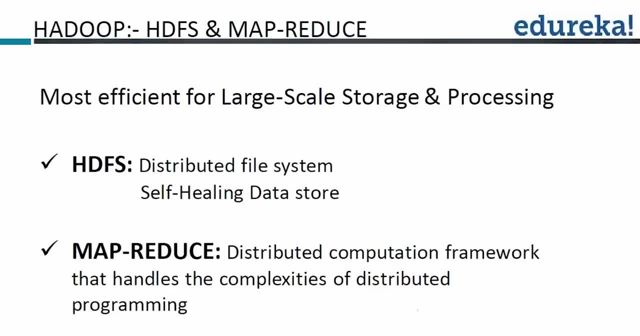 that you know Hadoop has got lot of ecosystem tools. it doesn't mean that you know you need to understand more of. you know Java or anything map reduce. of course you need you know. if you have Java expertise it's good, but you know it doesn't. you know there are a lot of other languages like you. 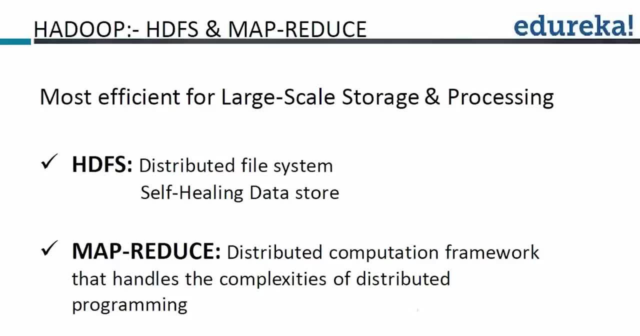 know, pig is there, hive is there? right, so you can use these languages as well. right, which are completely you know, which abstracts the complexity of map, reduce Java, and all that right. it makes it far more simpler so that you focus on the problems versus getting stuck on Java related issues, and all that right. 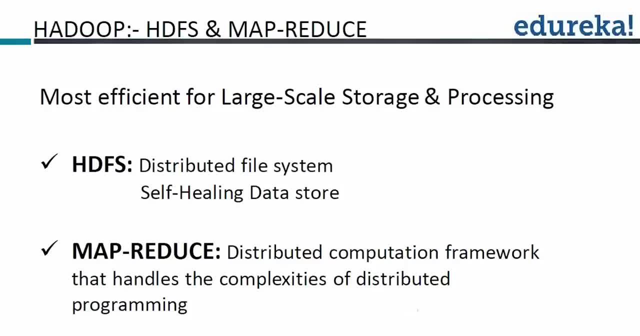 so that's the intent here. so do we still use map reduce or yarn? okay, Bryn Mawr? okay, I think it is up to us. yarn is more like a platform friend, so it's more a platform and you know, Hadoop 2 uses yarn, right it. 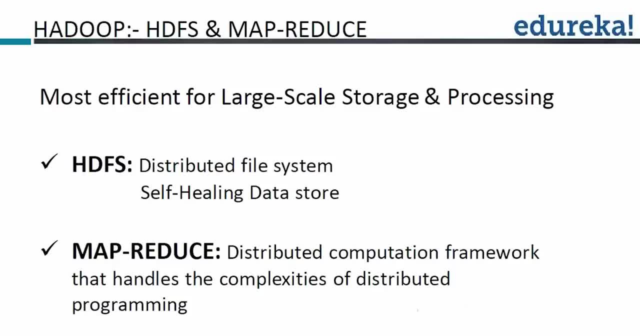 provides yarn, and MapReduce runs on top of yarn, right? so there are other frameworks that can also run on top of yarn. that's how it is, so we can use MapReduce on top of yarn. that is what we are talking about- and we can use these. 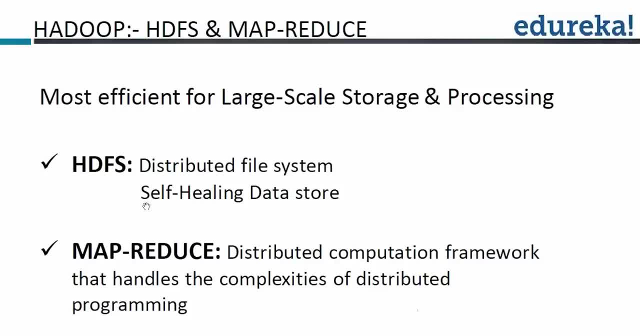 what I want to say. so look at this distributed file system, self-healing data store. yeah, map reduce. so what we have done very intelligently today, but you know, with Hadoop, is these two are combined right. one is the storage, another one is the processing- right, these two are coupled fine in in if you. 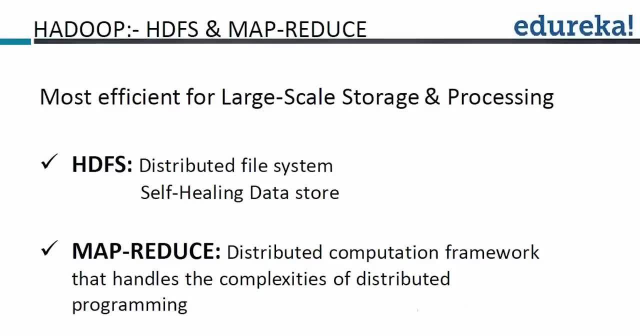 just rewind your memory how it was handled, you know, in a traditional system, right? so we always take the data that is stored in the storage area to the processing front, right? so when we take it to the processing or compute layer- let's put it that way, right- storage layer to compute layer when you take it. 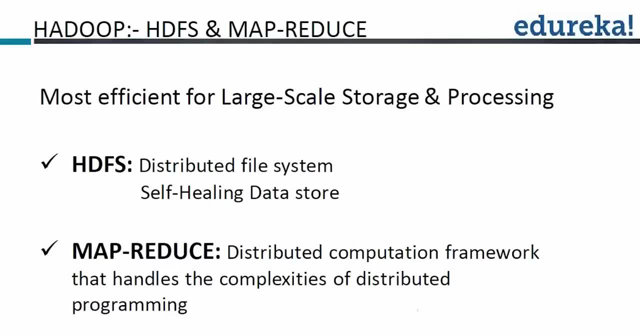 what happens when you take it itself. it can triple the network if the volume, data volume- is pretty high, right, so what we want to do is we? we have merged these two things together in Hadoop, so one of the fundamental shift, I would say. how to compare to the? 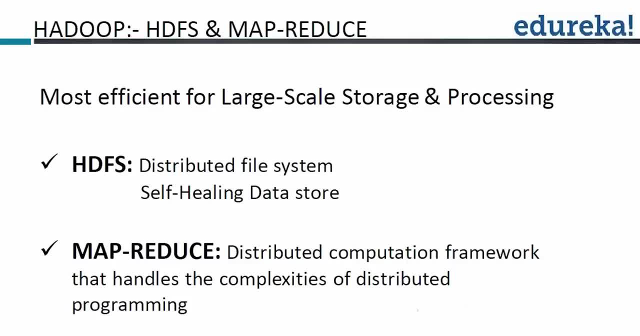 traditional system. why it is faster is the processing is taken to the data, right, versus the data is taken to the processing in the good old days. right, the data is taken to the processing, like you are shifting the data where it needs, and all that today, the processing program or whatever that is taken to the 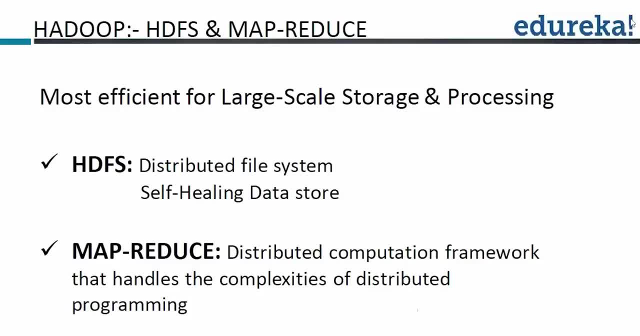 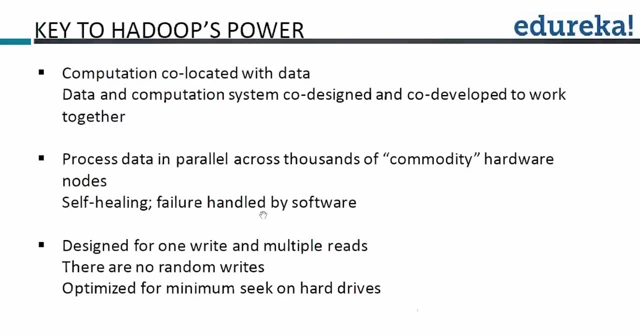 place where the data resides. look at the, look at the shift, so the data doesn't need to be moving along the network, right? so we have made this super effective by this way. let's move on from here. computation co-located with the data, right? so that's very, very critical. 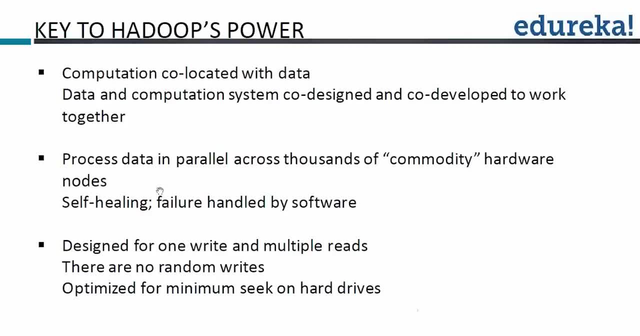 here, co-designed, co-developed to work together. process another thing: process data in parallel. thousands of commodity, hardware, nodes, failure handled by software, which is self-healing. so when we say parallel processing, friends, what we mean by this is, you know, for us, because data is stored as chunks or 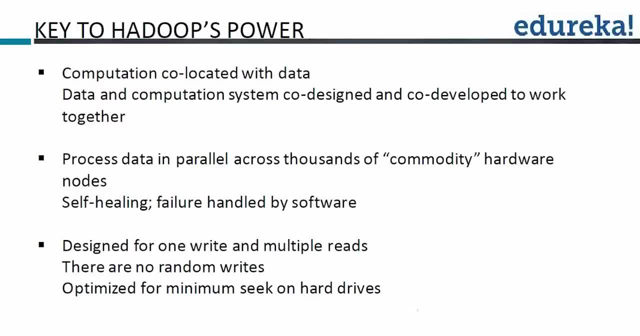 blocks in Hadoop cluster. so what we have. let's say we have a file that is stored in Hadoop cluster. so what we have. let's say we have a file that is stored in Hadoop cluster. so what we have. let's say we have a file. 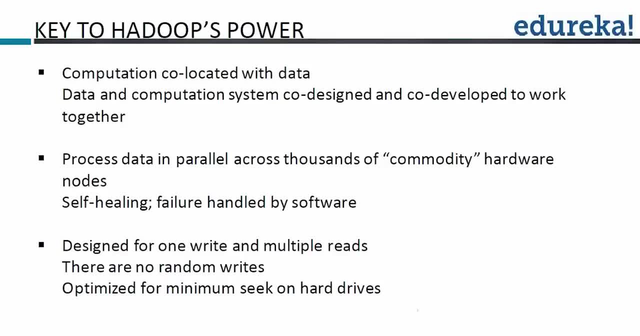 which is of size 200 megabytes. so if the default block size- what we set in a Hadoop cluster- is 128 megabytes, how many blocks we will be storing in the cluster? two blocks, right. one is 128, another one is probably 72 bytes megabytes, right. so 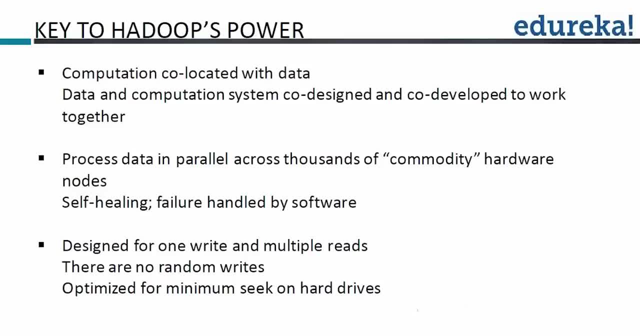 when we process these files. right, how we want to process, you know it will be processed like: imagine a file which is running two terabytes. it will be processed as individual blocks and commodity servers and multiple servers will be processing this blocks in parallel. so which is a parallel processing, processing which makes it 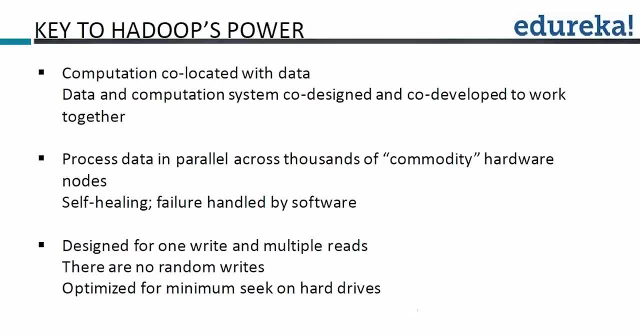 very, very efficient and pretty fast compared to, you know, the traditional systems. however powerful they were, they still cannot handle a very large volume of data. designed for one right and multiple reads. there are no random rights. right optimized for minimum seek on hard drives right. what when we say: 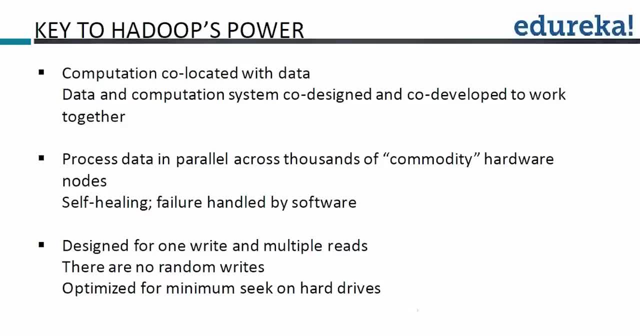 minimum seek, see. the other one thing is Hadoop has caught very high latency in the sense, see, it is not suitable for a OLTP kind of processing. suppose you want to get into a bank and look for. okay, mr Rajasekaran has come into. 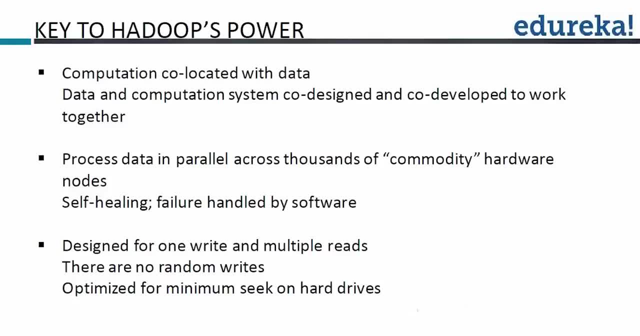 verify his account. you know, if they look at his passport they want to pull all the Rajasekaran's details. what they do? they just go by the you know account number, account name, something like that. right, they will have a primary key and all that. they are quickly able to get the data. Hadoop is not designed for that. 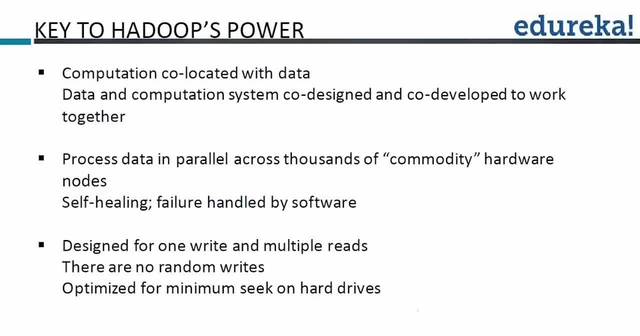 Hadoop is more analytical in nature. it has got very high latency, meaning you cannot go and zero in on a particular row of data quickly. that is not possible. you can't go and zero in on a particular row of data quickly. that is not possible. you can't go and zero in on a particular row of data quickly. that is not possible. 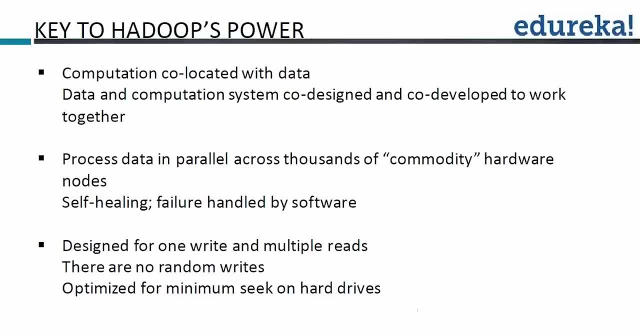 okay, RDBMS can do that for you very quickly because it is indexed, it has got primary key, foreign key and all that, whereas Hadoop has been designed to read data, which is a very high volume of data, right, if you want to read 20 terabytes. 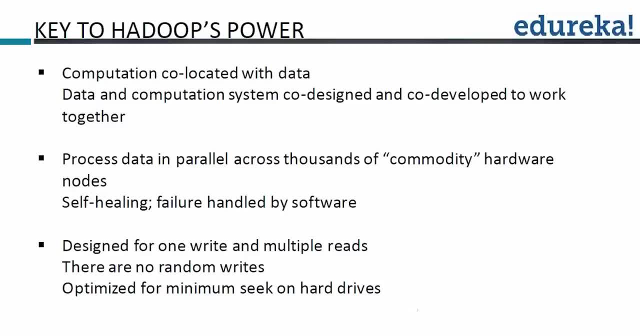 RDBMS will take a day or two and still may fail. Hadoop can do it in minutes for you, right? so it has been designed for such kind of purpose. friends, are you all clear so far? am I going in the right pace, all right, thank you. thank, thanks for the confirmation. yes, blocks, okay, shake on. 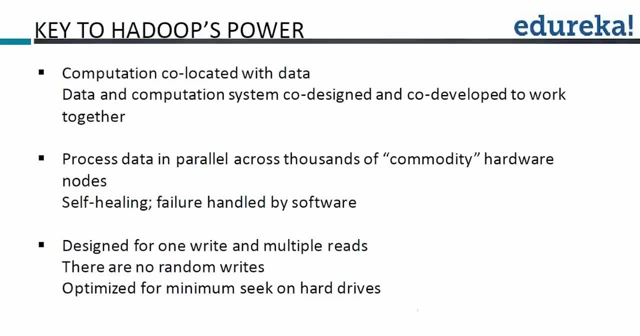 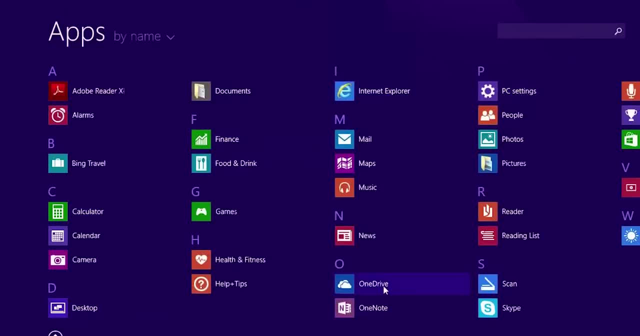 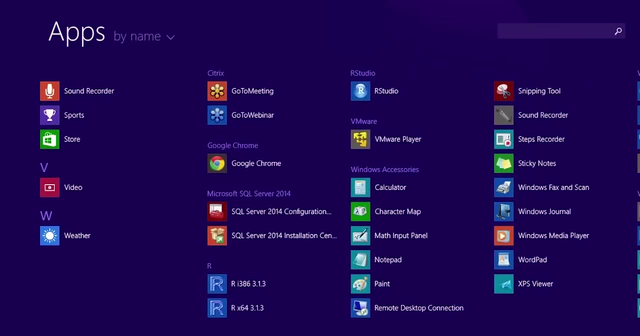 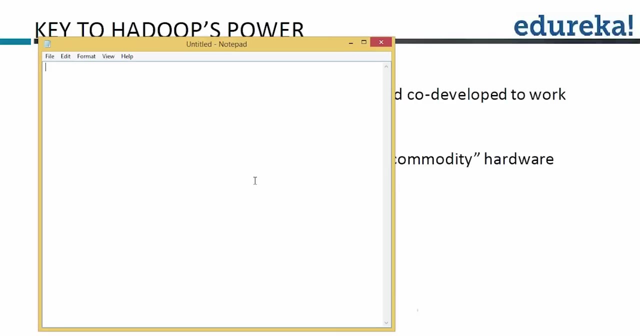 this asking: what are blocks? nothing, shake on. see, let's say: you know, you know, just give me a minute, I'll just show you. I like my. I mean I like to use like a quick whiteboard. okay, I'll take a notepad. see, what I try to say is, let's say, a file which is called test dot tat, right 200. 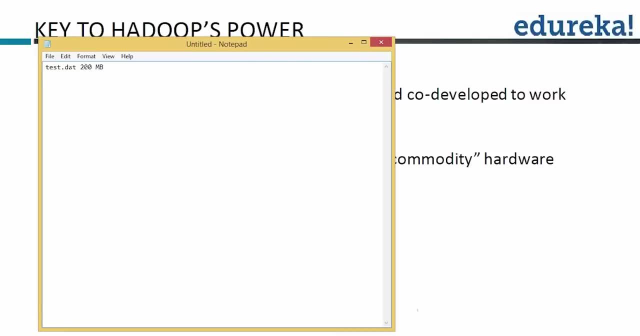 megabytes is the size of the file and block size. block size is one twenty eight megabytes. this is a default right, so I love b1 block 1: p2 right. so this is 128 megabytes. this one is 72 megabytes. fine, this is how it. 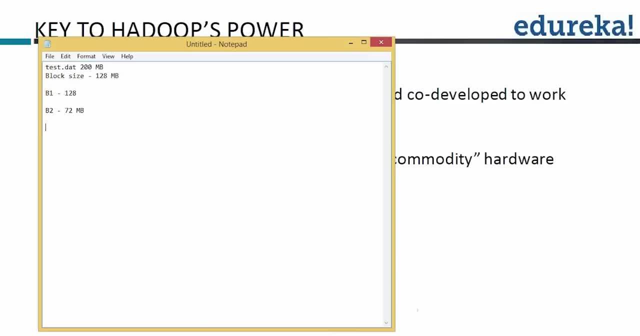 is stored. so these are blocks, basically blocks. so the tester that has been fragmented into two different blocks, so b 1 in block 1 in block 1, so the block 1. these are b2. so the test dot tat has been fragmented into two different blocks, so b. 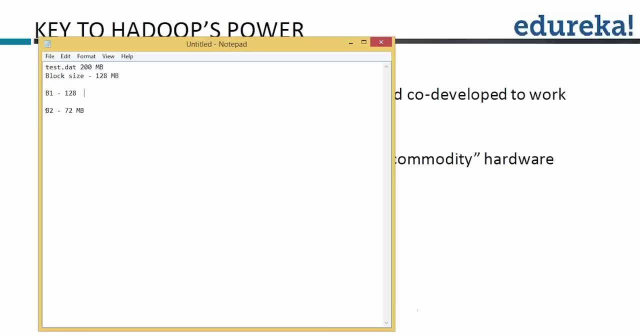 one could be stored in server one. i'm just taking, you know, i'm just taking a. giving you a very simple example. okay, p2 should be server two. okay, so someone, balakrishna, says default block size is 64 mb. okay, sure, balakrishna. see, uh, friends, just want to tell you in hadoop one, the default block. 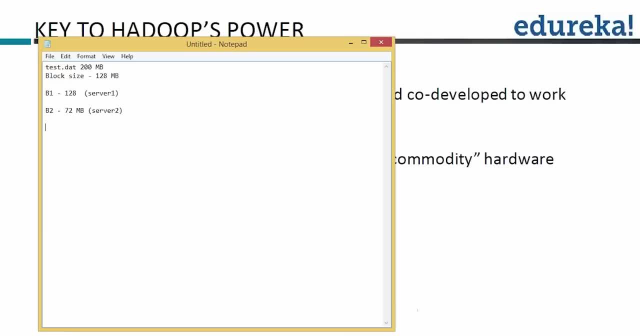 size is 64 mb. in hadoop 2 the default block size is 128 mb. fine, of course, this block size, it is not a sacrosanct field, it is configurable. so in another way i can say: you can go to hadoop 1 and 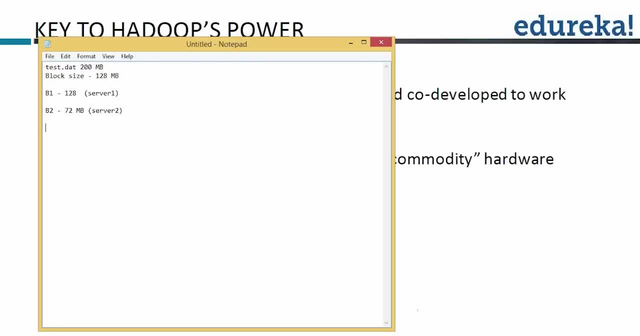 make the default block size to 64 or to 128 and to hadoop 2, you can go and set the default block size to 64. you can do anything, or you can even make it 300 as your default block size. so this is. 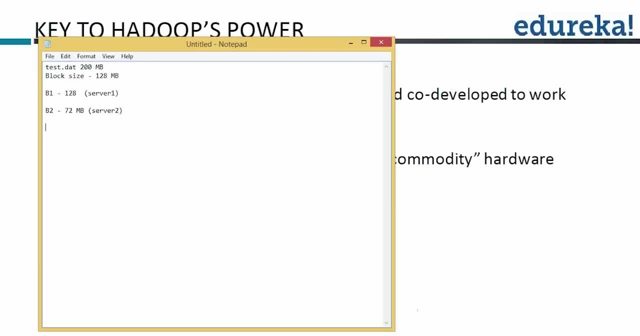 a configurable parameter, but by default, how do? Hadoop one is 64, Hadoop two is 128 megabytes. So that is something you need to understand, this. Thanks, Balakrishnan. thanks for raising that question. Blocks or server? no, no, Shrikant, blocks are data. 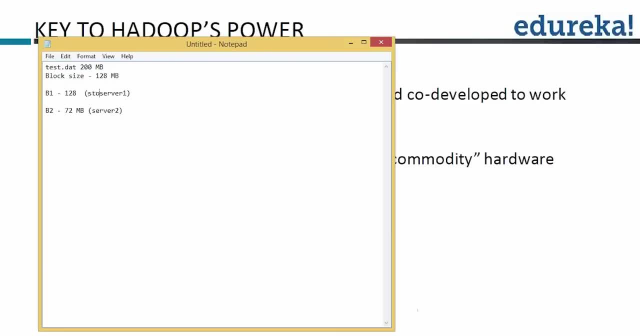 They are basically data blocks stored in server. You got it Stored in server, one stored in. they are physical data, but it has been distributed that way. It's like a chunks of data. right, You're just pulling part of the data. 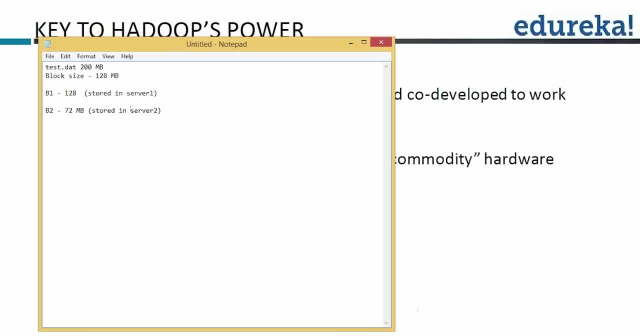 and skipping it in server one, pulling part of the data, keeping it in server two. So by pulling this, we are able to process. when we process, we do parallel processing. You got it Divided into blocks. exactly, Exactly, Shrikant. 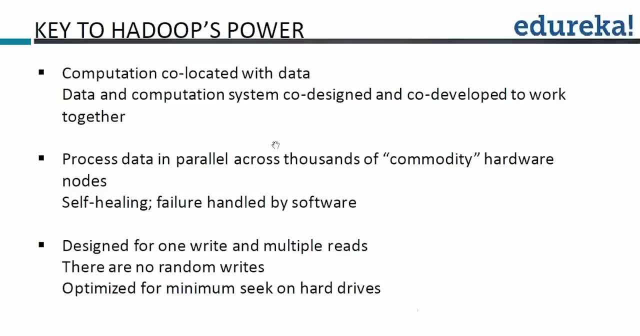 They are divided into: yeah, thanks, So that is key power of Hadoop. someone asked one is the data locality. data locality, which is nothing, but they are co-located with the data Computation co-located. one thing. 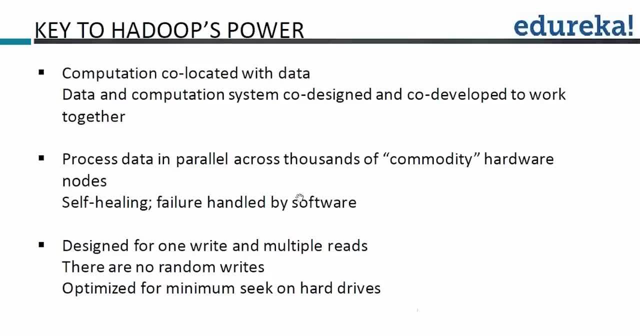 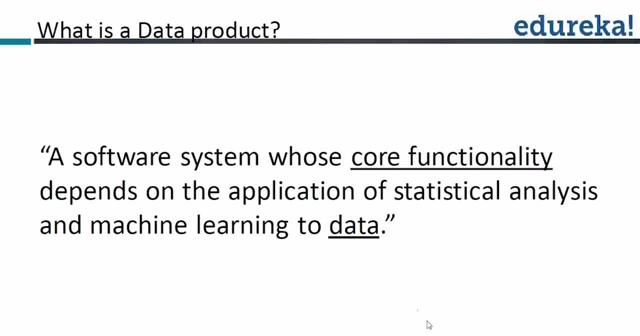 And again processing data in parallel. These two are very, very vital. You need to understand this Data product software system, whose core functionality depends on the application of statistical analysis and machine learning to data. So this is a data product. So that is also it is used for. 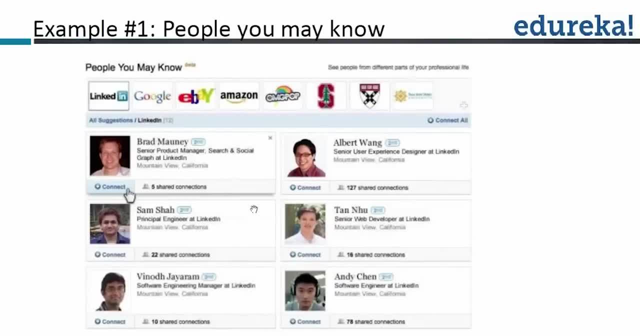 So look at this. You know people you may know. I think what is this? Does it ring a bell to all of you? What is this? basically, It's a LinkedIn right: People you may know and all So can someone tell me friends? 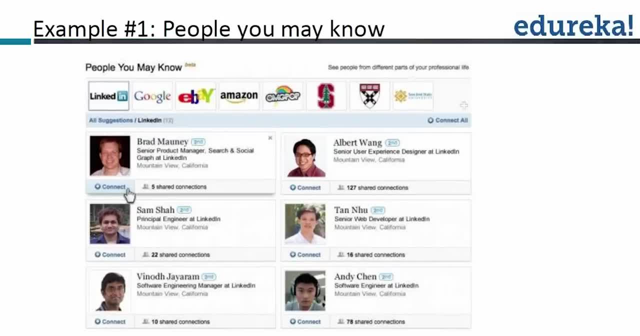 what could be the logic here? People you may know What is this basically? Any guesses here? Associations, matching skills, all are correct. Brilliant Manish is saying: recommendation engine. yeah, That's exactly the word I was looking for, brilliant. 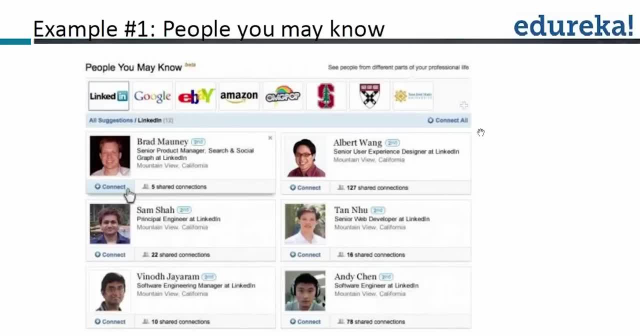 So yeah, other answers are also correct. but you know, this is the, you know this is the concept here: recommendation engine Friends, any idea? See, just want to give you a small picture about that. There are about. 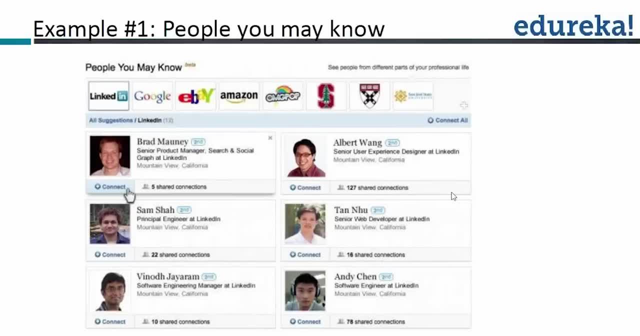 300,000 active members in LinkedIn, right, Like you know, the figure could have gone up by now. okay, But now see, the point is, if you need to go and connect with people, right, You need to go and connect with that many number of people. 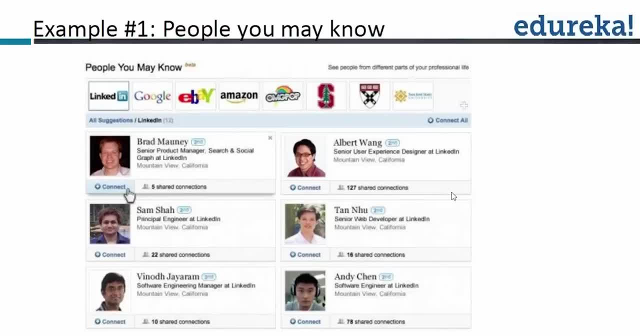 I think you'll probably drop, drop LinkedIn and, you know, go to some other site, right? People will lose patience, right? It's just not going to work. What they have smartly done, I think some of you, I think some of you have pointed out right. 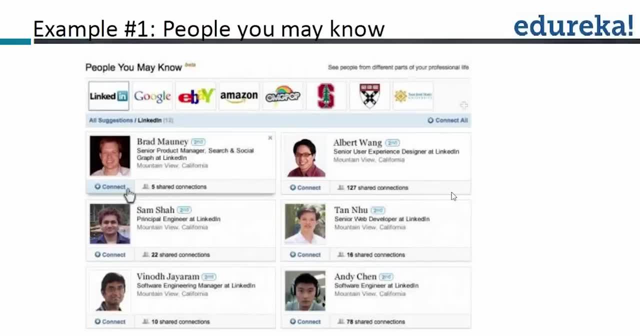 Commonality. they look at commonality and you know, pick up some of the common attributes, patterns, right, And they try to link you up whether you have worked in a, you have worked in the same company, okay, Same profession, same designation, you know. 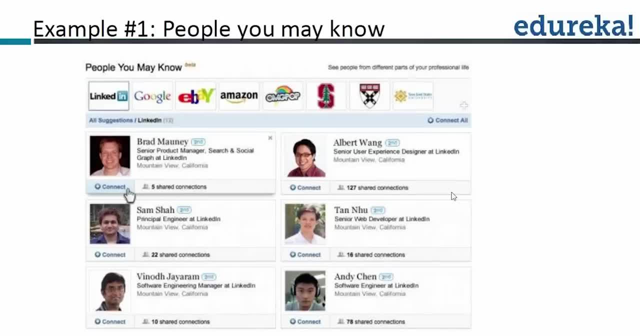 something like that same technology. They try to do all this smart matching right Associations. they do all these things okay. Then they prompt and it so happens, you know, I would say at least you know 16,000,, you know 60,000,. 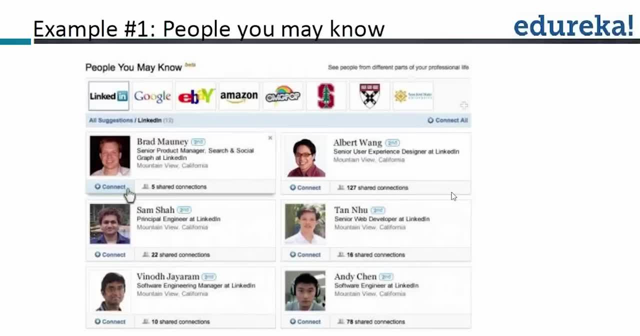 more than 60%. you know, you will. you know. it should be like a familiar face to you, right? Or I would say that you know 60%, you will go for it. You will go for it and you know. 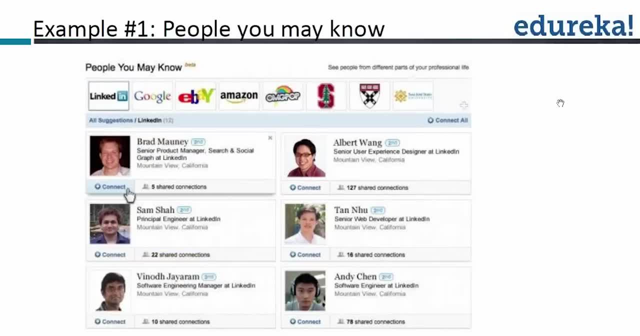 think that you know this is working right Versus the other. you know this is something, you know it's more successful and you know that is something you cannot ignore right. So they've done their job. 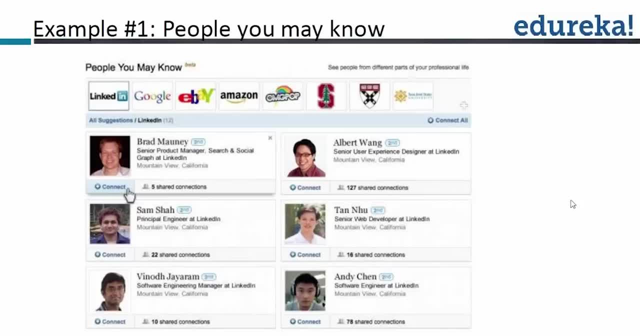 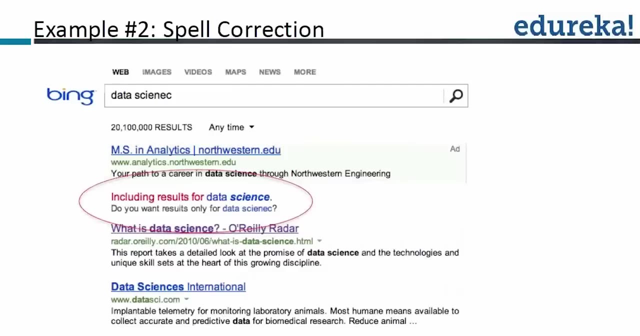 That's what I'm trying to say. Do you all agree with me, friends, On this part? the recommendation engine of LinkedIn. Okay, thank you. Spell correction: yeah, Again, see, do you want results for this right? 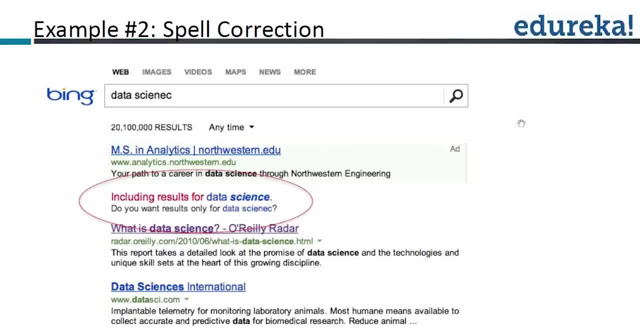 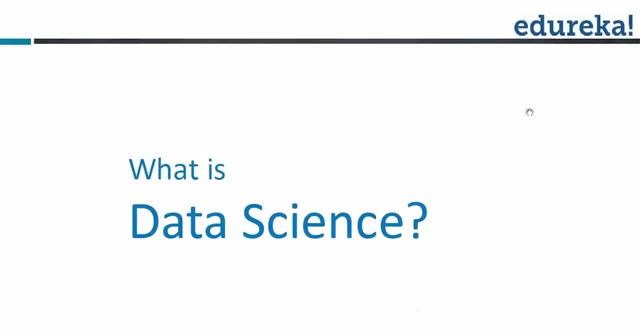 So they do this as well. What it relates to Hadoop Sikand, I'm coming there, I'm coming there, I'm coming to that part. What is data science? I think yeah, Sikand. So your question will be answered pretty shortly. 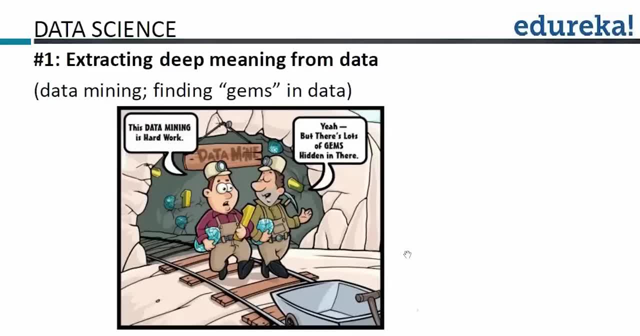 So what is data science right? So extracting deep meaning from data Data mining, finding gems in data Data mining is hard work, but there's a lot of gems hidden in there. How many people think that data means a lot right? 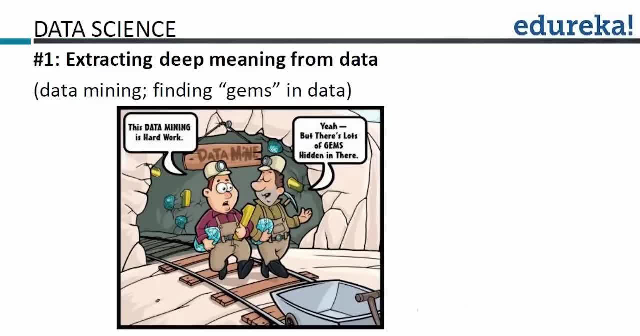 They also say: you know. one of the trendy statement people make is: you know the recent, you know. they also say the black, the you know. lot of people say that you know the data. if it is analyzed, you will find gems okay. 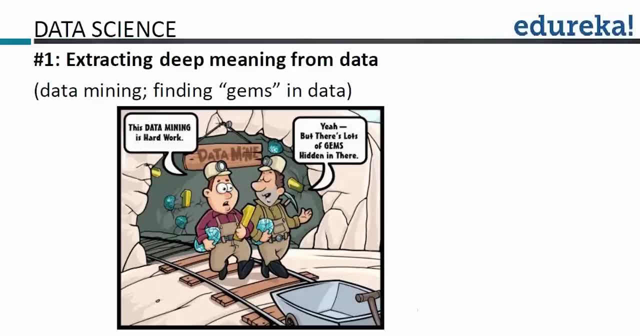 If it is properly analyzed. If you don't properly analyze the data, you'll find nothing. It's as good as like a dead data: dumb data right. It means nothing. So the data analysis right. That's a pretty vital thing, okay. 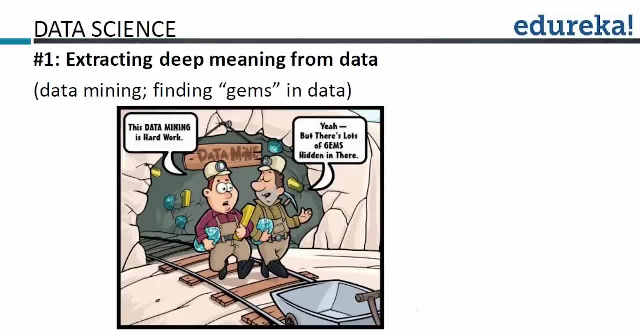 So let's talk about data analysis versus data science Little bit. I just want to give you my perspective here. See data analysis. it is, you know, somebody from a strong business domain, right? Let's say that you know you are given insurance data. 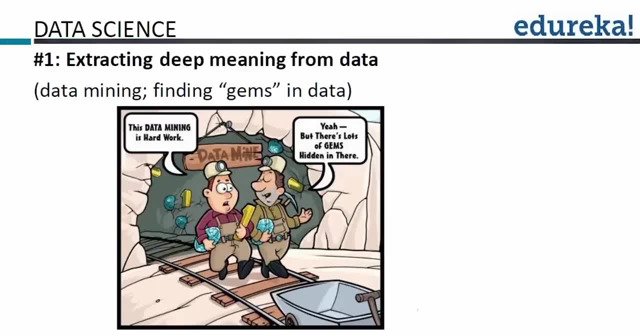 right? Do you think a non-insurance person, somebody from a different domain- let's say you know you're from a financial domain, right? Will you be able to make sense of insurance domain data? Yes, no, Okay. 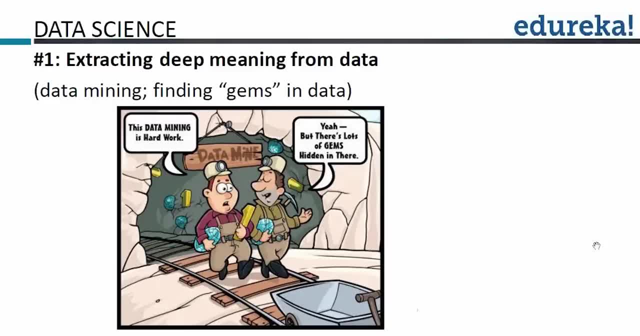 Some of it. okay, No, no, no, In fact. okay, Sajid, I think you're. I mean, I'll go with you. Some of it could be relevant. yeah, you're right, But yeah, somebody from the, let's say, retail domain, yeah, 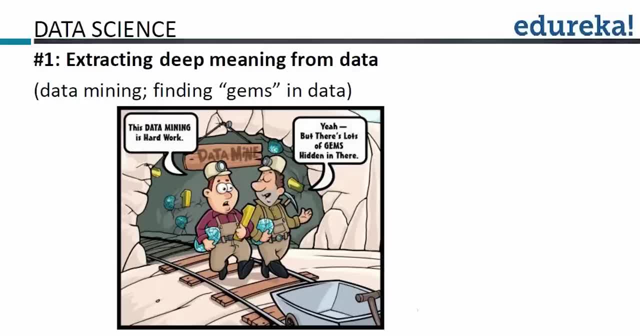 With insurance. yeah, You'll not be able to connect much, right? So, because each domain it's a mighty ocean by itself, right, And it has got their own domain: experience, you know, expertise and all that. So somebody from retailing you know. 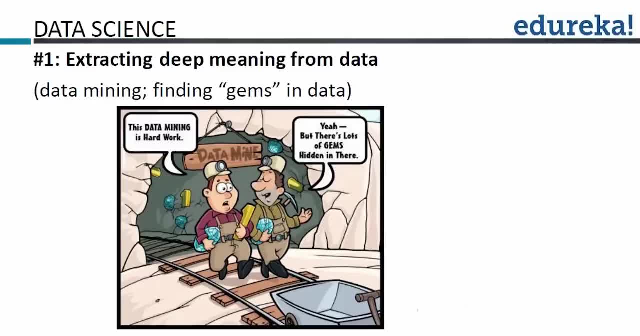 they will be very strong in that part, So they can do extensive analysis. They will know which algorithm to apply to get the best output or the best results and all that Right, Whereas if you give it to a financial person on a financial 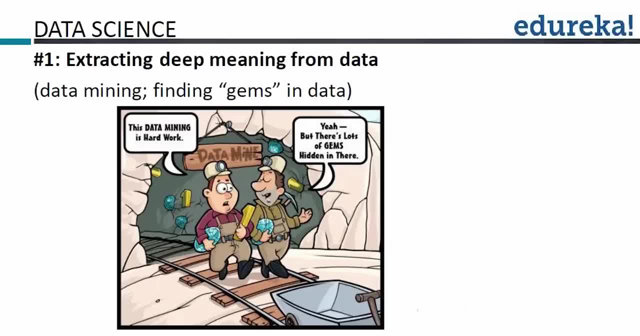 some financial data to a financial analyst. he can do an excellent job right. So it's very, very clear on that part. So that is more a you know. data analysis part, Data science: I just want to be you know. 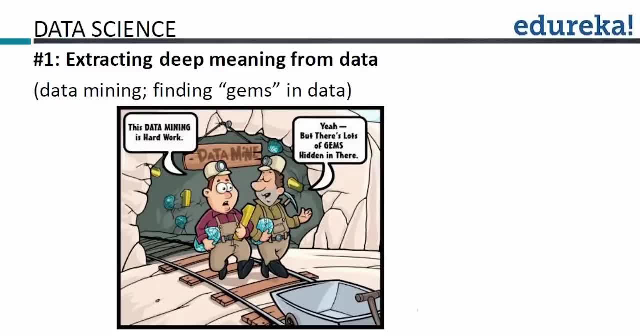 want you to have this difference very clear. Data science is more you know, it's more science than the analysis part, right? So an analyst will know which algorithm to apply for this business domain, Okay. Whereas a data scientist will know how to optimize the algorithm itself, right. 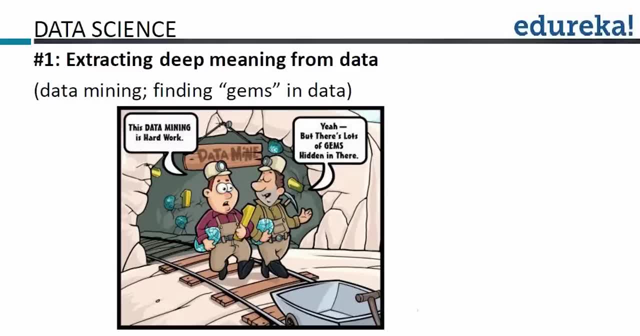 So it's more a scientific job, right? Since you know a data scientist will know, you know, should we use this clustering algorithm or should we use some other algorithm, right? Random forest algorithm. Okay, Should I take this linear regression? 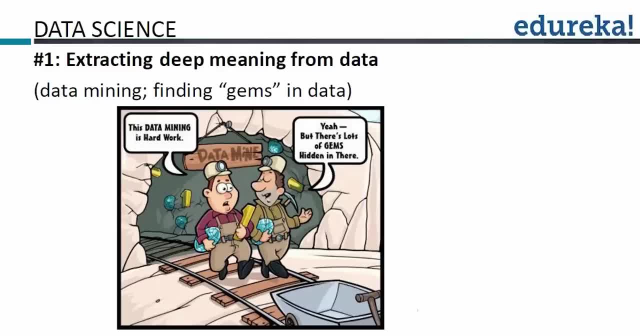 or logistic regression- right. So a data scientist will you know. take this linear regression or logistic regression- right. So a data scientist will know, not only know which kind of regression technique or which kind of logic which he has to do, he will also try to fix and optimize an algorithm. right. 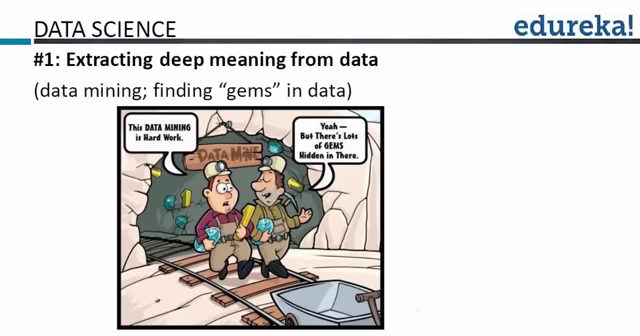 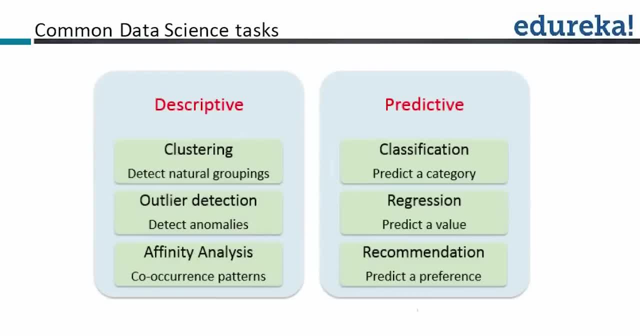 So you know that's more. a you know more. a scientific job is what I want to convey here. Now look at this descriptive and predictive right: Clustering. So you all must have heard about it. Clustering is nothing, but you know. 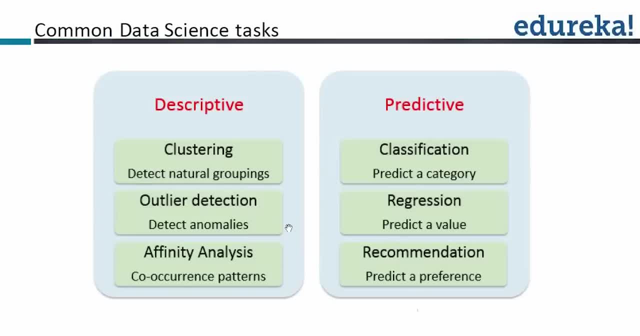 grouping or classifying the data. Data classification is nothing but clustering, Outlier detection. So you know outlier is, you know again, you know you're doing, you're taking a average of salary for a district right. 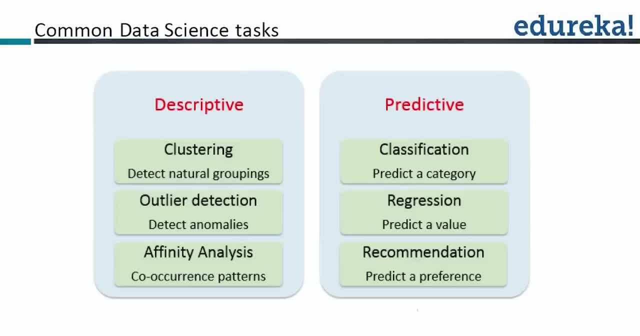 So let's say it is $1,000 per person on an average right And suddenly, when you are analyzing the data, one person is shown 50 million right. So it is an outlier right, It's a data anomaly, or, if you analyze it, 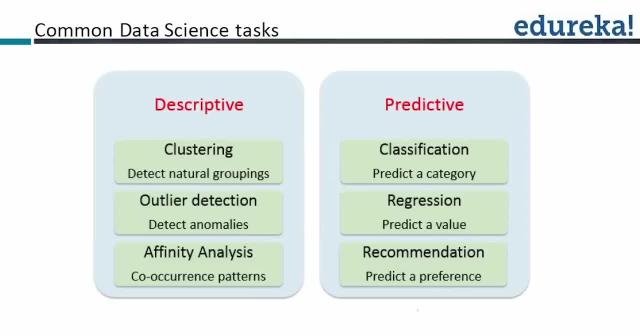 it could be like you know a high-profile sports person or you know a movie star. It's possible to So some analyst will be able to point out that Affinity analysis Look at the occurrence of co-occurrence of patterns. 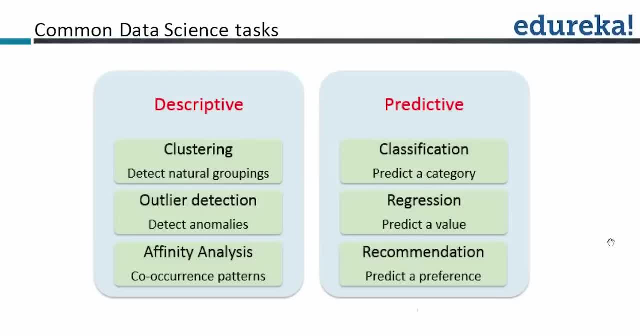 So that is possible, right? These are all the descriptive aspects. Classifications Predict the category. You know someone mentioned in the very beginning stage. you know they can do a. you know prediction Why they're using big data, right? 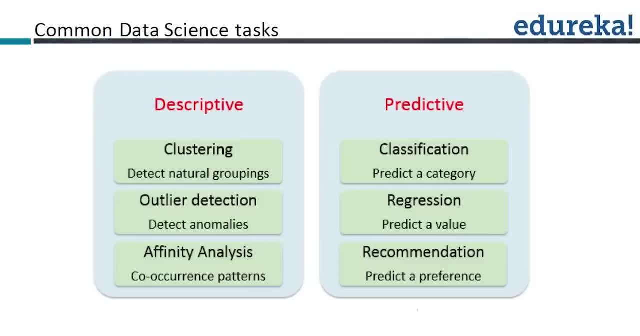 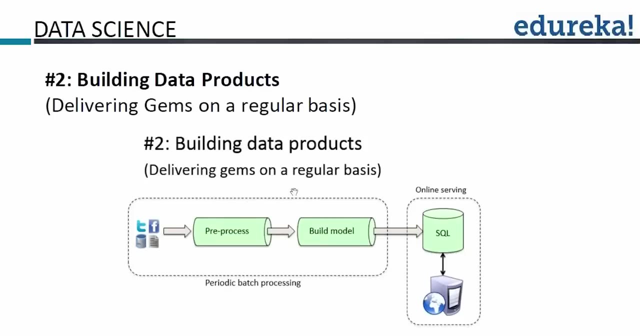 Predict the category. Regression Predicting the value: Yeah. Recommendation Predict the preference right. All these are possible in this data science world. Now look at this, Look at this: building data products right, Delivering gems on a regular basis. 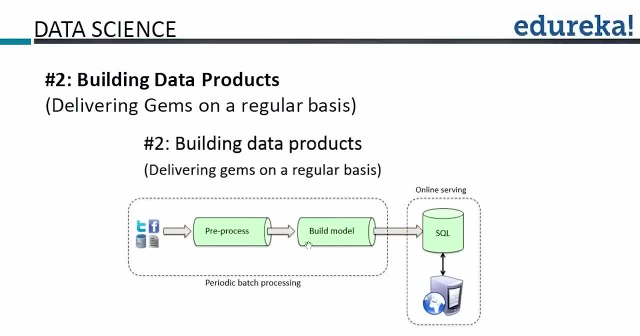 Look at this When the data goes through this processing tunnel. right, We are building a model and we are passing it to a data store, which is a persistent medium here. right? So we process the data and we send it to the data mart. 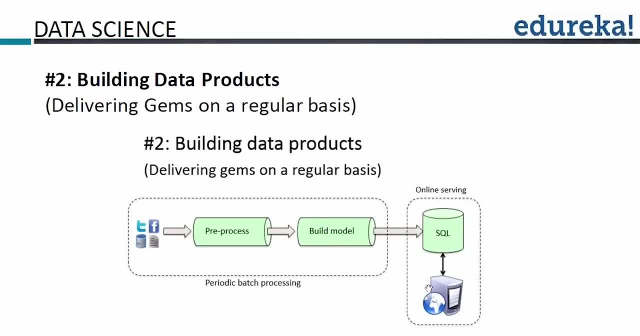 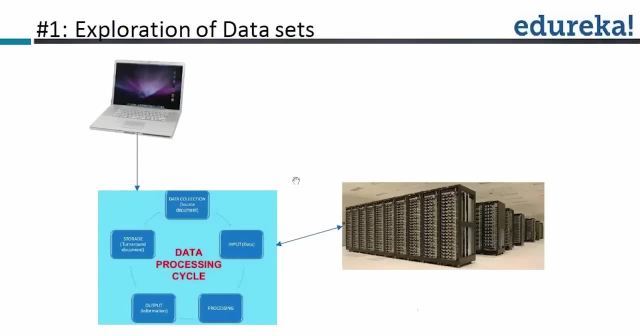 Let's say data mart or you know, like a warehouse where we get a lot of BI reports processed and all of that. okay, It's just a depiction on that aspect. Why Huddup for Data Science? Okay, sorry, 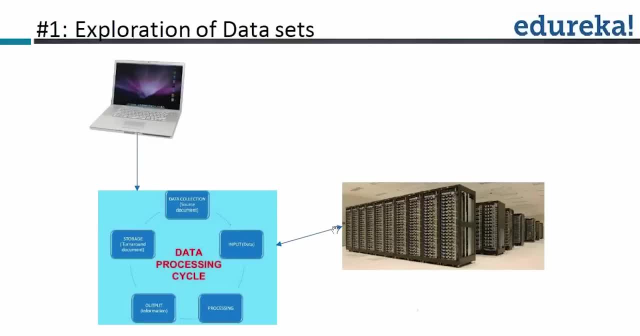 Exploration right Of datasets. So, friends, one thing I want you to understand before I go a little deeper on this is data science, data scientists, right, If you look at, even if you Google it, and all that, most of them are like you know. 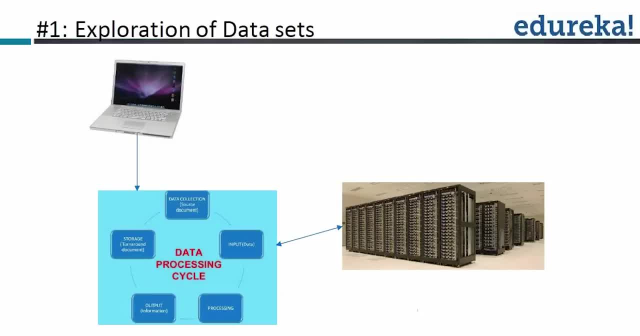 have a strong background in mathematics and statistics and you know they come from PhDs and you know operational research. you know they come from such a background, right? so? because? because they need to tune the algorithm, they need to optimize the algorithm. you know they work on things they need to understand. 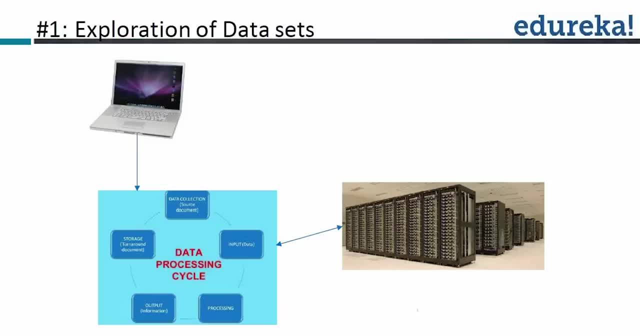 the. you know how the algorithm works and all that, so they need to have such a background. plus, you will be very, very surprised. most of the data scientists spend, I would say, at least sixty to seventy percent of the time in data preparation. in other words, data preparation involves going by, you know. 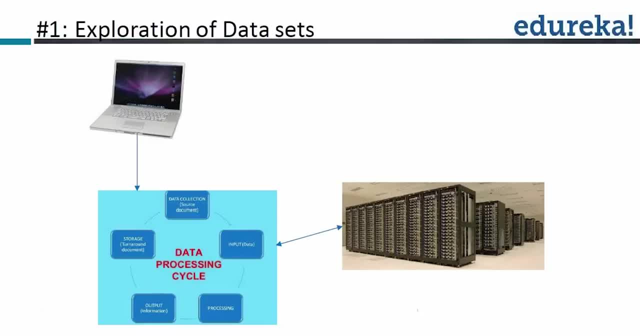 cleaning up the data, because data comes in myriads of sources. right, it comes in different avatars, so they need to clean up, make sure that data is ready for analysis. right, even for them to get on. get to that stage. text number one: right, so they need to be prepared for analysis. right, even for them to get on, get to that stage. text number one. 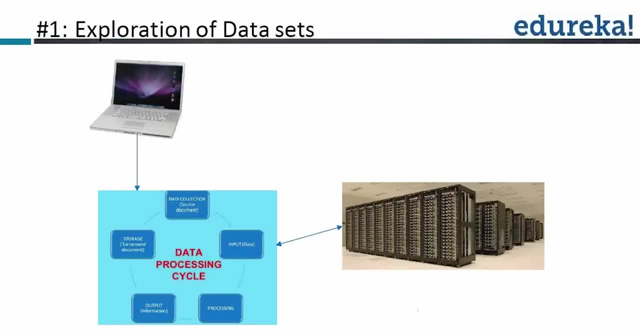 while takes them quite a while. right, because data comes in unstructured packets so they get, you know they spend significant amount of time doing that, right? so if you look at this data processing, exploration of data sets, so exploration is one of the you know data exploration, again, you know they, they may. 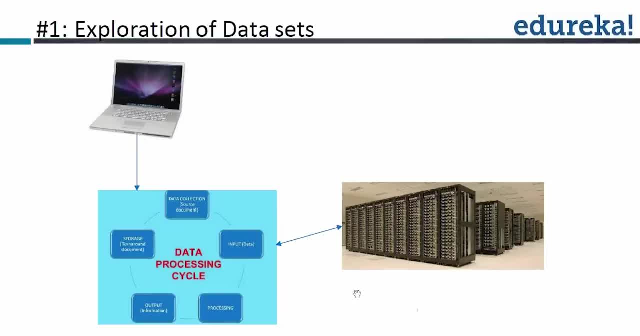 do exploratory analysis. they can mine the data. mining the data is like looking for insights and, you know, looking for outliers. they look at the data dictionary and look for. you know, as I told you right, you cannot simply do an outlier. you know, just like that, some knowledgeable person will know why you. 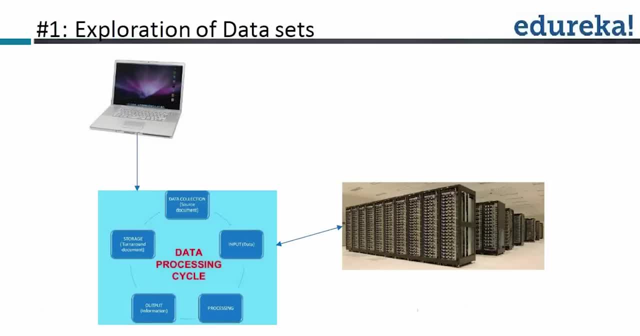 know an anomaly versus a proper. you know meaningful data as well, right? someone should be able to point that out. so all these are, you know, the analysis part of it, right, it's, it's, it's quite a significant part before it is. you know properly. you know before we can make out. 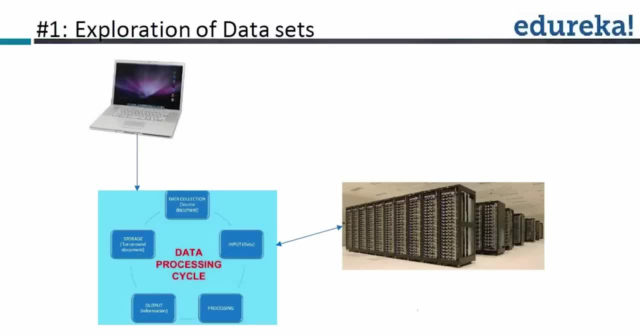 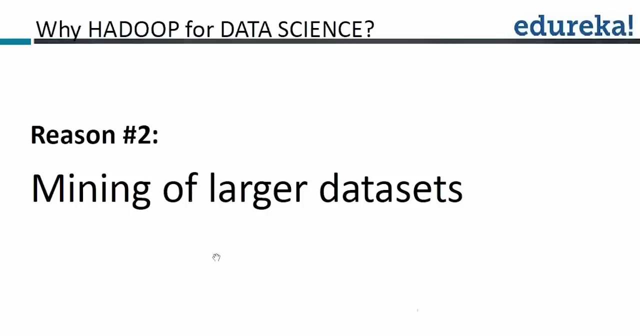 any insights out of the data. first thing is we make the data, the structure of the data, meaningful so that it's ready for analysis, so that preparation stage is like very vital. then we take it for to analysis. there are a lot of steps involved here: mining of larger data sets, as 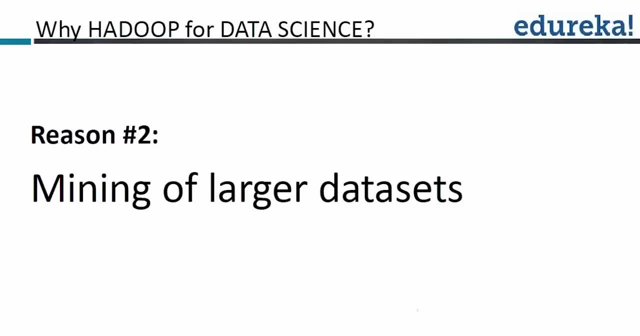 I told you data mining. you know there are different models for data mining as well different techniques used for right. so people use, you know some of them use SAS, some of them use Hadoop and some of them use are. so a lot of techniques are there in we. our relevance here is like you know why Hadoop right, so we will look. 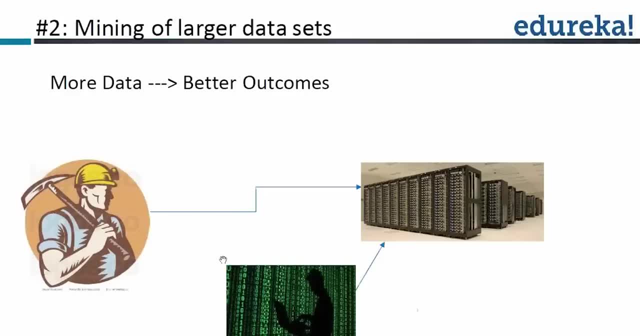 into the Hadoop aspect today. so what do we do? better outcomes, right when we do this: more data, better outcomes. so, friends, well, the other thing is, like you know, the more and more data you unearth, you make analysis out of more data. right, because even in your null hypothesis and all that, we always look at historical. 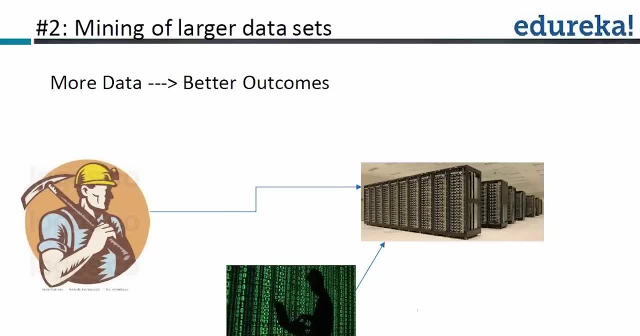 data, okay, and we try to discover patterns. so one quick example, friends, something you know: the data science how it is evolved today. so most of the, let's say, retail outlets, lot of this business domains, have enormously got benefited and I would just give you a small example. back in, 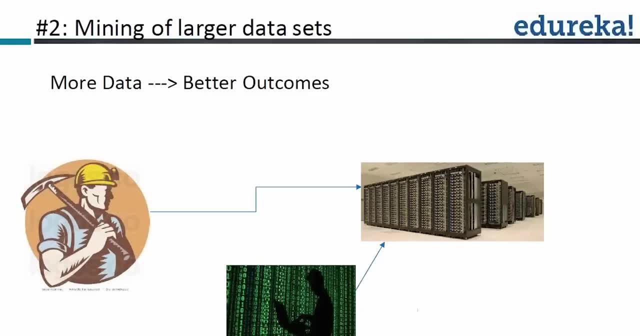 2000, or you know at least 10, 15 years back, right in supermarkets in us also, which was fairly well equipped and all that right. so people used to give a lot of coupons, lots and lots of coupons. most of them will not make sense to you, suppose i go to a. 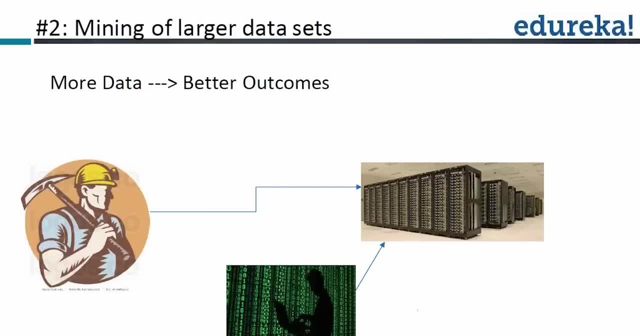 supermarket, right, they'll give me coupons on, you know, home products, baby products. you know i'll just trash them without even taking a second look. okay, yeah, i'm coming. upendra is asking how market researcher could use this hadoop. i'm coming to that, upendra, yeah. so now, as times have evolved, 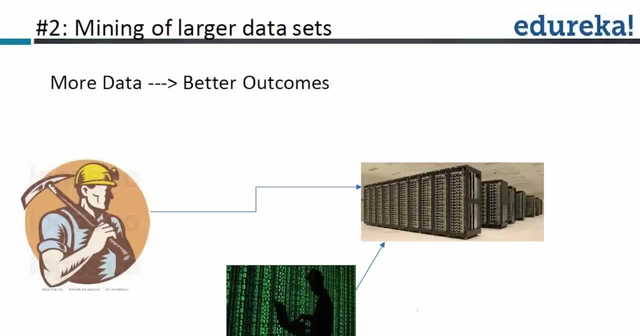 right, because most of them, you know you will just trash them, right, these coupons, and all will not make sense. now people have started observing the customers buying patterns. they are making deriving insights out of it. insights out of it, right, they are deriving the buying patterns. now they are sending coupons. they are sending, you know, relevant coupons to relevant customers or buyers. 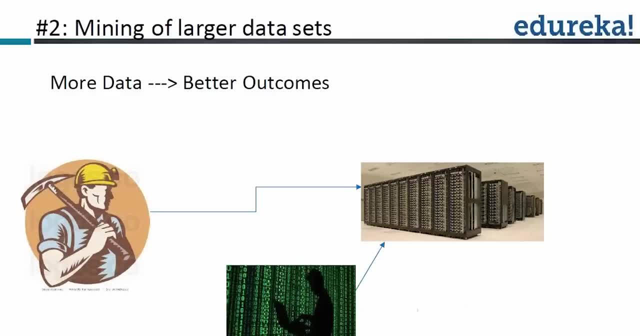 right. so it really makes you know and they, you know. it not only gives uh, you know, uh, customer loyalty, it also gives you know customer retention, customer you know more customers, you know they go happy customers. it's a win-win for retailers as well, right, so it has become a very uh success. i mean it's a. 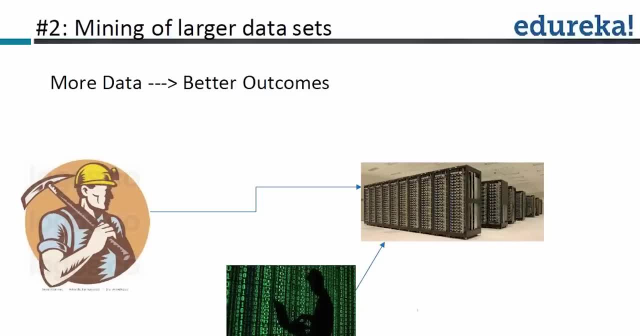 huge success story for the uh in the retailing. i'm just saying i mean i can replicate this story for so many other domains as well. now to answer upendra's question how market researchers could use this hadoop. can someone take a guess? friends, i told you a story. 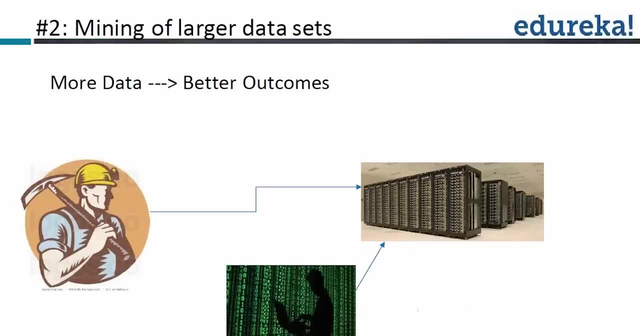 okay, which is which is a real story only. but how do you think upendra's question can be answered? i think you already know the answer in a way. where do you think hadoop will fit in here? any guesses here, friends, look patterns, okay. identifying patterns, okay, uh, okay. yeah, ashish has got a point. it says hadoop can store patterns of each customers. 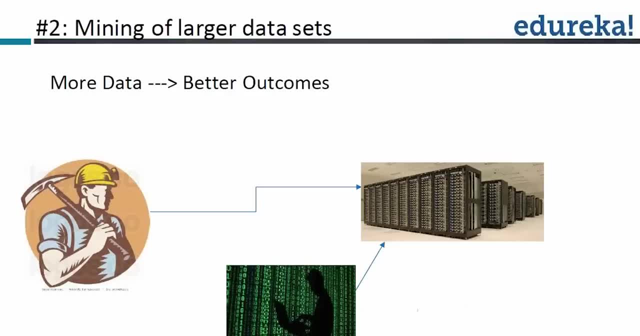 okay, behavioral buying, other patterns, okay. so one thing: friends, parallel process: okay, great, see, uh, how do can store this data? okay, we are talking about a very, very large database. right, because if you look at some of the major super markets in us, like kohl's- right, these sears, these guys have moved on from their traditional 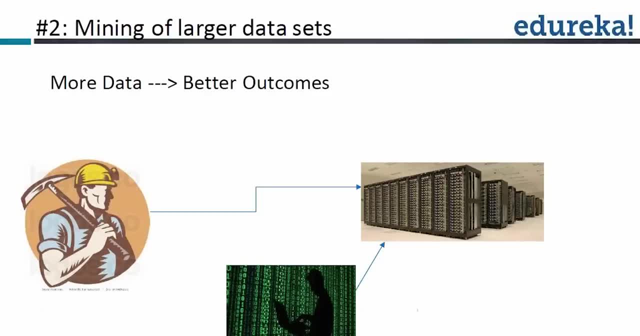 oracle to hadoop. if you go to sears, if you see their data architecture they move down to, you know, hadoop cluster properly, right, so data stored together associated. yes, sajith, yeah, maybe, yeah, correct. so data intelligence data, because we have got a lot of analysis tools in the data. 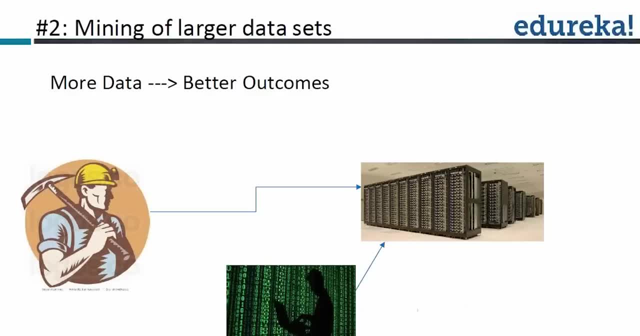 in huddup, which can be used to derive to analyze the data, right we are see, data science is all about, you know, preparing the data and analyzing the data. so hadoop can be very well used for data analysis and storing the data and, of course, data analysis right. so we need to store the data over. 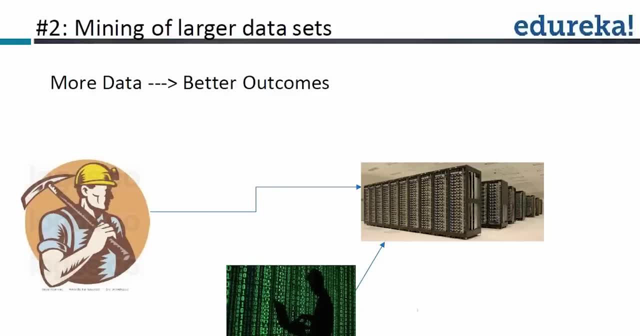 and above. i mean on that data. we analyze the data, right. we analyze the data that is stored. so how do what can play a significant role in the data analysis process in huddup? so how do can play a significant role in the data analysis process in huddup? 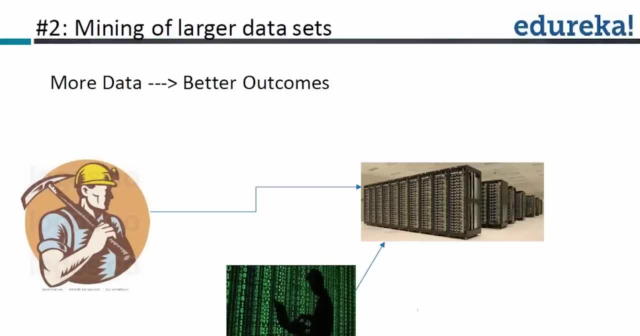 major role in keeping the data, like storing the data which is at a, which comes at a- very- uh, you know- low cost, right? plus, we also do extensive analysis using the data. is that clear, friends? what are the analyzing tools? yeah, funny, uh, analyzing tools. we have hive, we have pig. 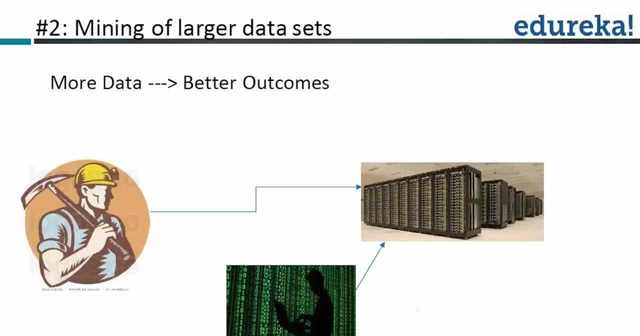 right, this hive can help us analyze. and there there is impala. i'm not going to go there, but you know i'm telling there are lots and lots of tools there and you know, daily there are, you know, different versions coming up, but you know the major ones are uh hive and uh pig. i would say uh. 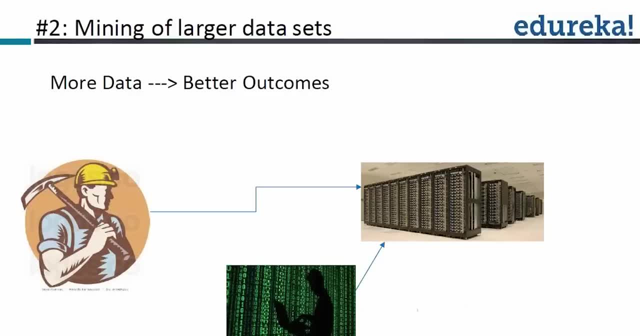 tableau is: uh, uh, it's more a visualization. uh, uh, platform finish, uh, funny, yeah, yeah. so that is more a visualization. it's a brilliant platform and you know, in fact, Tableau can work with Hadoop, you know. just to let you know, tableau can work with Hadoop also. 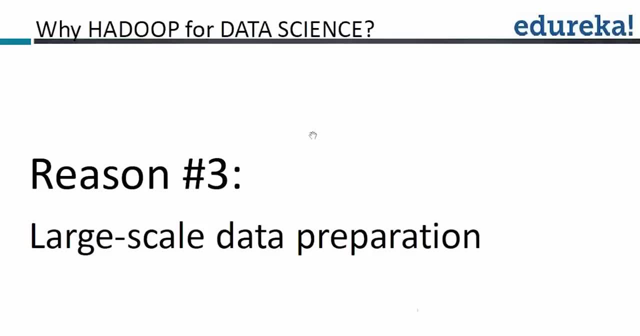 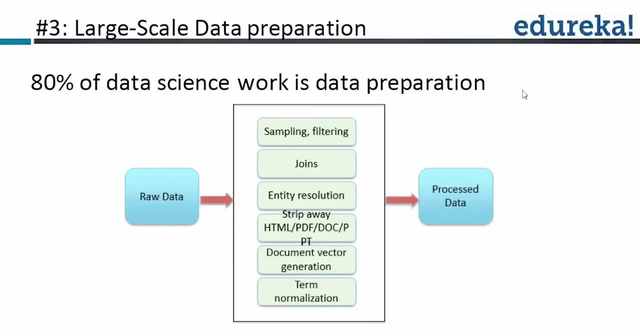 You can integrate it for reporting purpose. Absolutely Correct large-scale data preparation. Look at this, friends. 80% of the data says okay. Okay, I was bit off. I said 70%, right, so 80% Significant. look at this: Joints entity resolutions. trip away HD. you know you need to prepare the data that needs to be mined or analyzed, right. 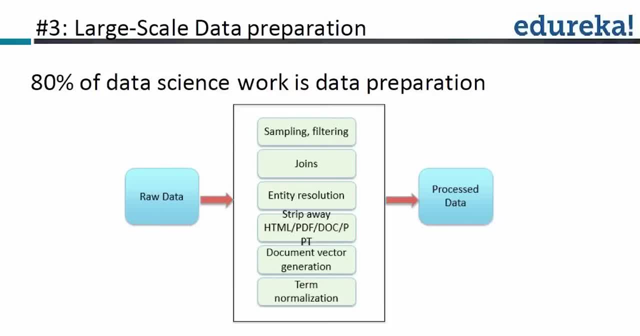 So the raw data, whatever comes in, will be completely unstructured. You need to Really make the data, You need to prepare the data so that you make it more meaningful for analysis, right? You cannot simply analyze the data. Just imagine, friends, you know, if the raw data comes in, which is to your highly fidelity data. 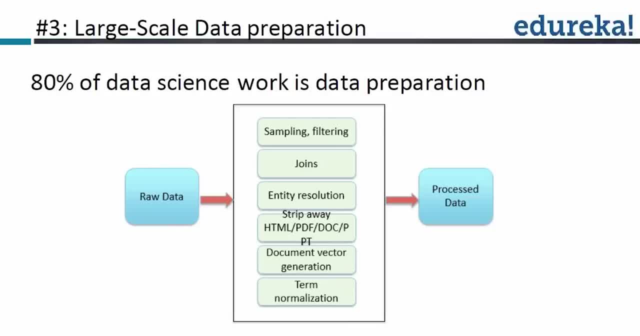 Absolutely, but same time it needs to be. if you want to analyze it, You need to bring some sanctity to the data, right? So You need to take care of these aspects. Okay, a lot of aspects, right? sometimes the data will come in. 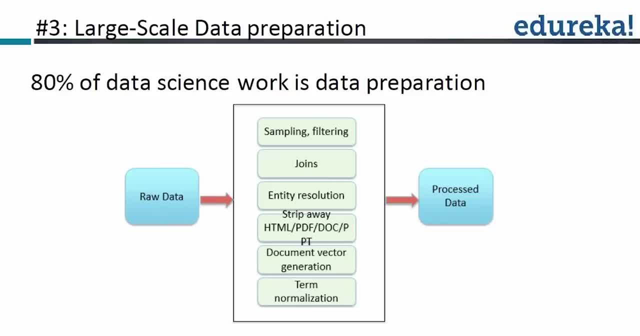 You know. I'll give you a very small example. Data comes in like you know one source. it is coming, The date is coming as DDM of Y by another source that is coming from us. It is common coming as a mom DD yy, right. So you need to sort out these things using you know. 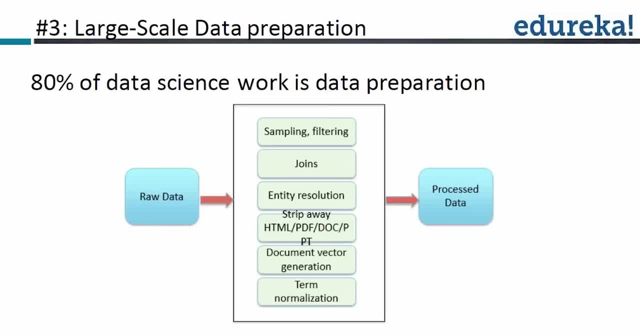 You know you need to use Either a map reduce tool or something like a Some processing engine. right, can you can even use PIG- it's an ETL tool- to do transformation To make it more consistent. right, You can use a regular expression. You can do all those things to do cleaning up the data so that it becomes consistent. 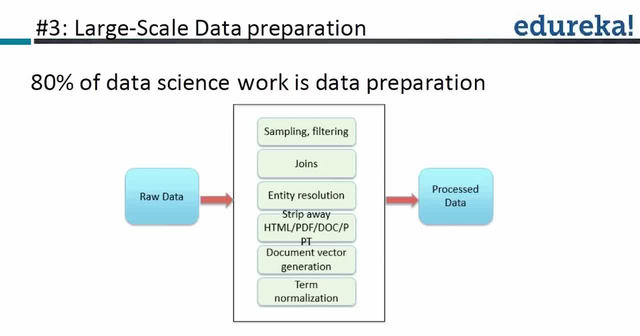 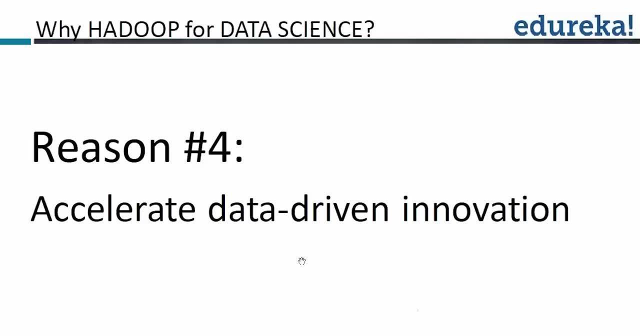 Then, once the data is foremost structured, you can do it, do the analysis. Yeah, so this is how the cycle is Accelerate: data driven innovation. So today we're going to talk about the. say one other thing, friends, there are not, you know, the Apple, what we have, you. 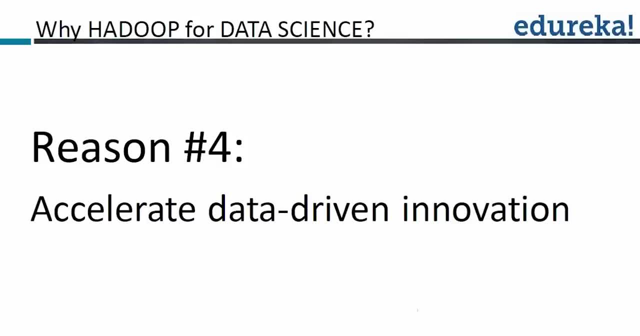 know I may be talking something completely out of the back, but I still want to tell you this: see, Jen, most of the companies, if you look at the marketing strategy, right, they all come back and say that you know they do a survey, proper survey, they do this pestle analysis. there are a lot of marketing. 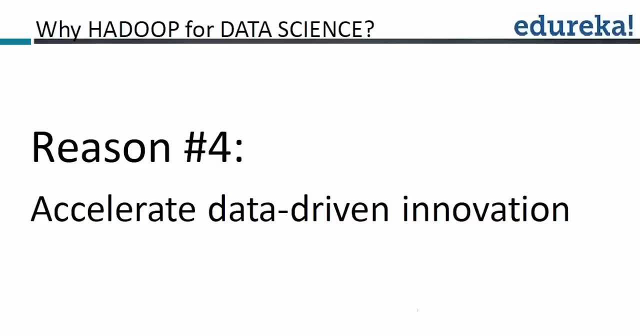 you know strategies, how you study the market, how you look at the segment, segmentation, customer segmentation- and they look at their locality, they look at the location and they look at the people. they do various things right before they launch a product. not many of them. or you know, Apple is like a one in a billion. 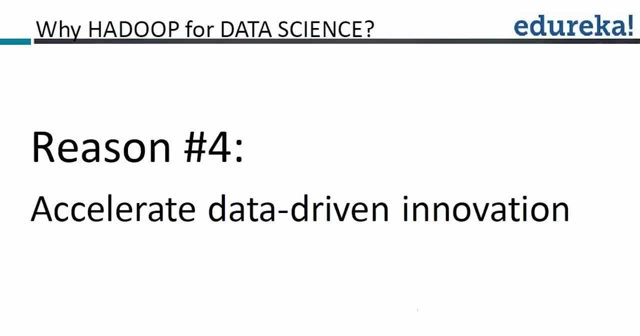 right. Steve Jobs had the foresight. he said: I'm not going to go by the market, I will define the market right. how many people have that guts and how many people have that conviction to still succeed? right, iPhone succeeded. we all know that. but most of them you know most, or you know. if someone says: 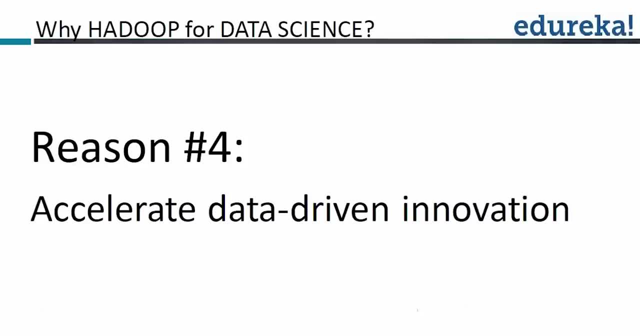 something out of thin air. of course, Steve Jobs had the financial muscle as well to launch a product like this, spectacular product like this. but how many people will have that leverage right, think about it. so if someone gives a statement like that, you will say: can you show me some backing source, can you prove it with? 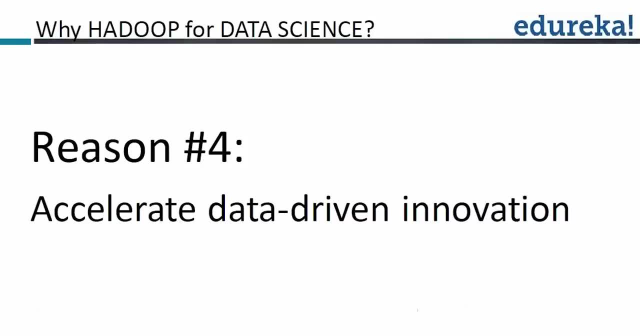 your data right. data plays a very vital rule, so we always want to ensure that you know it is supported by some data facts, something which is data driven right. so data driven innovation is far more. I would say that you know trustworthy or you know it's going to be more believable, or it's it, can you know? 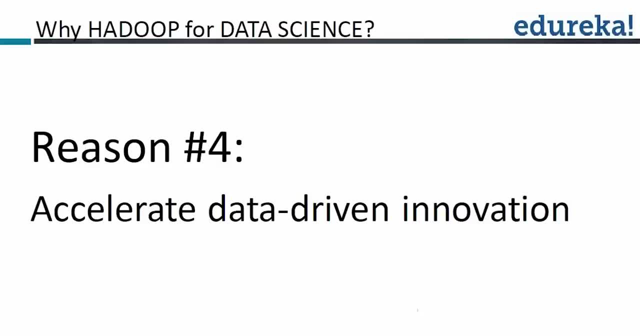 the chances of success in using data driven innovation is going to be- it's going to be higher than you know- something which is not backed by data, right? so sorry, I went to that example. you know, just to quote you, that people, you know something which need not. 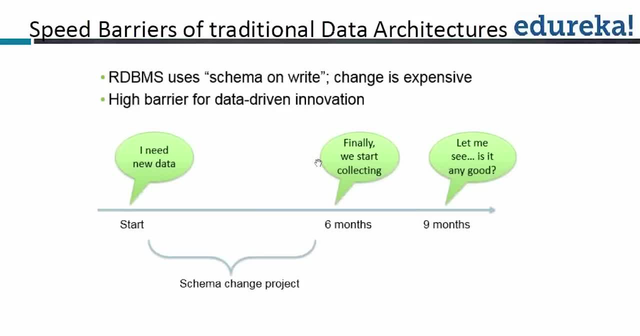 be. data driven also can succeed, right? I want to tell you that. look at this schema on right: change is expensive. RDB was right high barrier for more data driven. okay, upendra is asking more data. okay, anything you know, Apendra, I'll tell you. let's say, your World Cup, soccer 2014. I don't know how many people, what soccer. 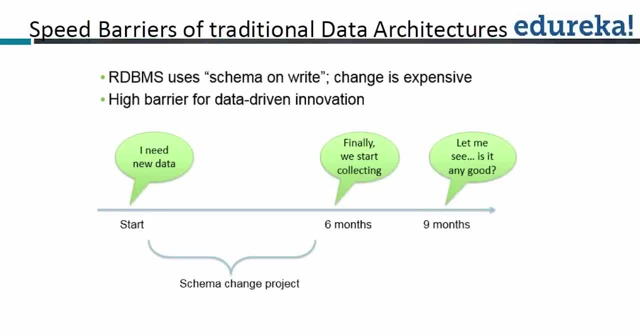 write the World Cup of Socorra chuyp analytics from Germany. right, they did extensive analysis on the data. they looked at players. ПЛАИСпЕ�� ×玩怕 PLAYER- ПЛАСЬКО DATA. they looked at players play업. 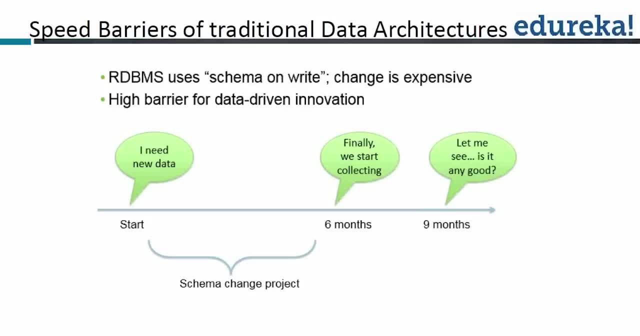 profiles they looked at. you know how. you know Germany was really. I would say that you know. I think I don't exactly remember the number, but you know I can tell you the, you know the overall strategy, what they did. they figured out that the ball position, right ball position of every player in Germany. 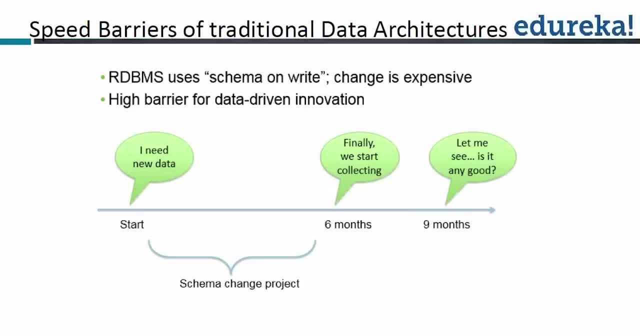 right. it was about six. six to seven seconds, or or rather five seconds, I would say. they brought it down to by one and a half seconds, so it became like three and a half right, for every player will be possessing the ball within themselves, so they were passing faster than how they were passing earlier. this. 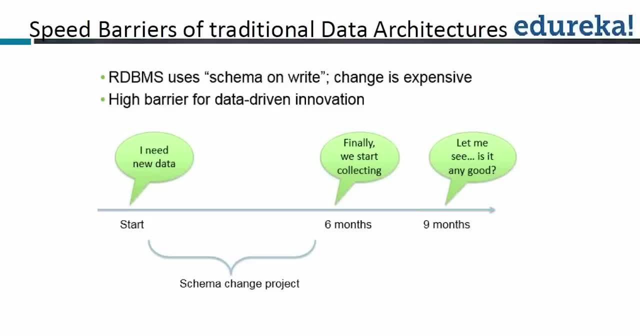 completely disrupted. the opponent players, who have just not prepared SAP analytics, gave this. you know. they did this analysis and told the German team: if you do this, you are, you know you can easily penetrate into the opponent's defense and you know the rest is history. Germany went on to win the World Cup right and 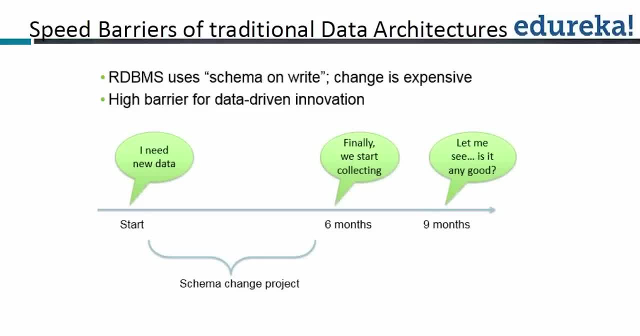 you all know how they ate Brazil for their lunch, right the semifinals it was like 7-1 or 6-1, I don't know what was the score line. they just thrashed them. and brazil, you know, surprisingly, brazil team had 51 percent of. 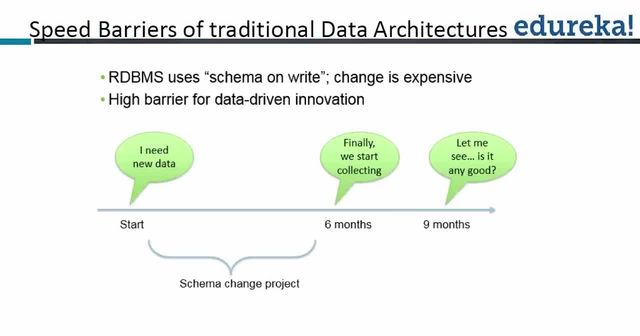 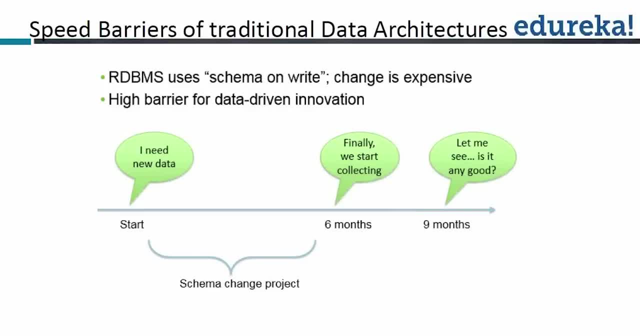 defense of Brazil. see, I'm saying: you know data driven, right upendra. there are so many things you know. you can say: you know how people do the patterns, you know the buying patterns, whatever I told you in Sears supermarkets, they are all data driven. just for your information, everything is data driven. is that clear? 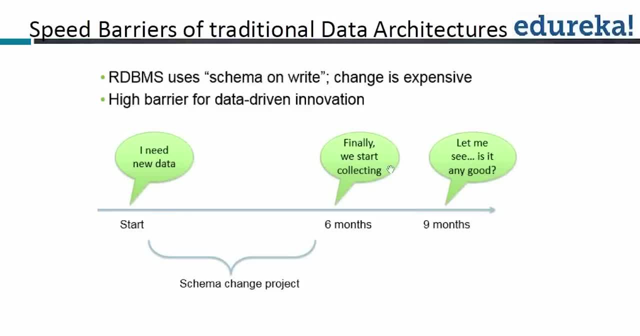 upendra, yeah, sure, so new data. finally, we start collecting. is it any good schema? see, look at this right schema and rate our DBMS. we all know it uses. see, it is a very, very strict schema. right, the schema is defined well in advance. then we start. 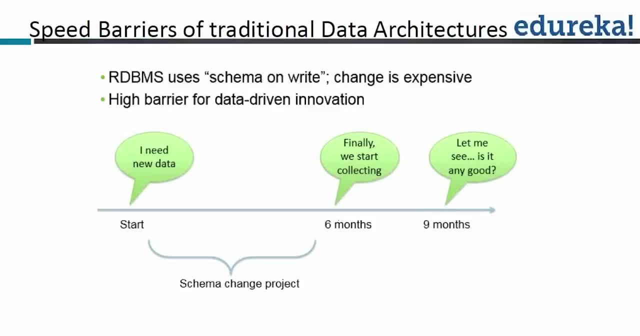 inserting the data. fine, then finally, I mean, we start collecting more and more data. is it any good? you know, it's like high barrier for data-driven innovation is like if you want to change the data, you need to be able to change the data schema. after some time it's going to be a problem, right, because it's all fixed right, whereas it's a. 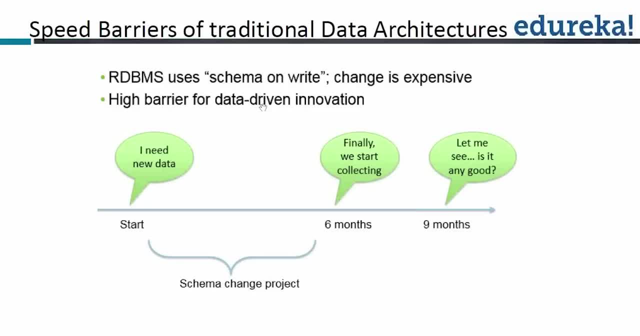 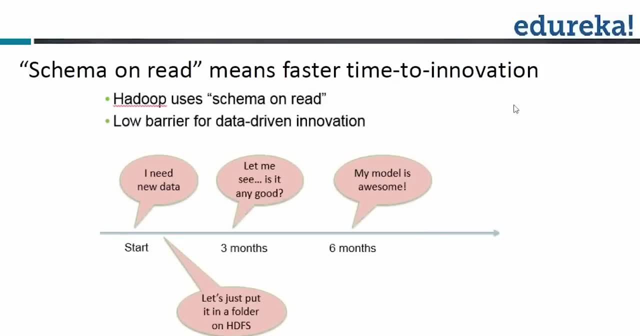 high entry bar, i mean high barrier for innovation, whereas if you look at hadoop, right, you can just put anything there you can put up. you can just push an elephant onto right schema and read: low barrier, okay, so it's. it's simply going to put it in hdfs. you can write any kind of data, any kind. 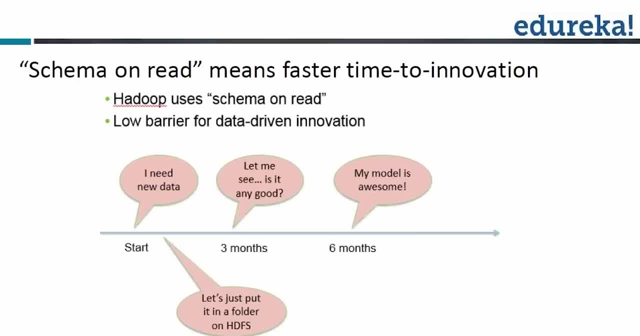 of unstructured data. also, it's a schema on read. there's a schema on right for rdbms, right, so that way you know how to. provides distinct advantage of: uh, you know the data being stored in a unstructured format and all that right, it is schema on read. so this makes makes it a lot more flexible and fluid. 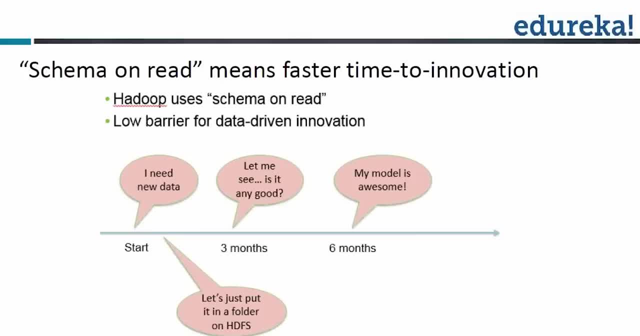 for data driven innovation. so how to provides that operational advantage, i would say in the long term, right? so, friends, any questions? before i show you a quick piece, you know, any questions so far? schema and read. okay. okay so friends, what i, what we say, schema and read is: 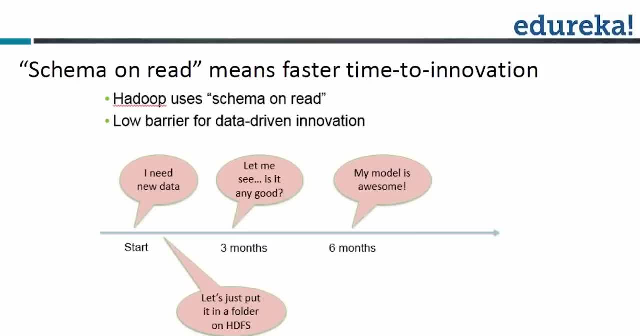 see when we are: uh, can you insert data without defining the schema in rdbms? can you just insert the data- yes, no- into rdbms without defining the schema? no? the answer is very clear. all of you know this right in hdfs i don't need to define anything. i can blindly insert data. right, i'll simply go and. 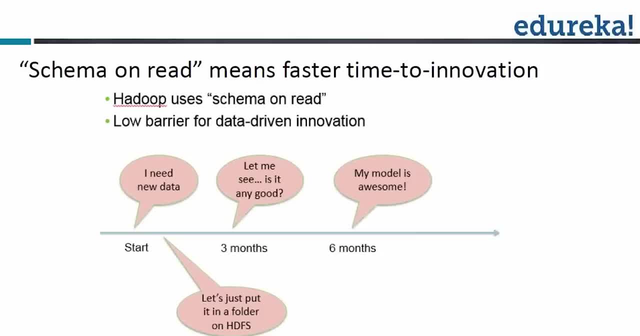 insert the data that is possible in hadoop right hdfs, which is your hadoop distributed file system, whereas in rdbms it's it is schema on right. that's why you can trust the data that is coming from rdbms. you are imposing the schema which is going to act as the gatekeeper. 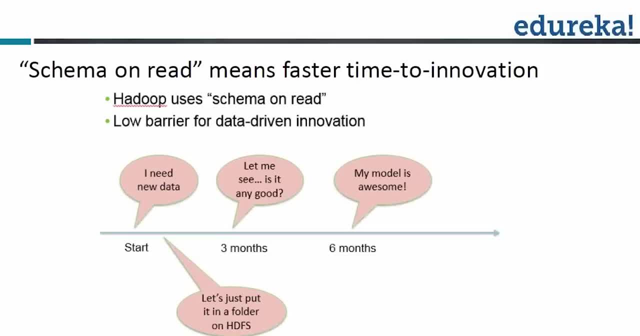 right. so it is going to have all the integrity, data integrity, everything is there. it's going to have this acid property and all that, when it comes to how to schema, is nothing but your design, danish, nothing but your design. let's say: in a table, danish, a quick thing is in a table you. 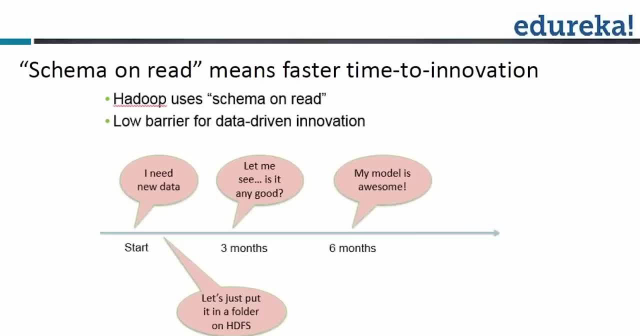 have rows and columns, right. call up one. i'm going to say name, age, gender. okay, name is danish, age is, let's say, 20. gender is male, right? so this is your schema. fine, so i need to have this very strictly defined in a rdbms, right? so this is schema on right. 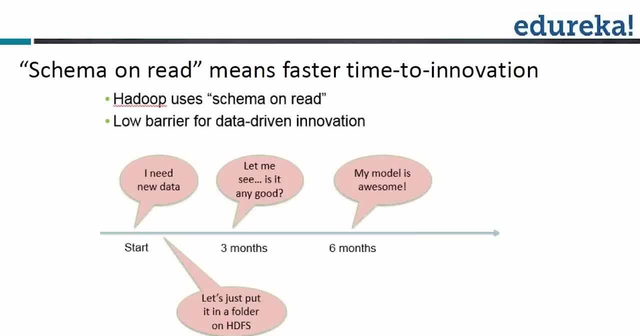 in htfs or hadoop, i blindly insert the data, that's all. but while reading? fine, while reading i can define the schema at that point. right suppose i want to load data through ping. ping is one of the ecosystem tools of hadoop. when i want to load the data through ping, i'm going to. 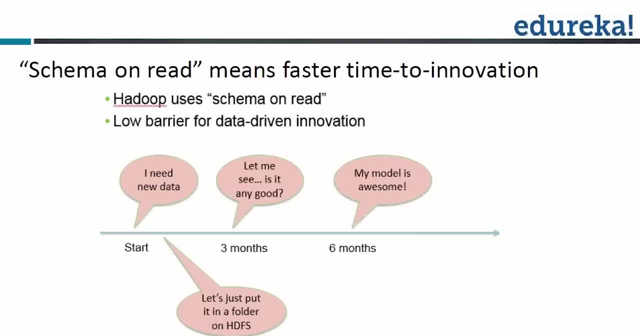 put the. i'm going to load it right. at that point i need to define the schema. that is, schema on read. okay, uh, i have another question. my, my, my, my previous question: does hadoop has any relation to natural language language processing tools? individual need that actually see nlp? uh, it's more to do with text. 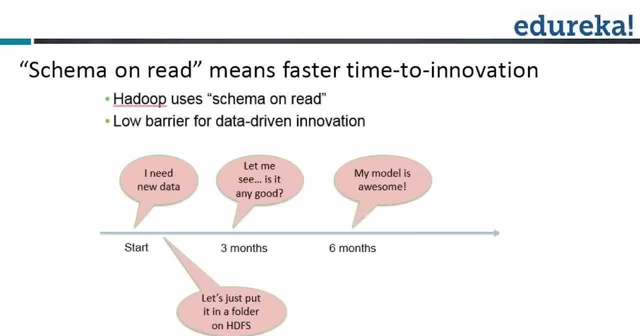 mining damodara. so, uh, i'm not an expert in nlp, but i can tell you that you know you can still use hadoop as a medium to process the nlp. you can still do that, that's possible and it is not like you know you need to have the nlp, uh to i mean it's if you are really doing the. 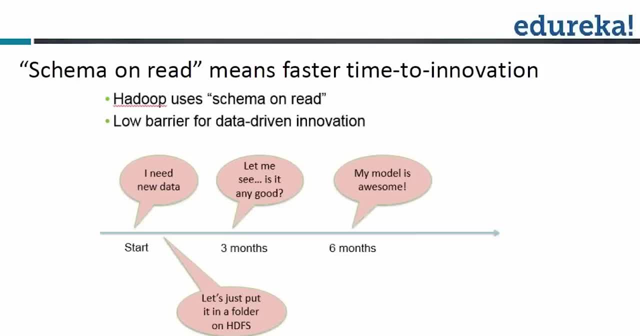 you know natural language processing. yes, you need to have the skill set, but you know if you're not doing that, you don't need that skill set. you know pretty simple. like people who do text mining, you know they need that skill set, otherwise it's not needed, right? digital marketing: how much? how much? 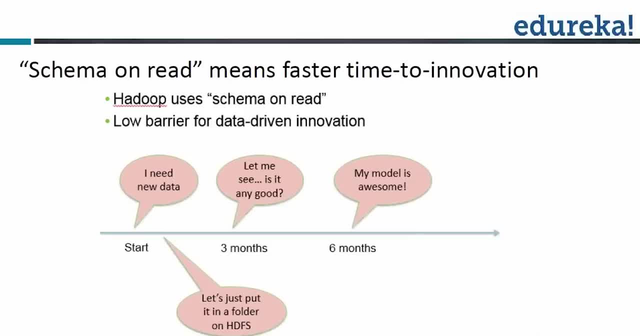 system. that's a great question. digital marketing- sorry, upendra, I'm not quite sure, but I'll try to find out. you know if? because a fantastic question? yeah, because digital marketing. I know that it's the one of the in things today, but I don't know, I don't know where I can place hadoop there. maybe can how to. 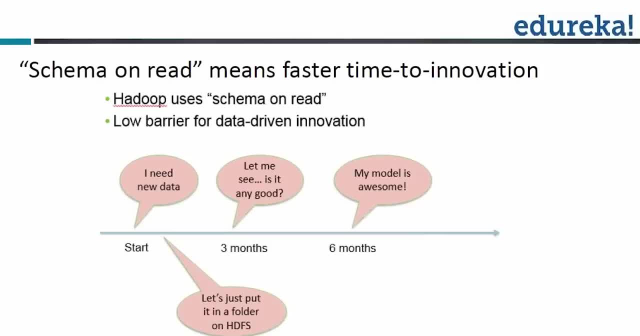 process the data from SAP? yes, max, it's possible, because how to pass, you know, I'm just guessing. open, draw the re. you know, max, I'm guessing. the point is there are Hadoop connectors for most of the leading databases, so I'm pretty sure SAP will have a connector to. so Pedro is de-mistifying. digital marketing is. 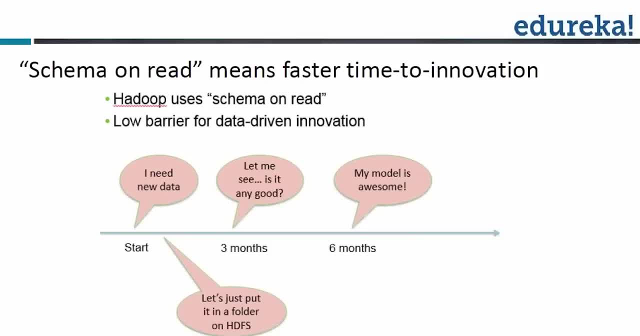 nothing but online marketing. yeah, it's possible, definitely, yes, Pedro. so cross so your question on the digital. if it is online marketing, I can say, Hadoop's, how can we use? yeah, then I can say that you know online marketing, you know, let's say, customer retention, you know looking at 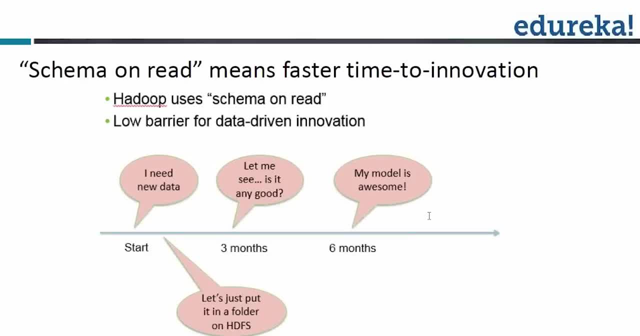 the customer segmentation. you know you can. customer profiling. you can use various things in. you know these are all marketing exercises, right, so you can very well use it there. security of at most no. Hadoop is fairly secure. it's. it's quite secure remote. how can we use Hadoop in cards and payment domain? it is very well used. 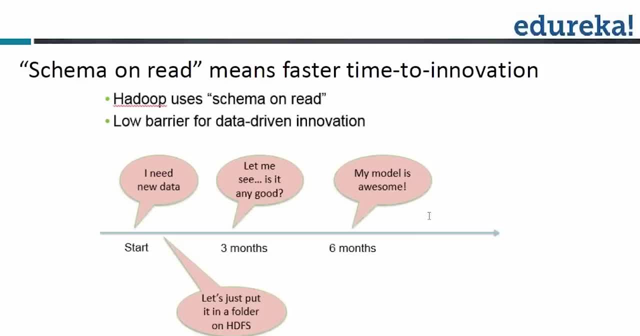 in, you know, but I would say in PayPal, I would say, and you know, Visa, all these guys are actually using it and of the use Hadoop clusters in their organizations and of course, it is secure to how does it help you? I mean, see, people are going to Hadoop primarily because you know it's not for anything. 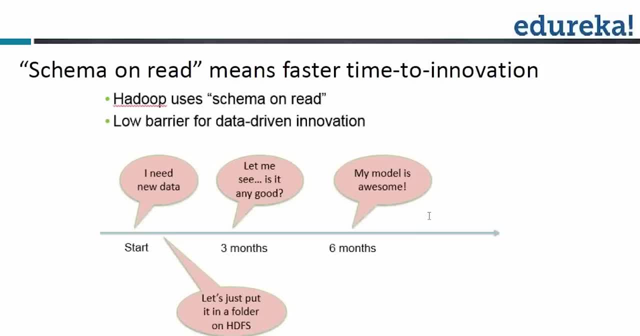 else. it is very, very cost-effective right, because most of these guys are, you know, burning dollars and dollars. it costly hardware infrastructure right. this has become completely, you know, highly cost-effective right, and it is, and of course it gives you gives a very good performance too. there are many. 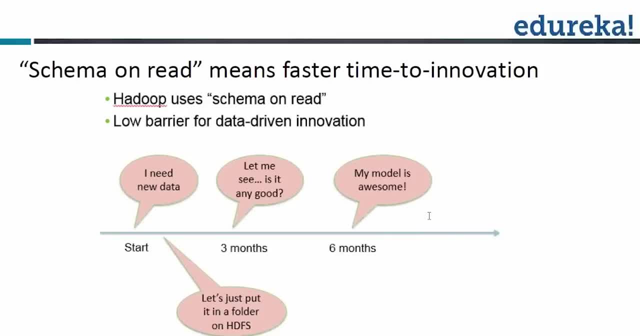 flavors. basic Hadoop, Ashish has got a very long question. if so, what flavor? what? according to better to an open sources of flavor managed by different vendors? okay, see, Ashish. I would say plain vanilla Hadoop is great, right, you just need to know how to install that, and installing is not a big rocket. 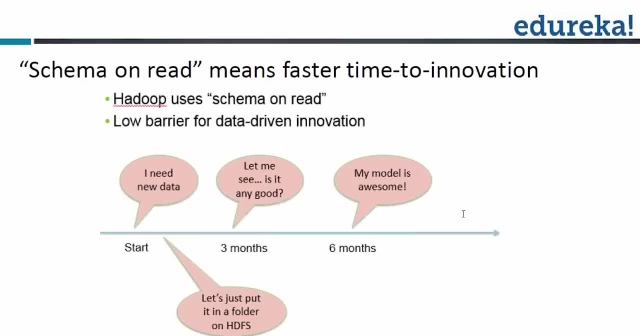 science, you can easily get it done right. I can clearly say that. so, and there are. you know these guys. you know most of the some of the corporates they prefer. you know Microsoft has got it, so you know Microsoft has got it. so HT insights and IBM insights is there, and the cloudera has got its own. 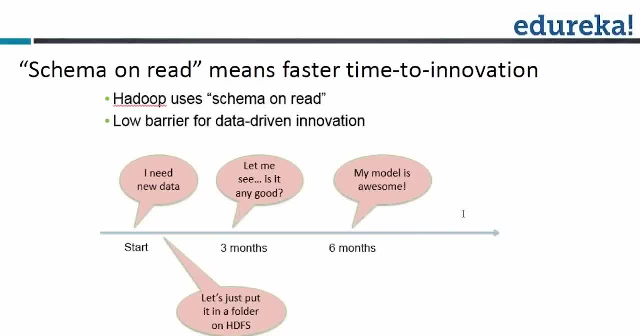 Hortonworks is coming and pushing their own. you know. all these guys are, you know, coming up with the flavors of you know Hadoop. just like Linux distros, right, they people have their own flavors, right. so I would say, you know, if you are so comfortable using the plain vanilla Hadoop, that's great, otherwise you can you. 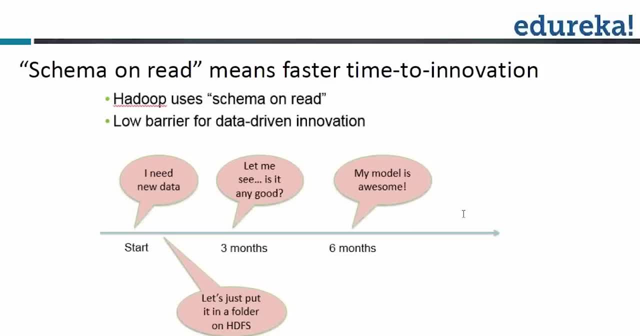 know you can always go for cloudera and all these providers. you know they come and offer you this, so but I would. I am very comfortable. you know I've been using the plain one, so, which is very comfortable. good on right compared to RDBMS. absolutely yes, Neeraj. absolutely yes. how can we use it in Linux? yeah, you. 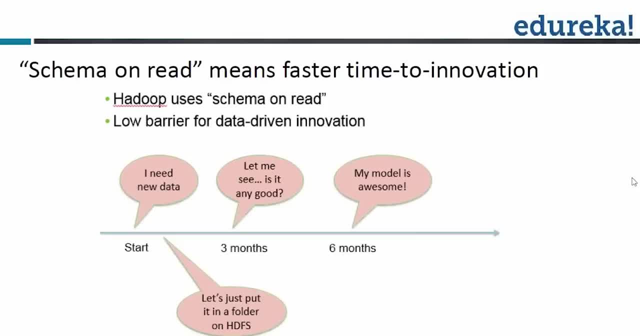 can just use it. Dhanesh, you know Hadoop is available from you know for Windows as well. quite recently they've launched that. you know it is by default. it is suitable for Linux. I, Upendra, is asking: Hadoop can process any kind of data. how can server protect? 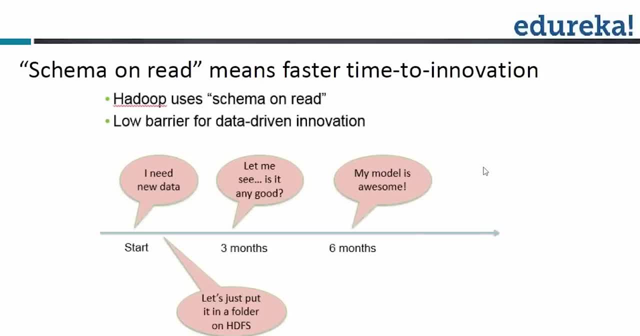 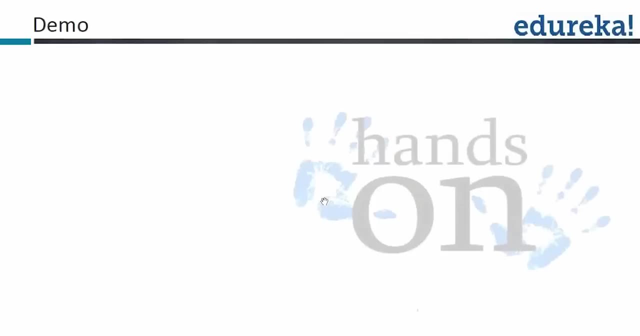 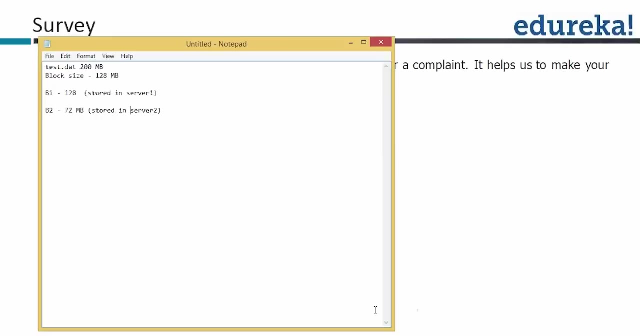 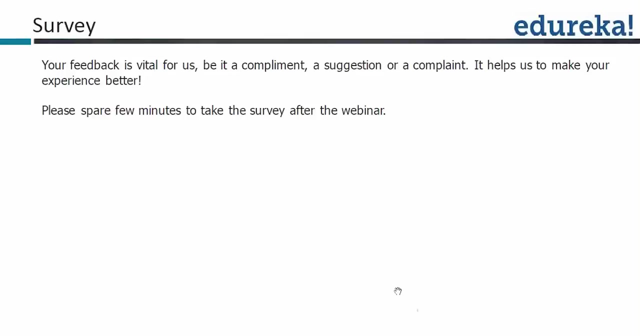 password and ID. no, it goes through a secured shell, upendra, there's no problem about this. yeah, it's not an issue. go through SSH, okay. so, friends, you know, definitely I need the feedback, but before that I just thought I'll show you a very quick- you know, a quick- processing. if you can hold me, hold for another 10. 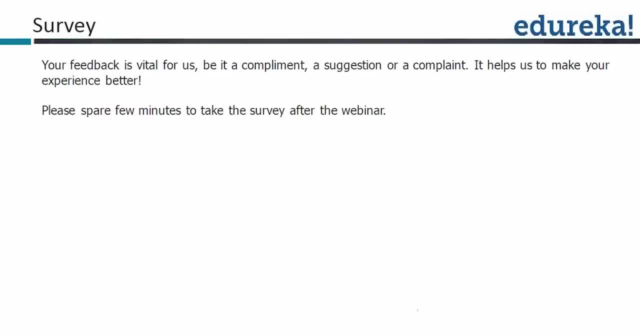 minutes, right, 5, 10 minutes. I'll quickly show you what I you know. is that fine with all of you? yeah, excellent, so just bear with me, sure, so what I'll close this, you know, of course, towards the end, friends, after I'm done with the small lab, I request your feedback, right? so that's very, very. 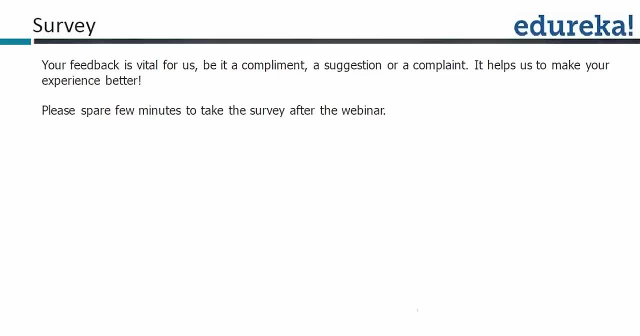 important, you know, as clearly stated here, be it a complement, us suggestion or complaint, you know be very upfront and you know, provide your thoughts, because you know that's definitely going to. you know we believe in continuous improvement, right. 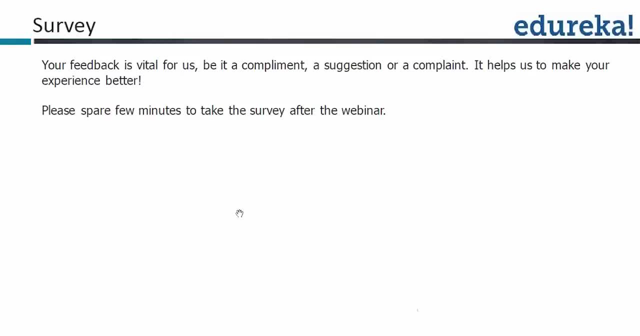 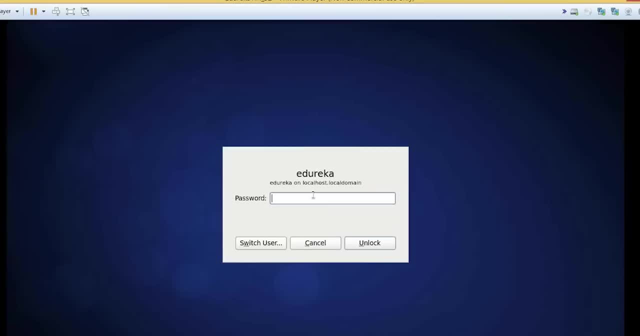 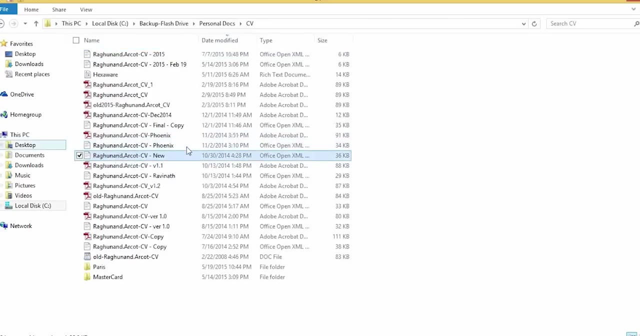 So please help me on that part, Sure Thanks. Thank you, Upendra. Yeah, So I will go to the you know lab session. So what I want to show friends, see here. just give me a minute. 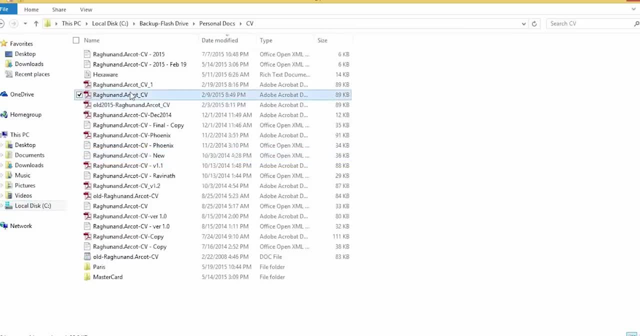 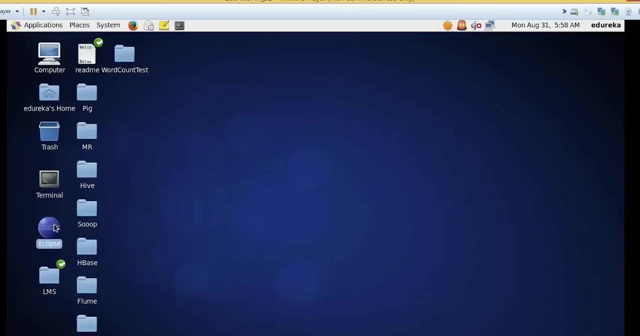 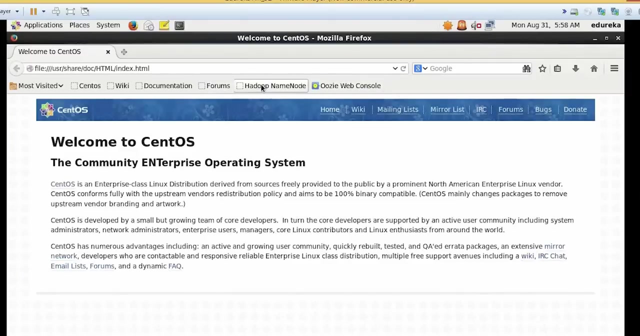 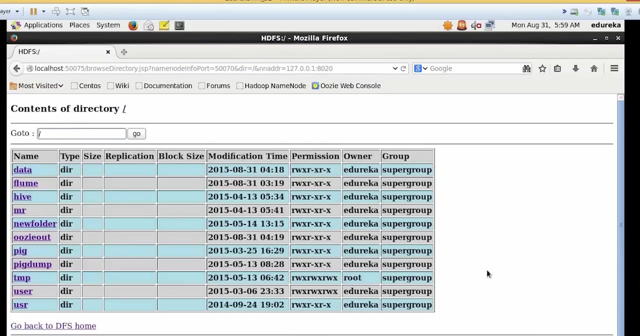 I want to show something like: if I have this, see, I open the terminal. just give me a minute, Okay, Can? I will try to answer this question. Can Hadoop be helpful for Java developer? Absolutely, Devi. 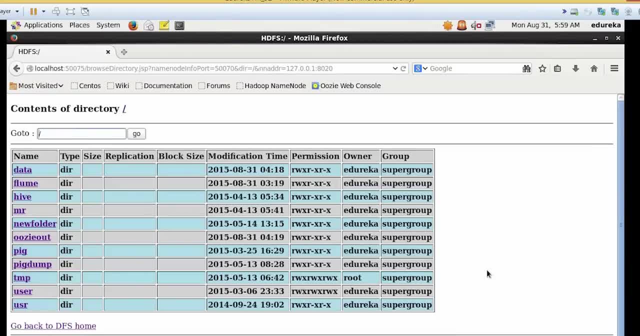 There's no doubt about that. Someone is Java right. It's going to be supremely helpful, No doubt about that. So I want to show you something you know very, very interesting here. Just give me a minute. 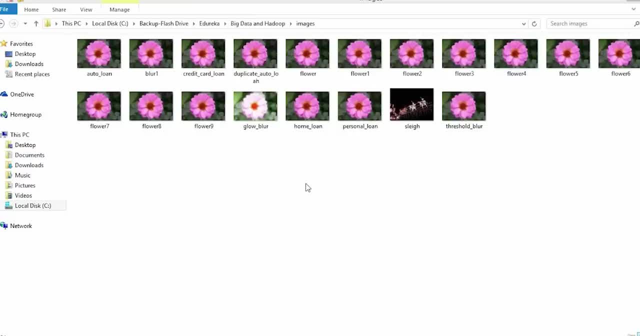 Okay, I got it So okay. So, friends, okay, I have a question here. What about non-Java? Absolutely funny. There is no, as I told you right, Java, non-Java, it doesn't matter at all. 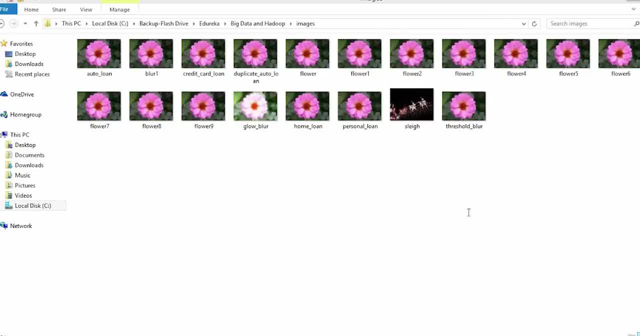 A lot of people have reservation. Can non-Java guys pick up Hadoop? My answer is so overwhelming: yes. So not to worry about that, because big high there are so many flavors. In fact, I understand Java and as much as possible I try to use the non-Java part of it. 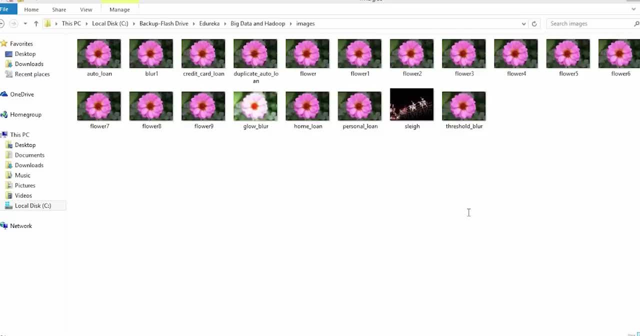 The reason is it makes it even more quicker, right? You don't need to learn Java for that, So that's pretty much it. And what are the different type of job roles in Hadoop? Anil Kumar, Yeah, 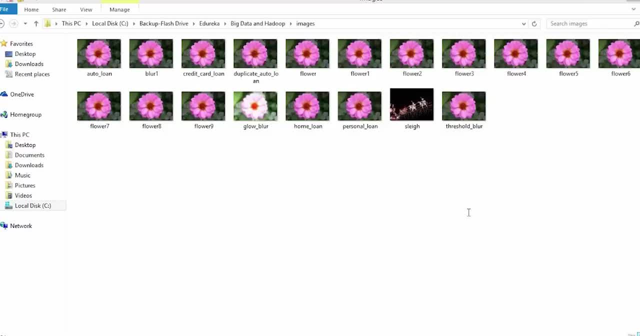 Anil, I think you know you can write from being a developer and you know analyst And you can be an architect. You can be a data architect, You can be a big data architect And you can be a big data programmer. 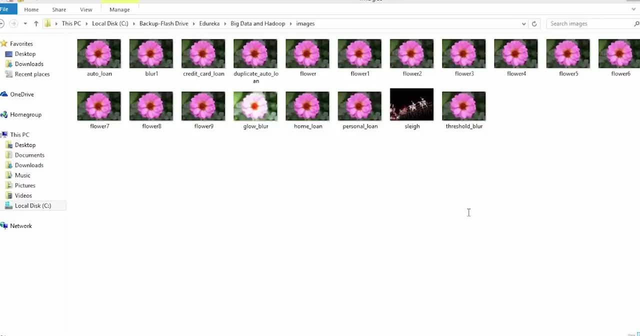 And a lot of multiple roles. It depends, Anil Kumar, where you exactly want to go. Which NoSQL best to learn. That's like us, Okay, Neeraj, great question. There are about 150 NoSQL databases, right? 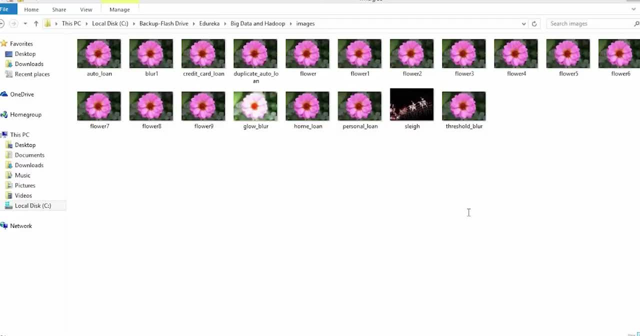 There are 150.. There are about 150 NoSQL databases approximately. So there's nothing like best to learn or anything. I would suggest take one NoSQL right. You can probably start off with HBase or one of these things right. 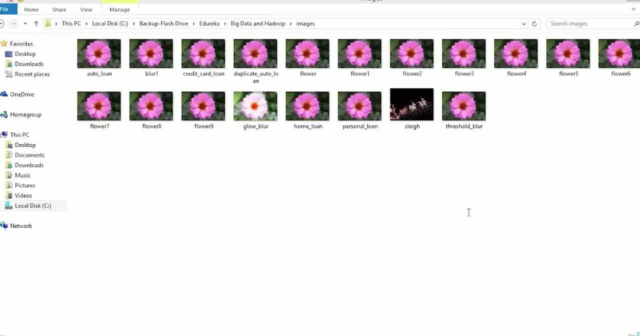 Understand the nuances of NoSQL, How is it relevant, How is it different from a traditional RDBMS. Then understand one NoSQL database, Then you know. that will give you the big idea about you know what is going on. 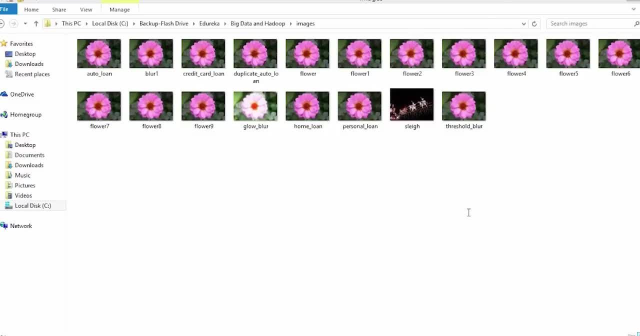 Then you know, then you can move, You can do that. Yeah, So the others should be. like you know, there are different flavors available. Mongo will be better scope. Yeah, possibly, yes, Mongo, yeah. So, friends, I want to show you something very quickly here. 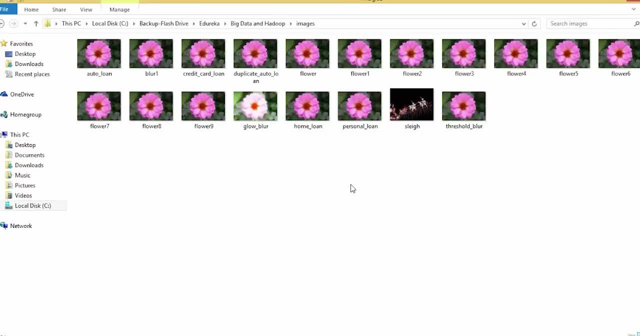 I won't take much time. Yeah, there are categorization. Indira is asking. Yeah, there are graphical databases, There are columnar databases. There are- you know what to say- A database which provides high consistency versus high availability, right? 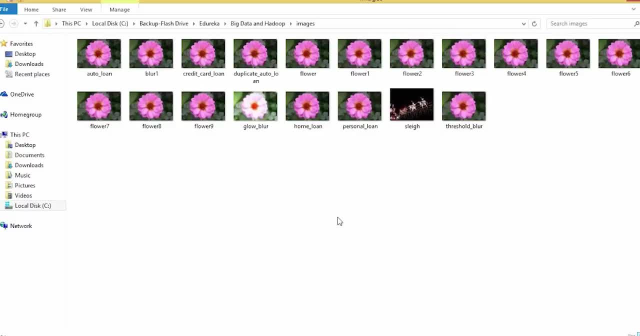 So different kinds of databases are there. You're absolutely right, Categorizations are there. So it's not like you know one, you learn the others will be, But you know you, at least conceptively, I would say that you know there will be. 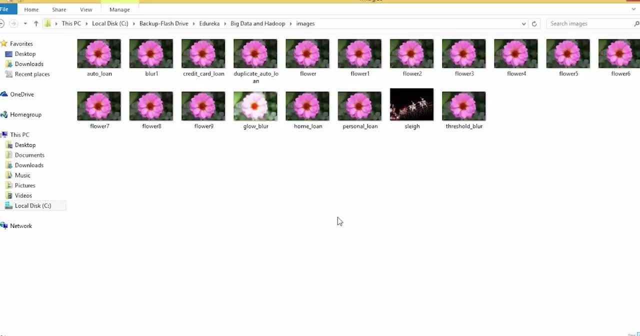 you can at least, at least you can, you know, get to some point. But you know there are, like you know, you know like Google table is there and you know hyper table, And some of them are derivatives of these kind of these families of databases. 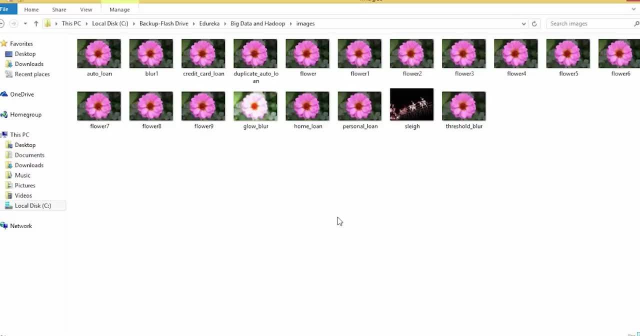 There are different families, But you know at least NoSQL. you know. from that aspect. I'm saying, if you learn one, one or two right, it should give you a broad perspective of what a NoSQL database is. 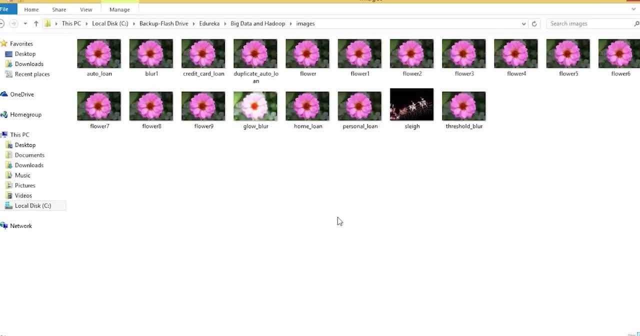 That's my point. How do we get data video formats in real time? Yeah sure, Key value, That's right, Indra. key value pairs and all that. What's the best? if I'm looking for key value, Key value. I think Redis is there, Indra. 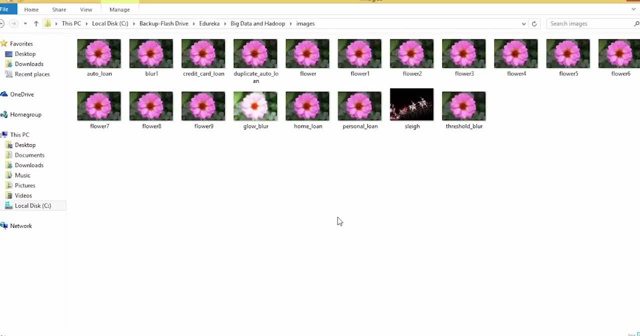 Yeah, Redis is there and Cassandra is there. Yeah, these are all based on key value pairs. I would say, Yeah, that's right. How do we get slides and video recording? Sure Slides, of which one Rajat. 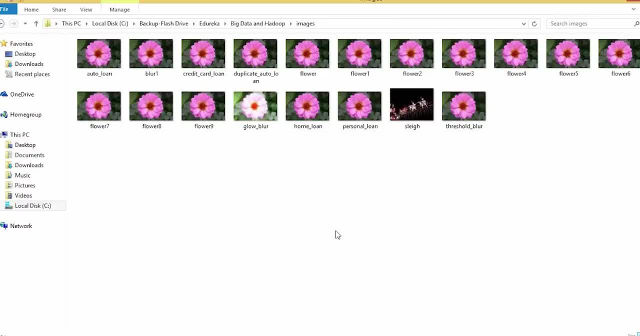 This, this session is. this session is recorded. Rajat, You may need to check with Edureka support. You just need to find out the other ones, You know. you may need to find out. You know whether this becomes available. I think you can check with the support. 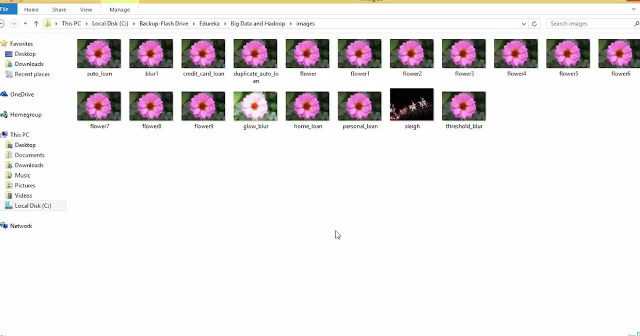 I'm sure they will help you. Yeah, So, friends, just want to tell you this is like a quick problem, right? I'm not going to go explain the overall things, right, But This is a, you know, a simple analytical task. 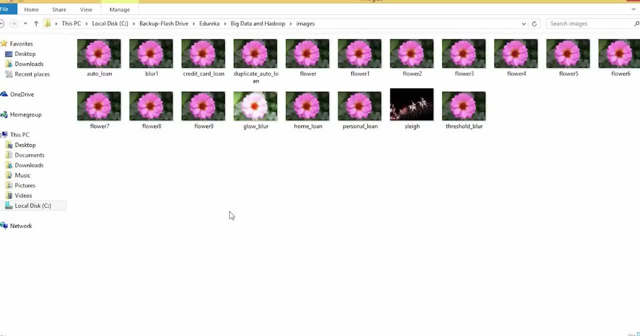 How Hadoop is playing a major role. I want to just tell you this: right, Look at this number of flowers, Right? Can you all tell me your observations? Just a high level observation. They all look alike in a way. Is that correct? 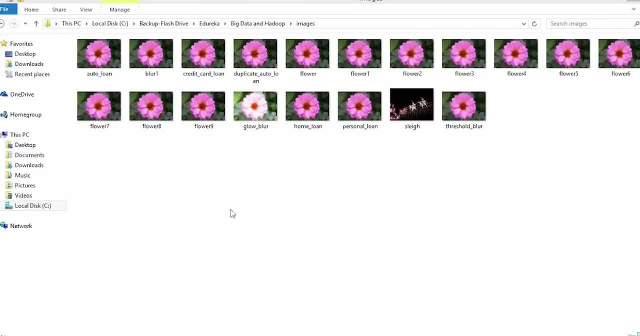 Names are different. OK, There are a lot of just majority. look like a look alike, correct? Yeah, Friends, you know I want to, you know, just want to lead you on to this problem. These are. these are all types of flowers. 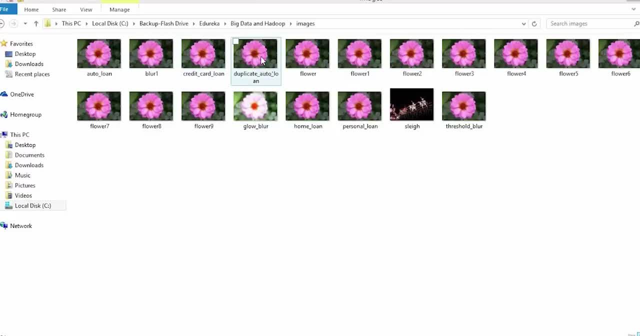 Right, And This one. This is nothing but the duplicate of this. OK, This flower is getting duplicated nine times Right. So, in other words, I have how many flowers here? Nineteen items selected Right, So I have how many duplicates here. 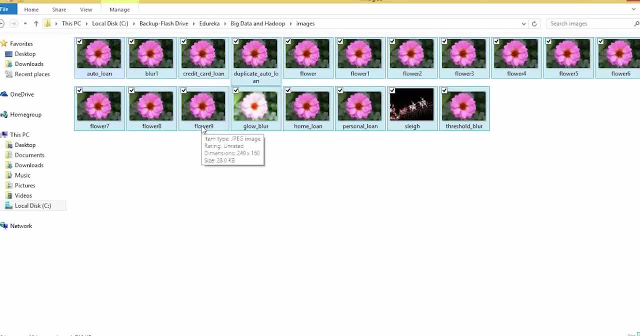 One is here And nine times of this certain. So in other words, if I the business, the problem statement for this exercise is to get rid of the duplicates. It's a pretty scientific problem. So let's say: you know we are talking about. you know, I need to get nine images. 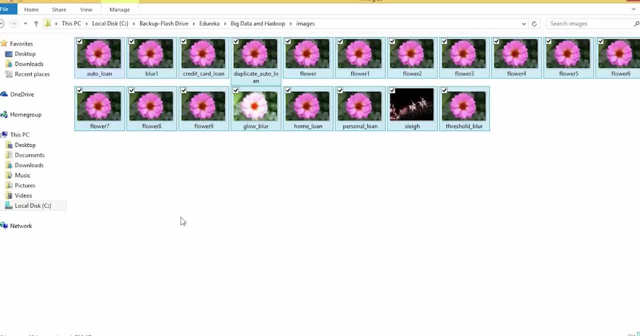 Right, Let's say you are given 100 million images, Fine, And someone tells you that you know you are working for a Cryptography project which has got like fingerprint scanning and all that stuff. Right, It's a very high, sensitive project. 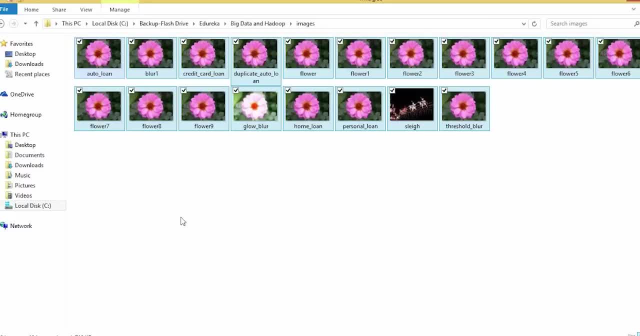 They want the data to be treated with utmost confidence. Now they are looking at you know various fingerprints they've given you. Now they are telling you to get rid of some of the fingerprints that have come as duplicates, OK, And they say the number of duplicates could be maybe 100 or 200. 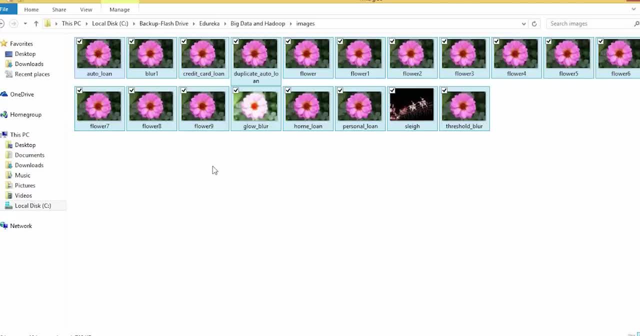 How do you do this? Any vague idea? you guys have Any vague idea? Anybody has this idea. friends, Image processing tool- OK, matching pictures- Upendra says that. Any any other guesses? friends, OK, so well, I'm not. what I am trying to say is: it's a very scientific problem. 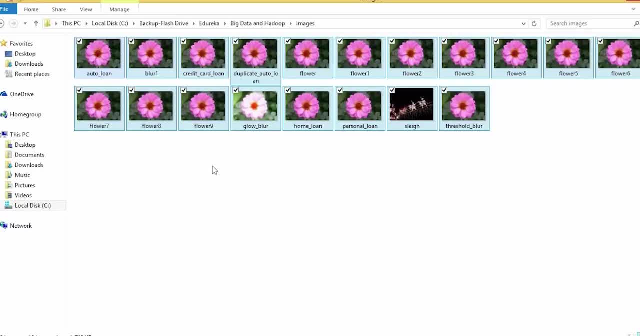 How Hadoop uses you know. I just want to showcase that part. Beautiful Anil Kumar. He says MD5 value, Right, So that's size of the file, may not? you know said it. The point is, size of the file is a very misleading attribute. 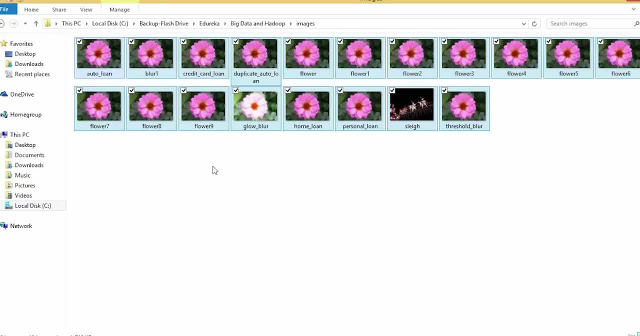 Right, It could still. the size may be the same, but the file type- So many things can be- you know different, Right? So MD5 is one of the you know algorithm, Right? So that gives you like a hashing value. 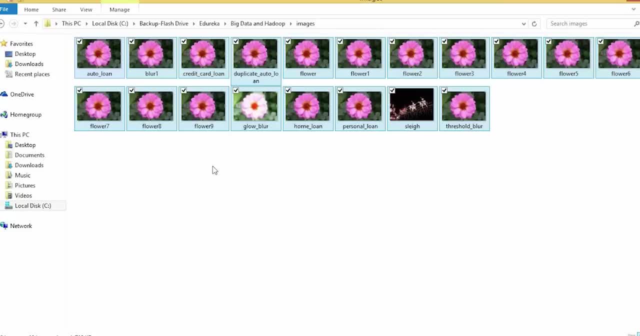 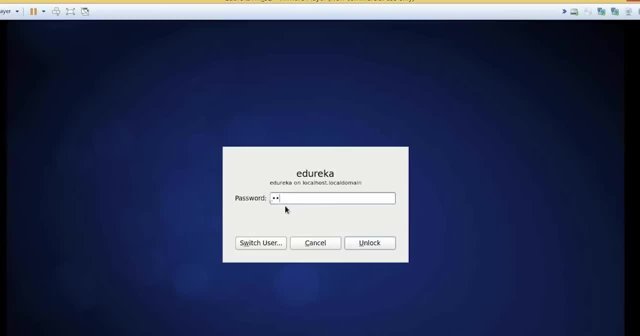 Using that, you can be able to find the duplicates Right. So that is something you know. I just want to showcase that quickly. I'll not be, you know, taking much time here, So what I want to show is: 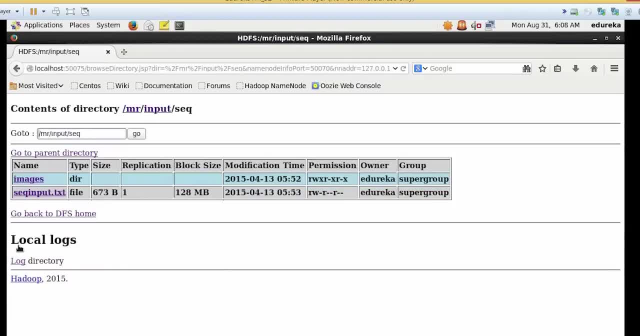 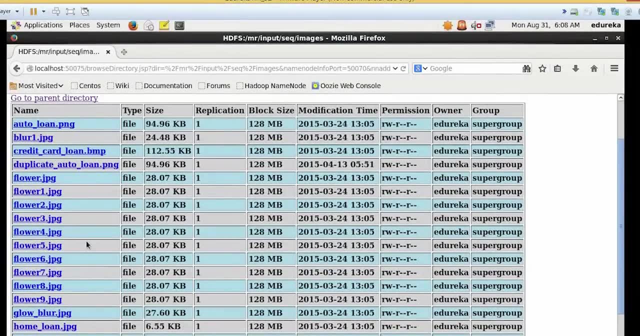 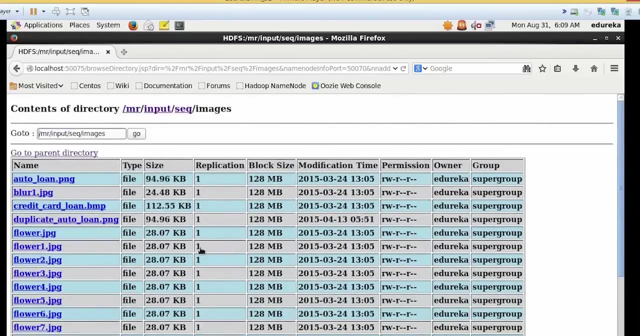 Map, reduce input. you know I have already put these files, these images, into this folder. right now I want to get rid of this. I don't want to physically remove these files. I would rather know. instead of getting 19 entries here, my output should have only 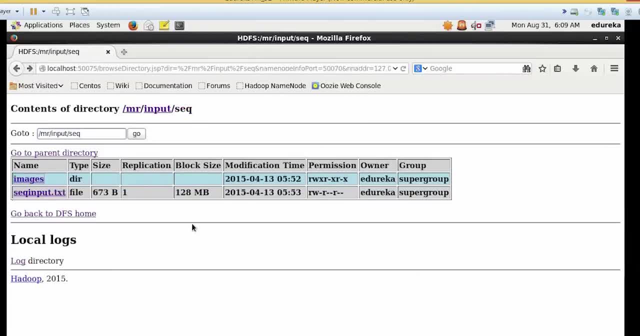 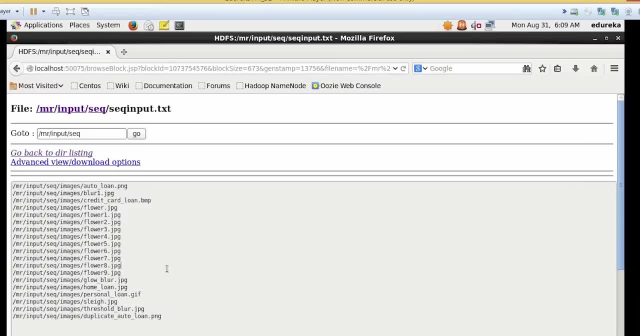 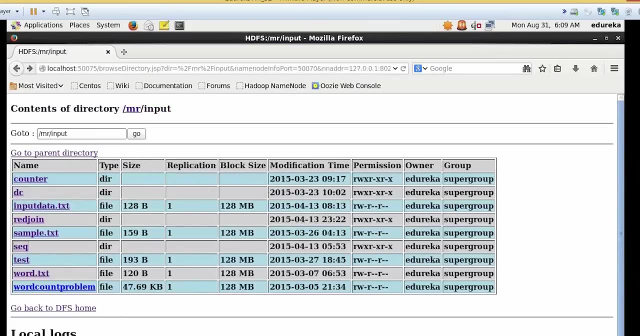 Nine entries right, Ignoring those 10 duplicates overall. So this is my. it has the URI as well where the flowers are stored. So my, what I want to convey here is, like you know I will, I have my eclipse. Just give me a minute. 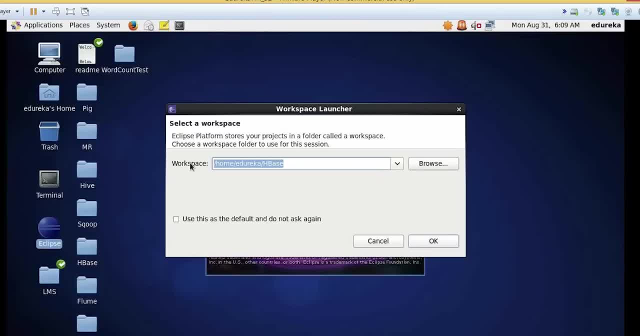 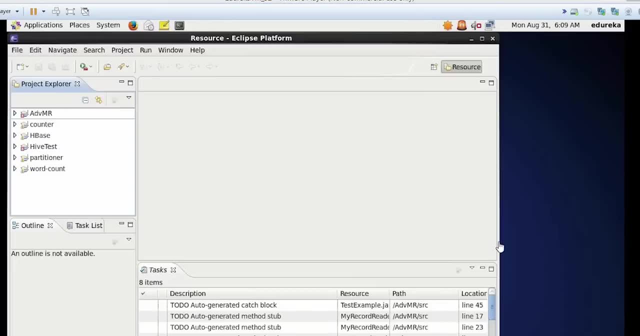 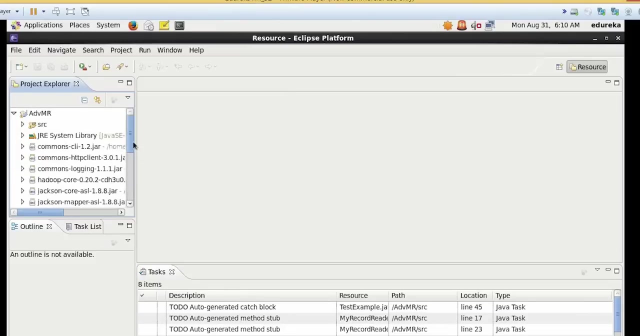 I can show this quickly, I'll be great. OK, Just a minute. OK, I got something here. So, friends, Differentiate the duplicates. OK, I'm coming there. Differentiate So what I want to convey here. friends, differentiating the duplicates is you. 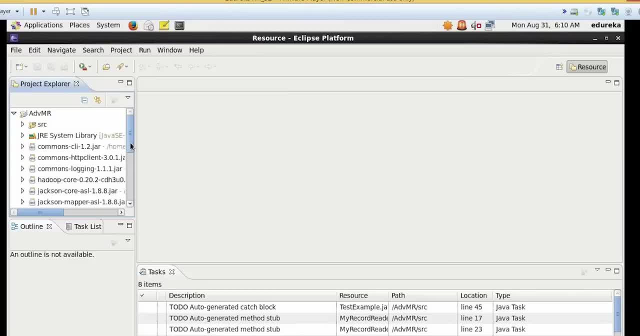 know the empty file. I'm going to put it in a compressed format, right? First, I'm going to put that as a sequence file, which is nothing but a binary file. Then how do I do that? You know I'm using a framework to do this, right. 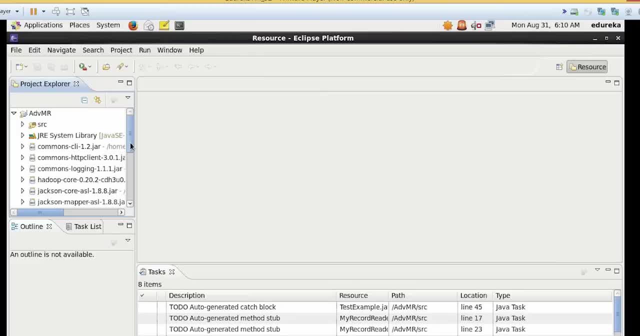 Using a MapReduce program, which is nothing, but you know it's part of the Hadoop, So I'm using MapReduce framework here. So what I want to do here is see, I have this first thing, I want to keep all these files. read the files completely. 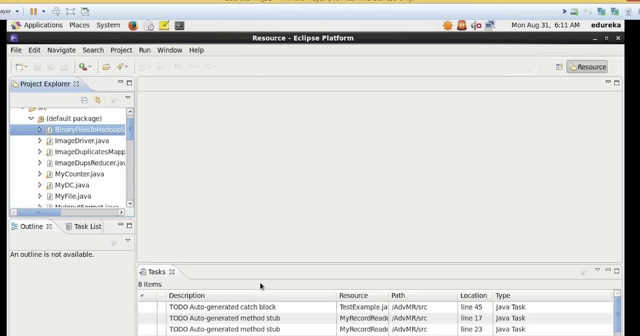 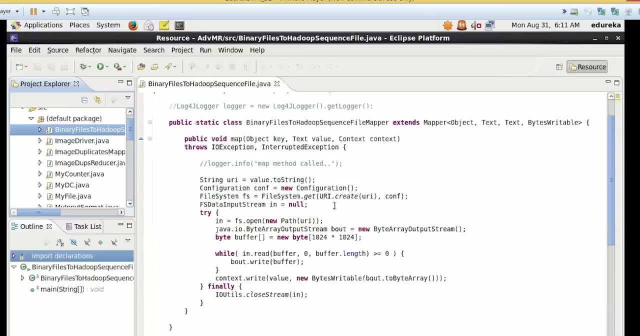 There are two steps process to this, friends. OK, two steps process. Just give me a minute, I'll explain you this, Then you can ask this question. Fine, There are two steps process. two step process. One is: I want to convert everything into binary. 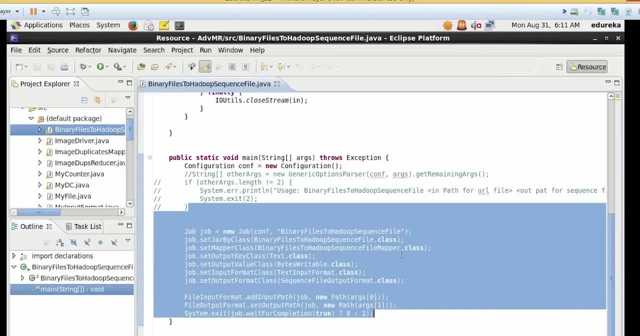 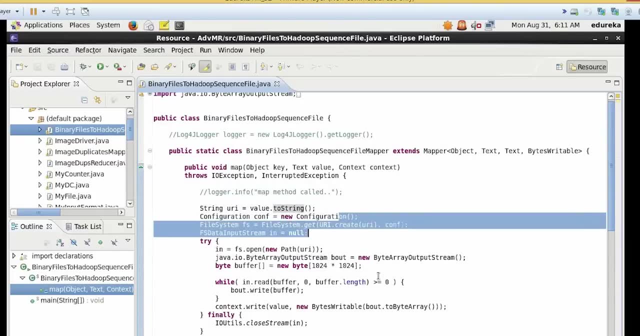 So let's not. I'm not going to go too much deeper into the source code, But what I want to convey at a high level is: I want to read the file one by one, based on the URI. Right, I showed you the input. 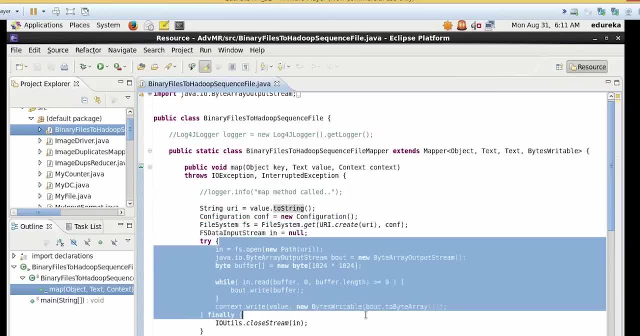 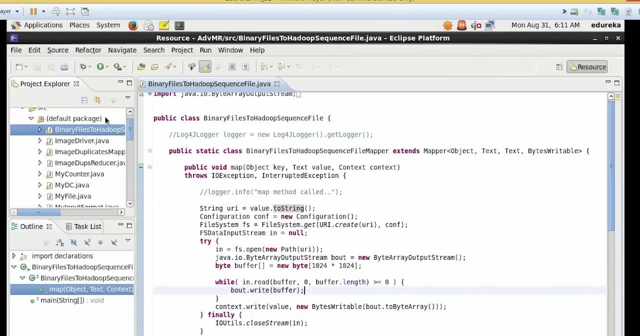 Right. Then it's going to read: create a byte stream out of that. Fine, You got it. So that is the first step I want to do, Then the second step. OK, that is the first step. Second step is this: is my reading that file. 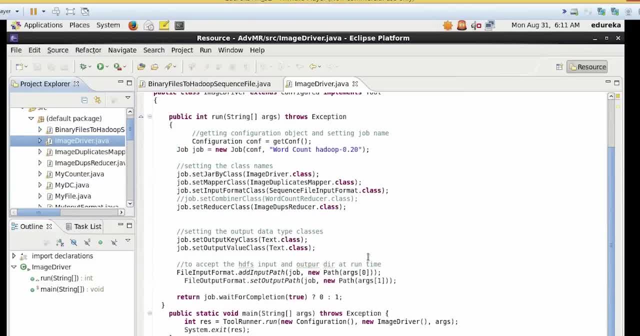 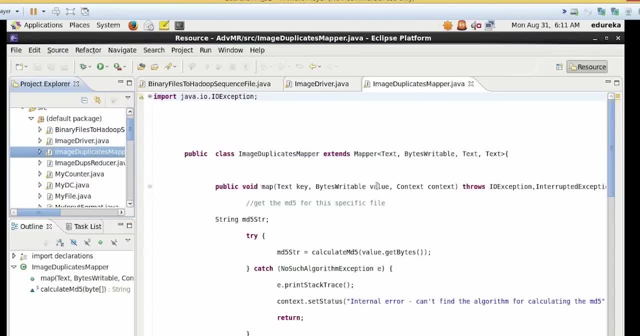 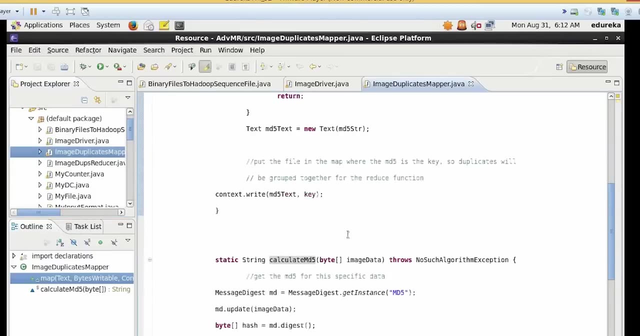 Fine, Reading that file Right, I want to process image by image. I want to create an MD file. You know, here I want to create calculate the MD file, message, digest file, Fine, So that is going to generate a hash value which I want to convert it into a hexadecimal. 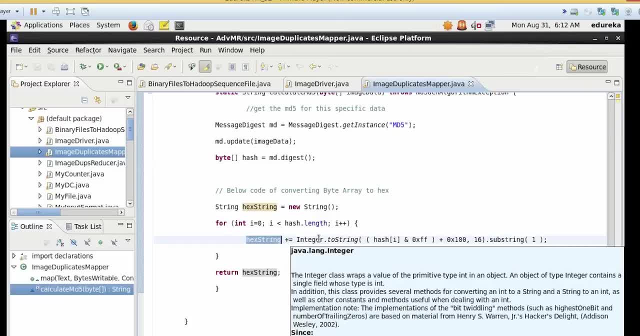 Fine. So if the hexadecimal matches, OK, I want to just drop that. So those are all duplicates. So again, there is something called MapReduce in Hadoop. MapReduce is nothing, but you know, map is processing, reduces nothing but aggregating the results of the processing. 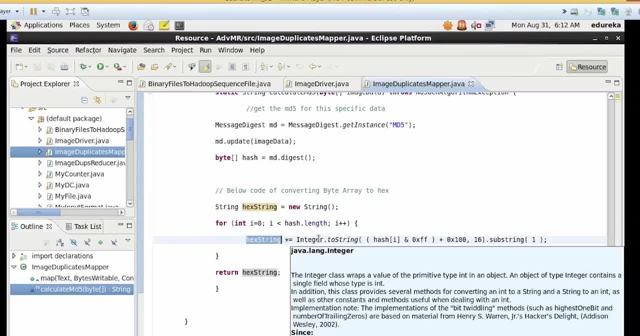 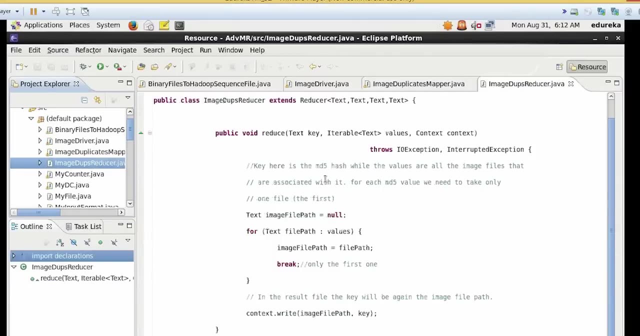 OK, so if I have 20 documents coming in right, with each one of them, you know having different, different results when I want to combine it and aggregate right, that is what is your reduced process? Fine, So now When I do this, reduce right first, you know I want to get in and you know. 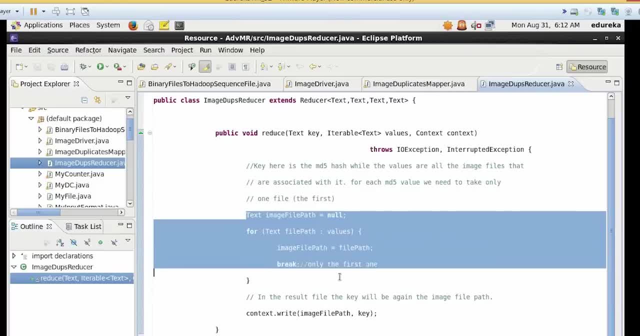 just do this. I process only the, you know, the first time, because if I have 20 different identical values, I want to get in the first time and do a break so that you know I don't get to process the duplicate once. 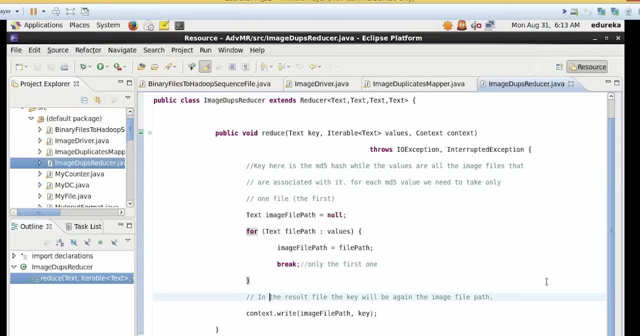 So I'm using the Hadoop framework very effectively, The Hadoop MapReduce framework. Any questions, friends, in this? How to run the same program without Java like big Sure. I mean we need to write logic for this. funny, it's going to be a lot more. 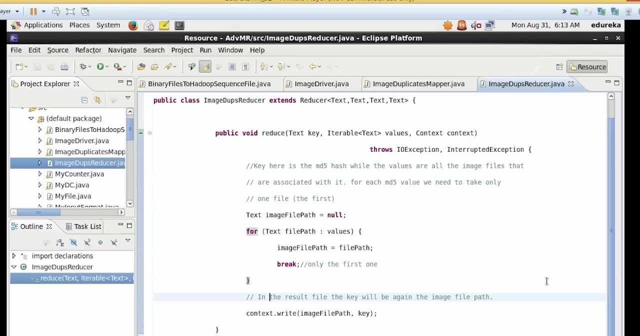 you know simpler in big It's going to be, you know, fewer lines and because it internally uses MapReduce, big internally uses MapReduce, So It's more like it will do the. you know you don't worry about how it is done. 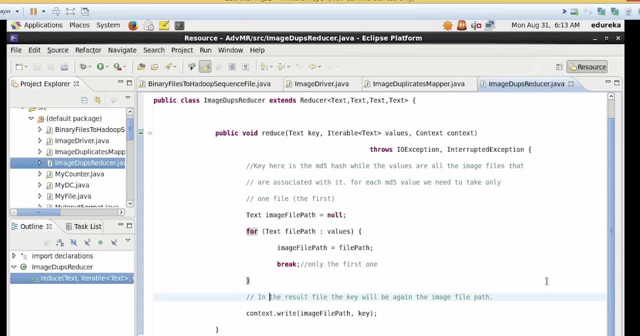 internally and all that. you just tell what needs to be done. Big will take care of that Right. So that is something you know big is extremely useful for. But you know, if there are completely unstructured, and you know. 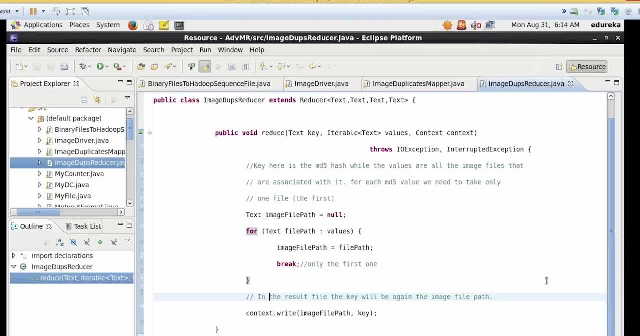 audio video files and all that. I would suggest to use MapReduce, at least at the first level, because there are more supported libraries and you know tools And tools in Java compared to other areas Right, So you can exploit that. Then you're going to begin for the second level of analysis. 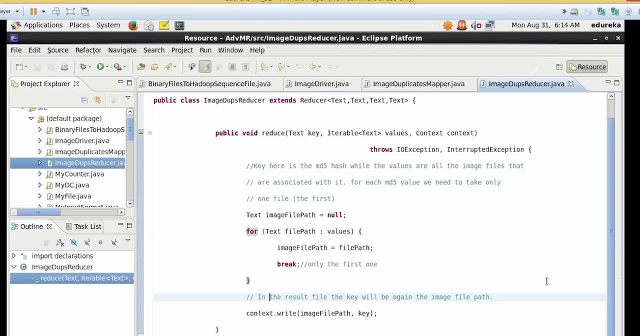 You can do that. No, no, no, it will not be time. Indra is asking: is something like SQL PL? No, Indra Big is more like you know. yeah, it's closer to SQL. I would say closer to SQL. 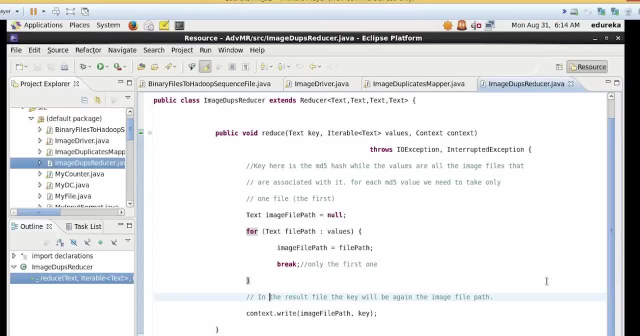 If the memory in which duplicate is present is very large. No, no, it will not be time consuming, Rajat. It will not at all be. Why we want to do this into binary format is to we want to process the binary. 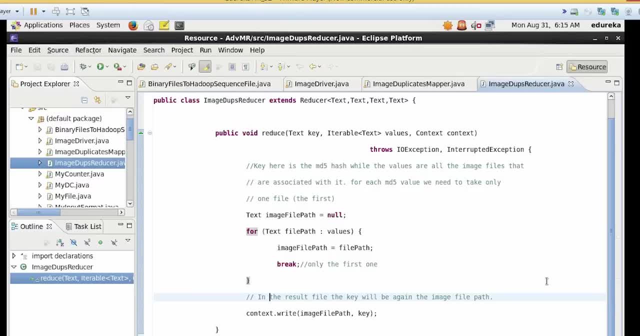 Now we see I told you about. you know the step. Initially you can process things in chunks, Right, If 100 million map process you know runs, because these are all distinct images, Right? Do you want to run 100 million processes in different computers? 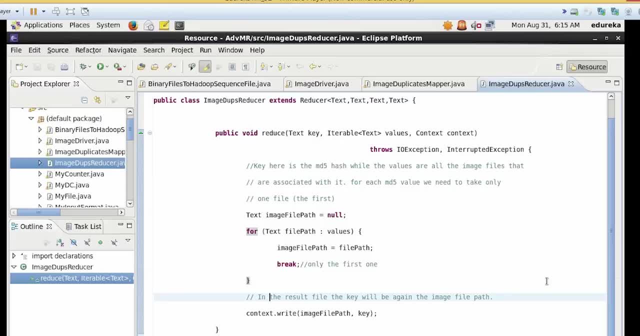 Is that very efficient, Yes or no? Because these images are very tiny, right? Jif files, JPEG few are bitmap. They are all tiny files, right? Is it good to process that many files in you know a separate process threads. 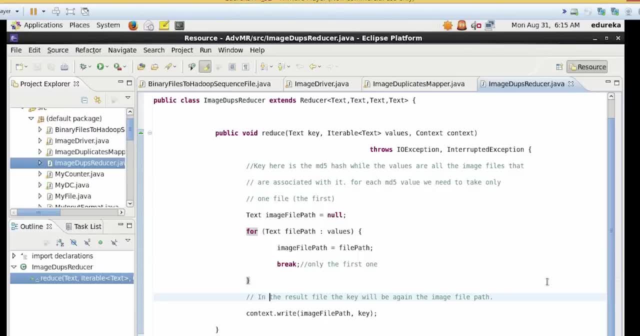 Is it good to process 100 million files? No, right, You all know this. It's a no because it's going to be overheads in collating them and all that, Right? So you want to create Because it's a very small file, right? 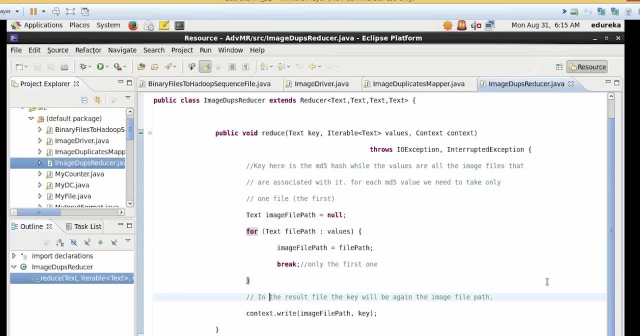 You may want to process it as sequence files, which is nothing, But you know, I want, I want to compress them and, you know, keep them tidy so that my processing, in fact processing speed, improves overall. Right, You got it. 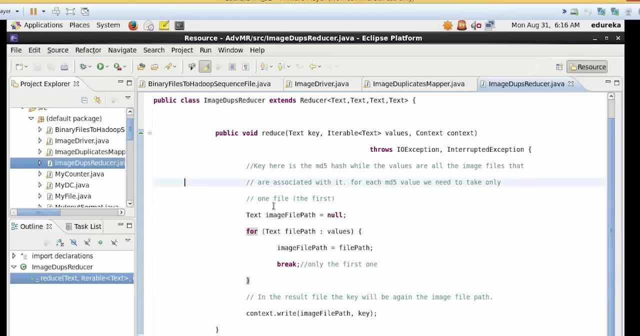 So let, first thing, Do you all understand the overall structure of this program, What I mentioned, folks. First thing, I want to convert that into a binary sequence file. Second thing, I want to read the file, Get the MDFI value of each file, then go to this: you know the aggregation part. 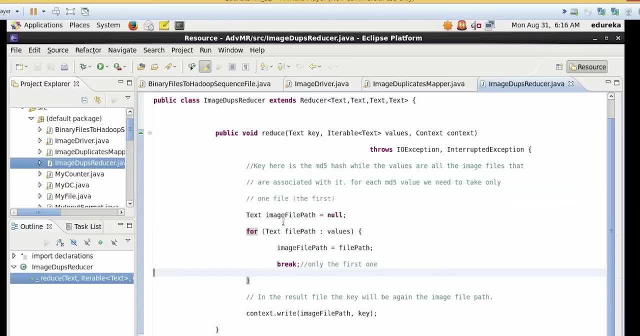 And you know, because I'm not physically removing the file, I'm only putting the path first time. I do this for the same thing, you know. for the rest of them, I jump out of the loop by doing a break. Are you all getting this logic overall? 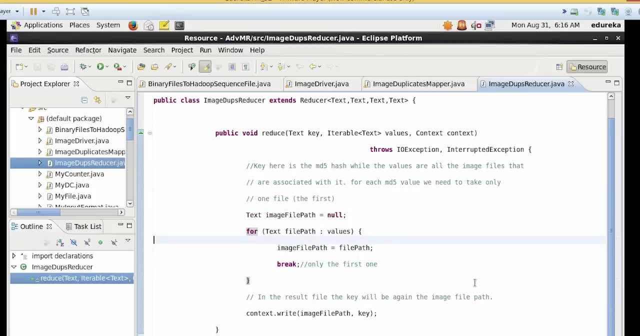 Do you understand what I'm saying so far? OK, why we do? Yeah, binary, Why we do this is to simplify the. you know you need to process it right. You can't do. you know I don't want to treat them, as you know, separate. 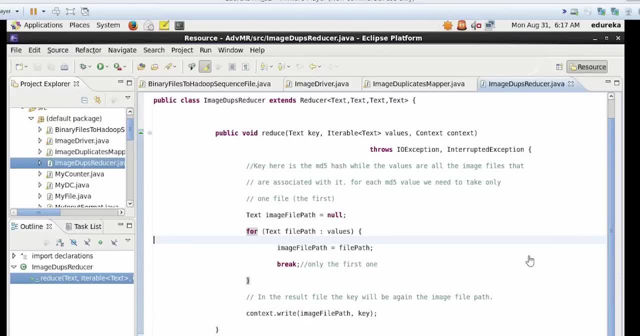 files and process, because that's going to be very, very time consuming. So I want to compress them. So that's why I'm treating converting them to binary Fine. Secondly, when you are, when you want to process these images, Right, I need to have it in some format. 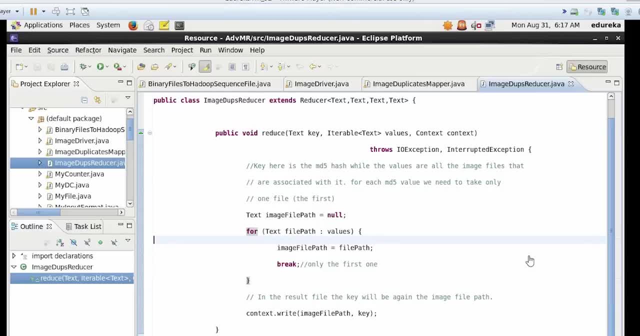 So binary format is the, you know, compressed and shortest format I can have. Mohammed, are you clear with this? That's why we are doing this. Then only we can build some hash out of the file. First thing is we need to 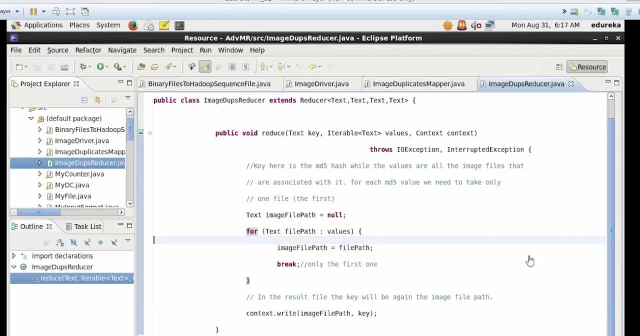 Read the file itself, right, then convert that into binary and all that. Yeah, Is that clear? Yeah, OK, friends. but overall, I want to ask you: are you understanding the what we are trying to do with the overall files, right? 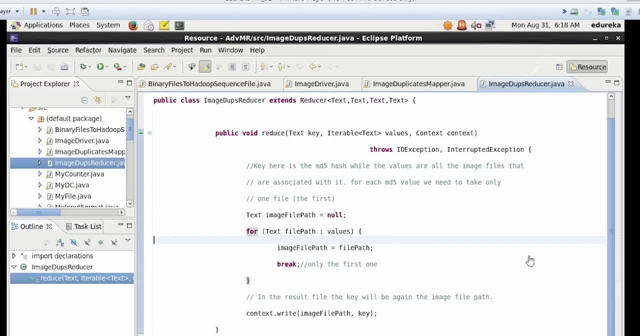 The overall structure. you're understanding what we are trying to do. Is that correct? OK, brilliant, Thanks, Fred. So what I will do, I'll execute this. I'm going to convert this into a job, very simple job. 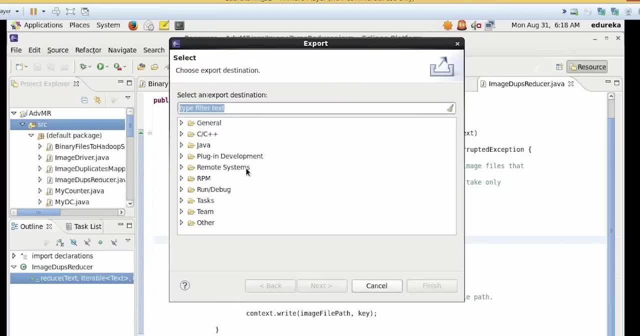 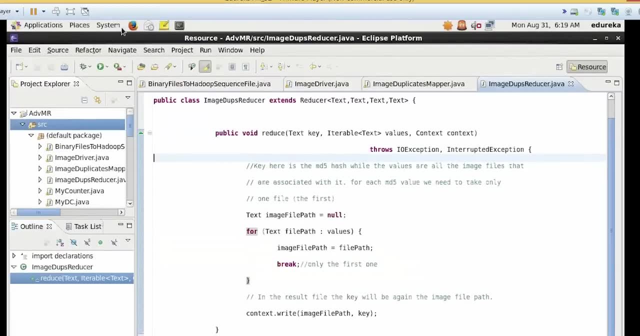 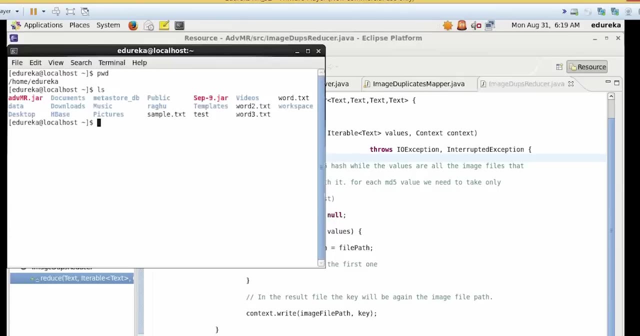 Give me a minute. OK, I've done something. Let me go and check it out. Just give me a minute. Have the jar file right there. so I'm going to do Jar, OK, The first thing I want to. 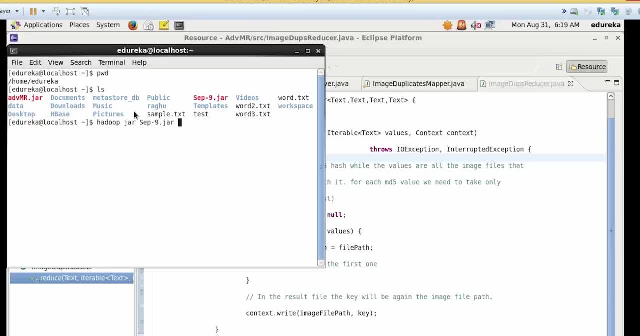 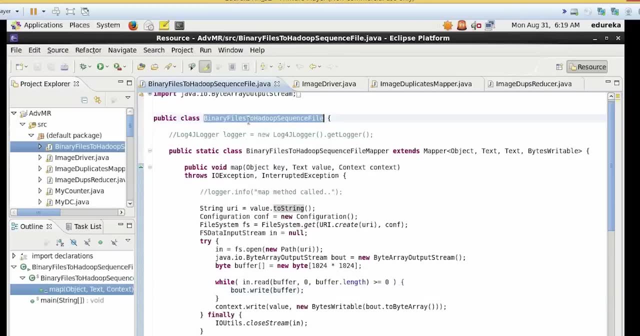 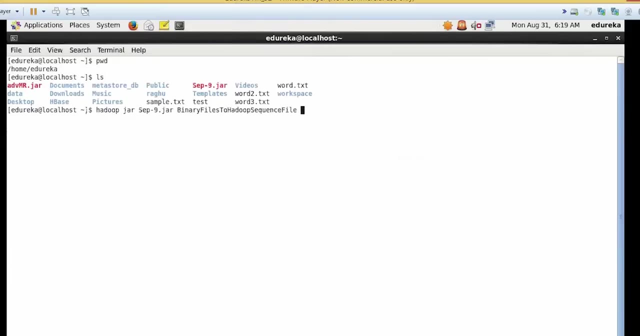 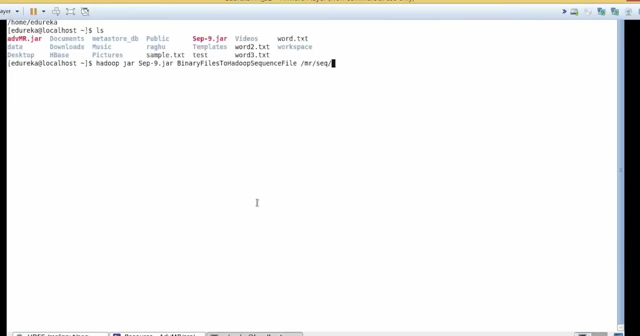 And The first thing I want to, And the minute my input is MR, MR Sequence, I think the input file, My input sequence, second text, And I want to write the output to September 9th: Yeah, Emma. 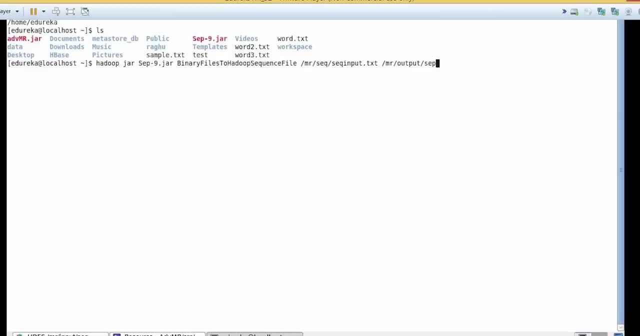 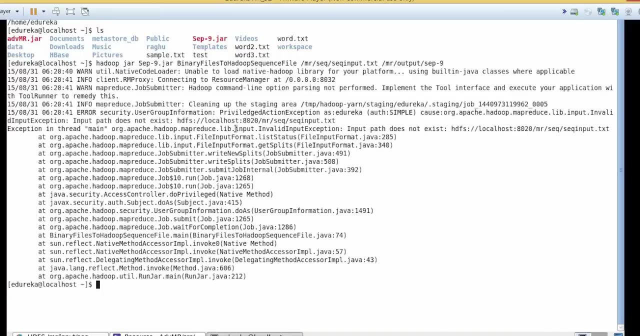 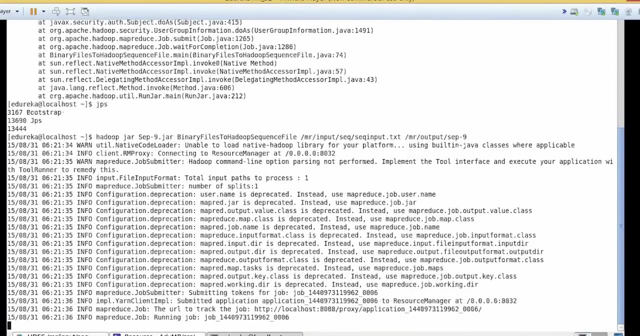 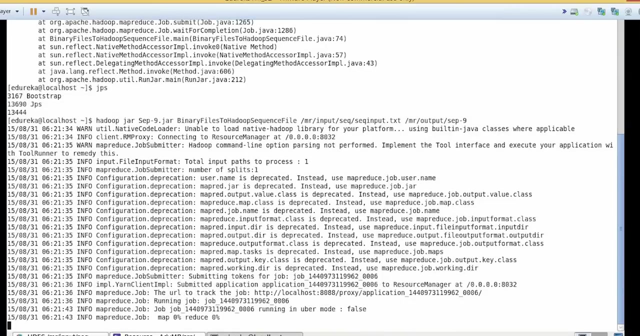 Just September, September. OK, that is a file, OK, um OK, Um yeah, i think i gave this mr all mr input, or there is a folder in. okay, give me a minute, thanks, thanks tomorrow. thanks for suggesting that here. so my is asking. 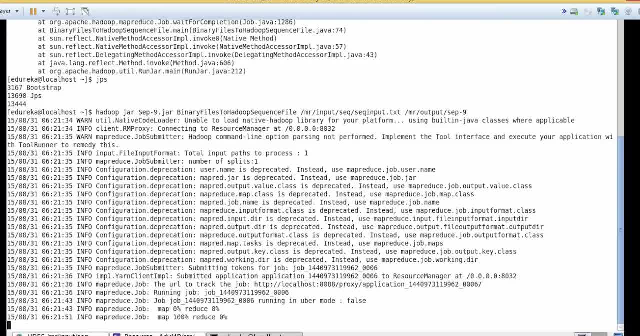 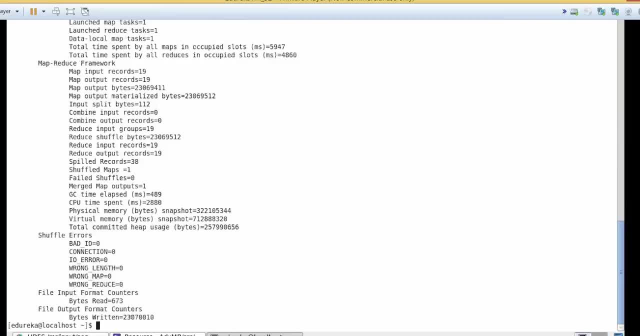 distributing file in multiple slaves. and how do we compare each images, duplicate of no, actually read more. the point is: see the it's going to be, yeah, it's going to be distributed, I agree with you. but you know when the binary file, whatever we are contributing, right, if it is stored as stolen, as distributed, right, the point is we are 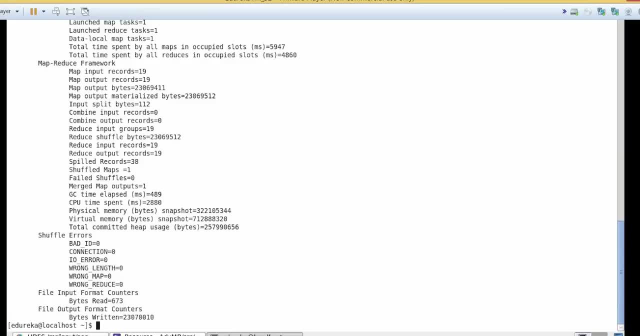 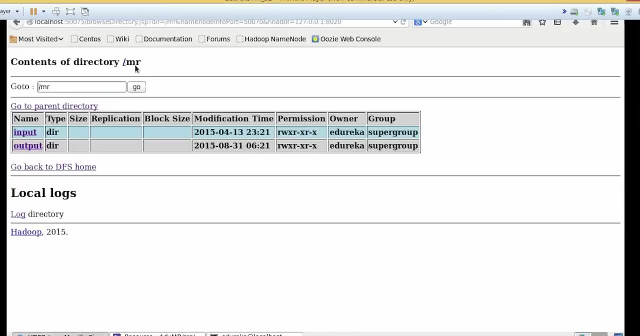 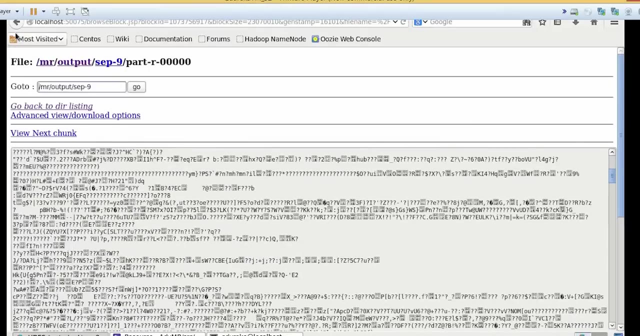 going to keep this right. we are this the file. ok, let me show you. instead of talking about this, right, let me show you this part, this part, right, this is my output, this file, this is my binary file. ok, if this file can be distributed across the cluster. 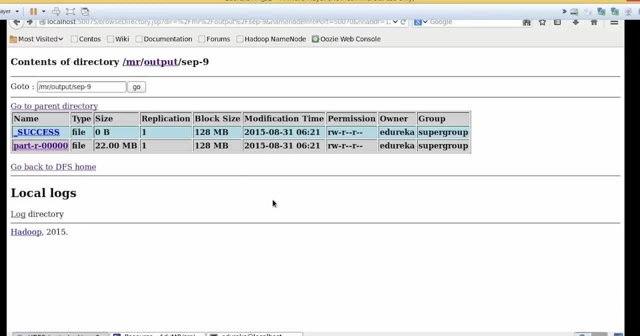 that's possible. this file itself, part 00, right, which is our, which is our cluster, ok, this, this file can be distributed if the threshold size of this file, if the file is about, let's say, 300 megabytes, it can be distributed across the cluster. so, 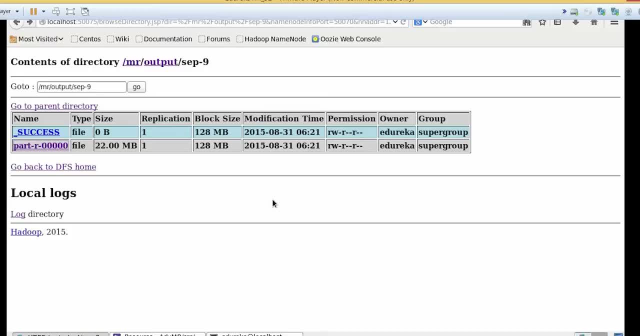 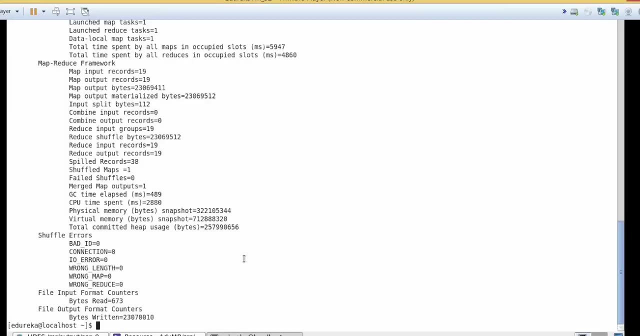 overall, the, the framework, hadoop framework, will take care when it processes, it goes in, you know it can still process it as individual blocks. that's possible. so I will tell you how it can be. because when we are doing this right- see my second part of my second part of the processing right, this is my first part, right I have. 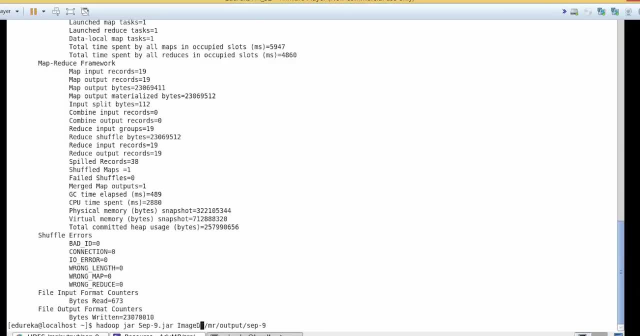 converted that into binary. this is my second part. okay, what will be the input for my second part? the output of the previous thing, which is nothing but this. right now I am going to- let's say I want to do- output. September 9th, say final, let. 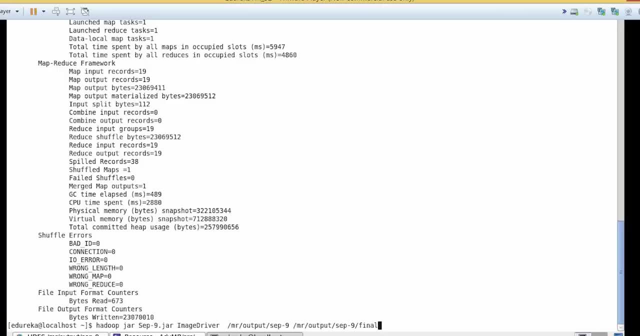 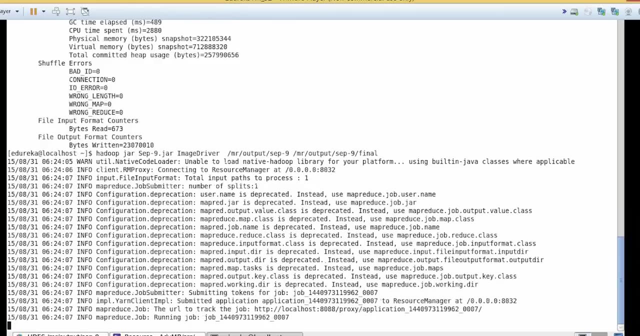 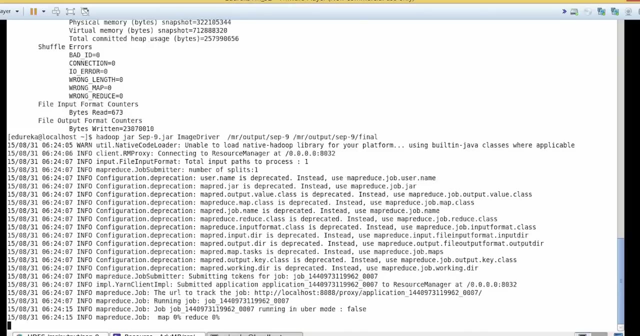 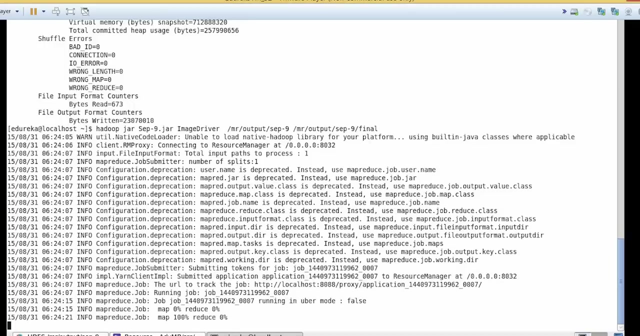 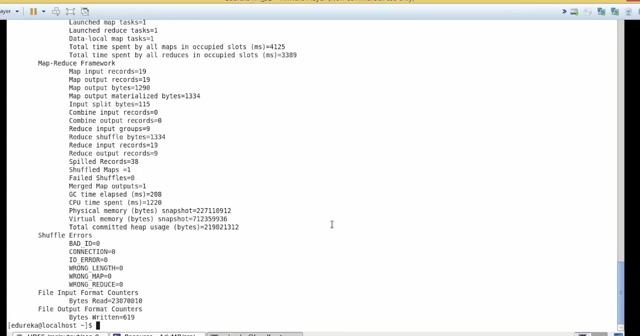 me say that: fine, so let's try this. so read my point is: if that file, the output file, which is what you saw here, if that file is large enough, right, it will get distributed across the cluster. okay, and the hadoop framework, by default, it's going to follow the thumb rule of data. 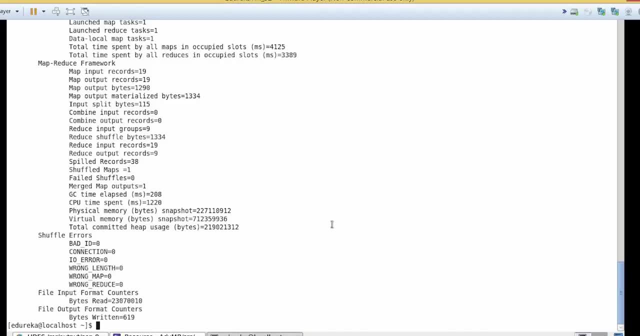 local data, locality, right, which is nothing, but it is going to take the program, which is this jar file, and all these things, configuration files. these are all the programs. it is going to take them into the respective slave missions where it is going to run the you know processing. so now it has done this right. 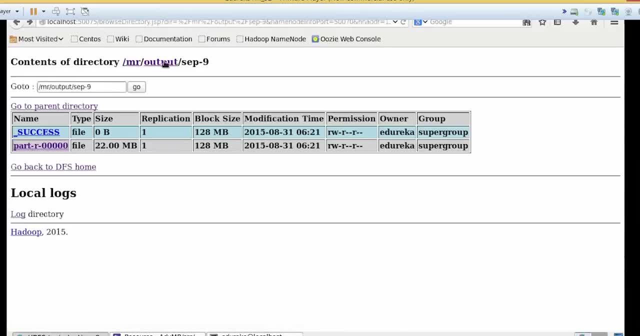 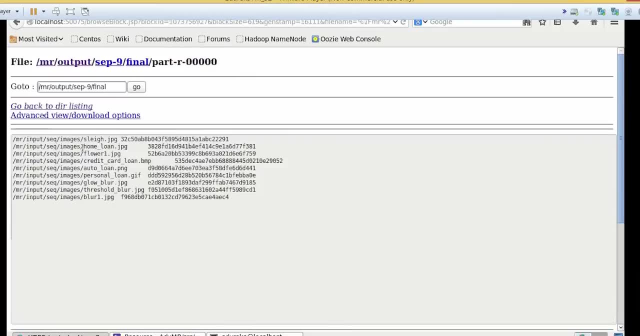 okay now if I want to go back to the output and be able to there, if I take this, left our assistant type, See the, the hash value or the MD Phi algorithm. Fine, so those image. when you are comparing two images, you cannot go by the size. 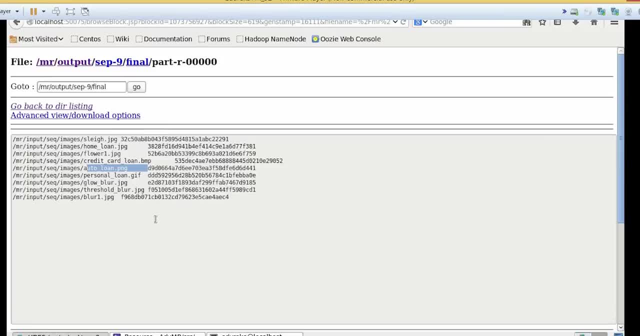 You cannot go be the types and all that, but the hash value, the binary format, right. once you Create the hash value using the binary, It cannot be different. I mean it will be the same for two identical images. That's my point. So we are gotten rid of the duplicates. 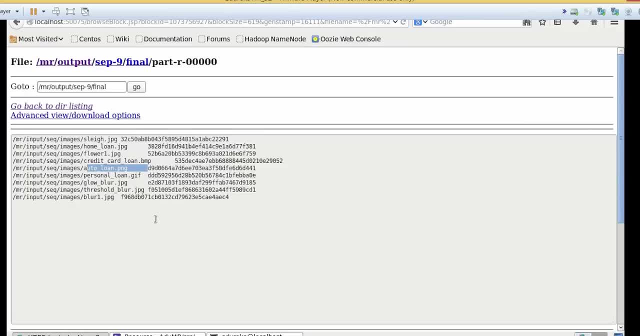 Is that clear, friends, overall? See, Hadoop can play a very major role in exercises like this. You can probably. you know you can also how to avoid noise in a bar conversation. That's a very famous program to right. we can use Machine algorithm, machine learning algorithm, for that right. So the again, Hadoop can play a major role there. 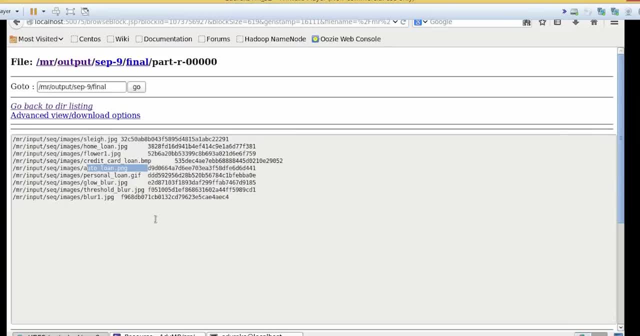 Is that clear to all of you? Okay, so, friends, we have come to the end of the session and Hope you found it useful. If the images in the crop of the images, I Don't understand this question. Roger, images is the crop. I'll try to answer Rajesh question then. 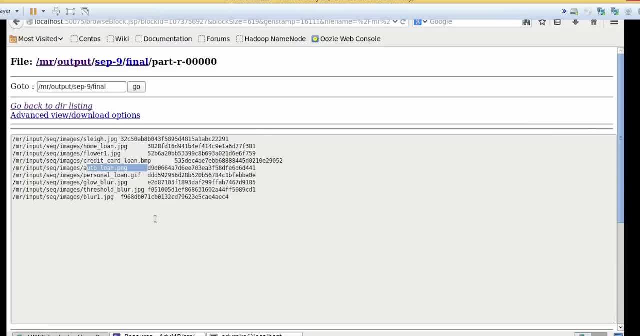 I'll wind it up. so, friends again, as I requested, hope you enjoyed this webinar overall, so hope you found it useful. so I really want you, to you know, provide the feedback, as you know, as I requested earlier. yeah, sure, said it. so, Rajat, maybe, if you can, sure, sure, Indra, maybe Indra can you know, help you to you know, solve. 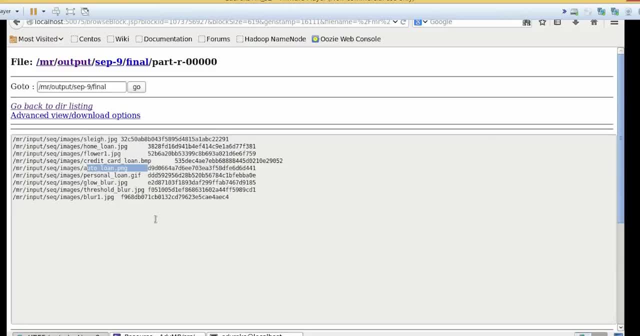 the. I mean provide this information. new images, crop of previous images. will it be? yeah, yeah, see any image, identical image. I just it's going to have the same value. that's my point. yeah, you image a world image, right, so it's going to be. you can, you can find out this value and it will be the same. that's. that's very much.